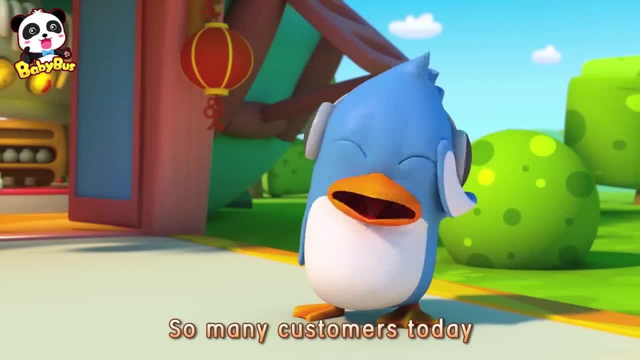 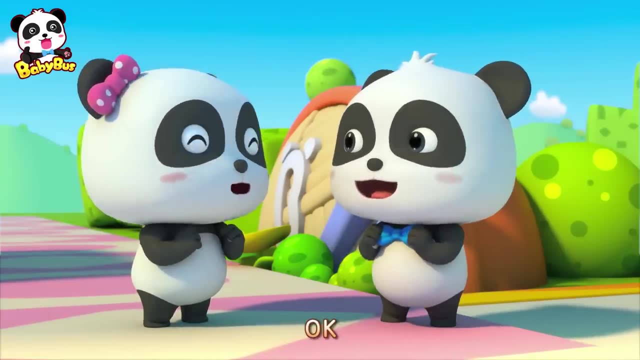 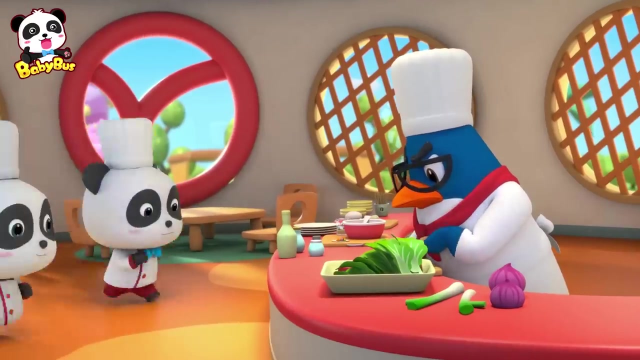 Thank you. We've been busy because of so many customers today, so my father asked me to help him. Miu Miu, come on, Let's help out. Okay. Baby Mugs change into little cups. Kiki, Miu Miu, are you ready? Yes, 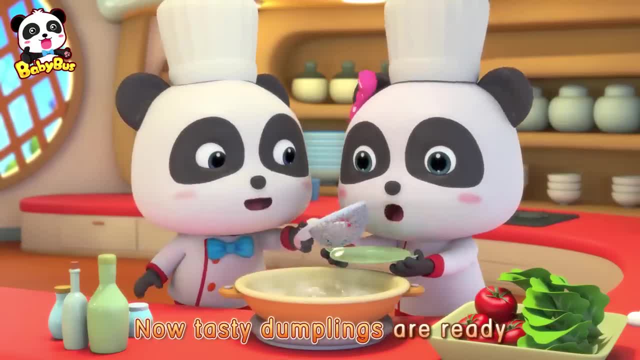 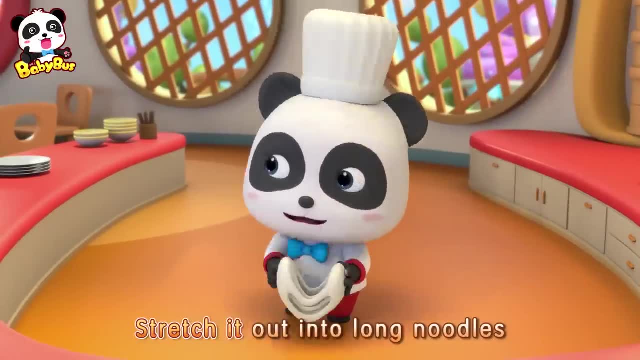 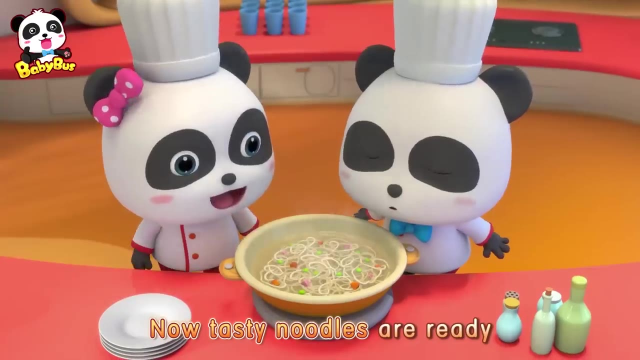 5,, 6,, 7,, 8,, 9,. no tasty dumplings are ready. Put some flour, pour some water, mix and make the dough. Stretch it out. stretch it out into long noodles 1,, 2,, 3,, 4,, 5,, 6,, 7,, 8,, 9,. no tasty noodles are ready. 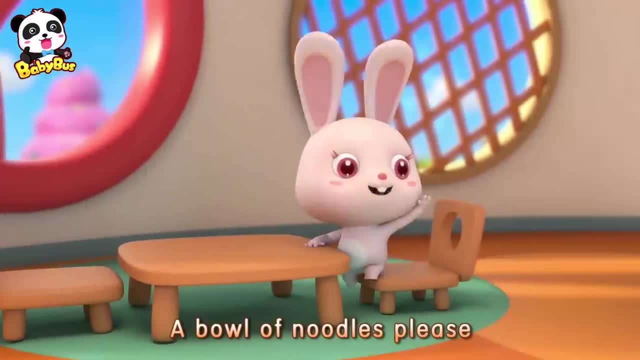 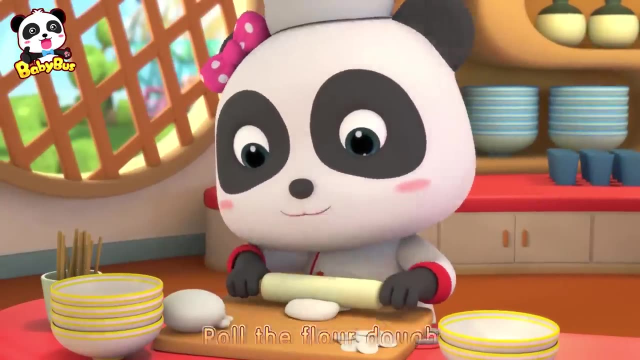 It's so delicious. Give me one more plate, A bowl of noodles, please. Okay, Chop some veggies. make the filling, roll, the flour dough, Let's make. let's make. make the dumplings 1,, 2,, 3,, 4,, 5,, 6,, 7,, 8, 9, 9,, 10,, 11,, 12,, 13,, 14,, 15,, 16,, 17,, 18,, 19,, 20!. 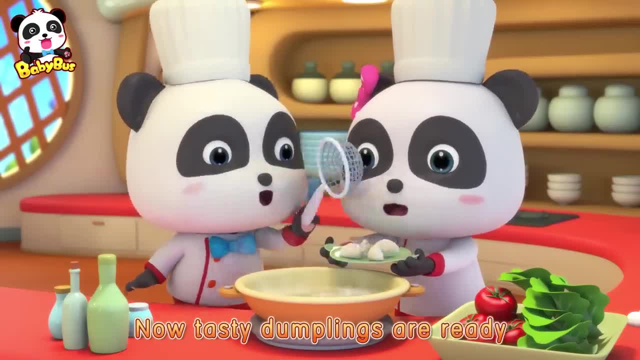 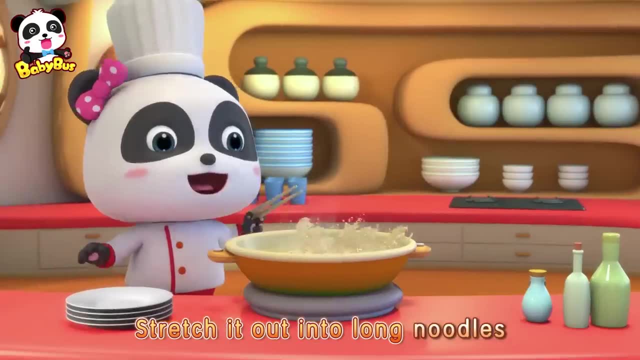 Now tasty dumplings are ready. Put some flour, pour some water, mix and make the dough. Stretch it out. stretch it out into long noodles: 1,, 2,, 3,, 4,, 5,, 6,, 7,, 8,, 9,, 9,, 10,, 11,, 12,, 13,, 18,, 19,, 20!. 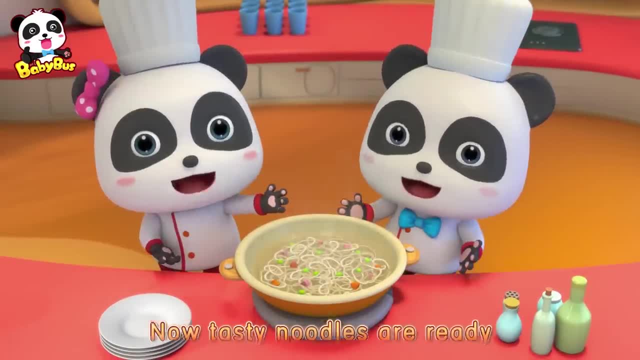 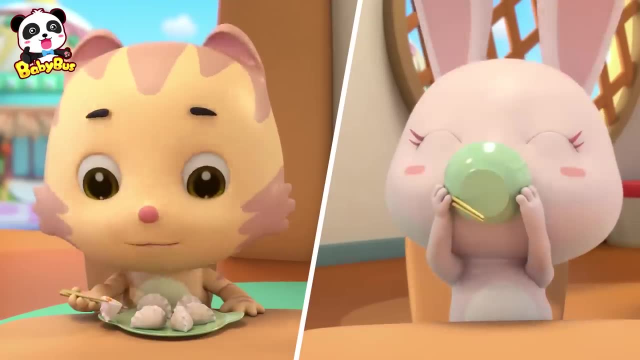 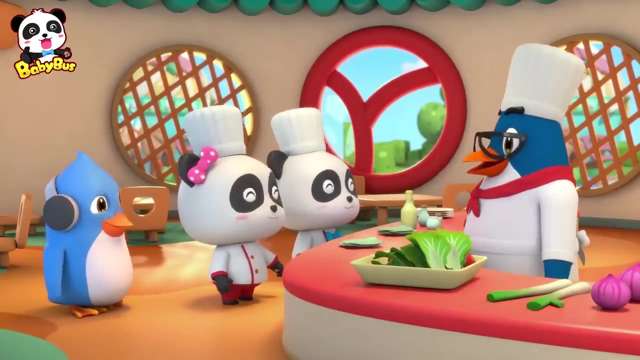 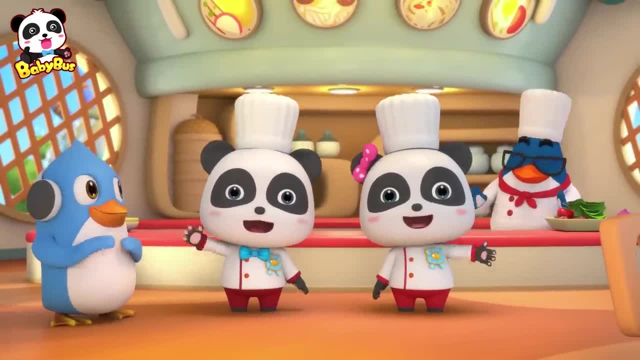 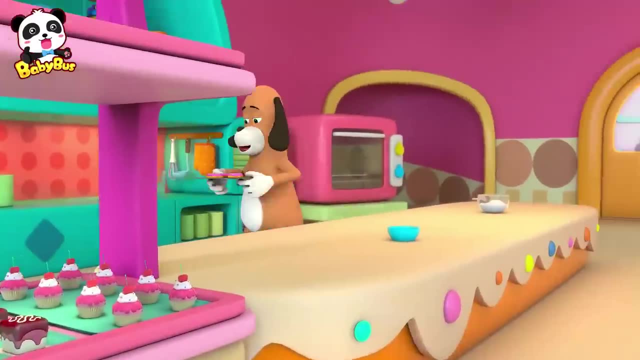 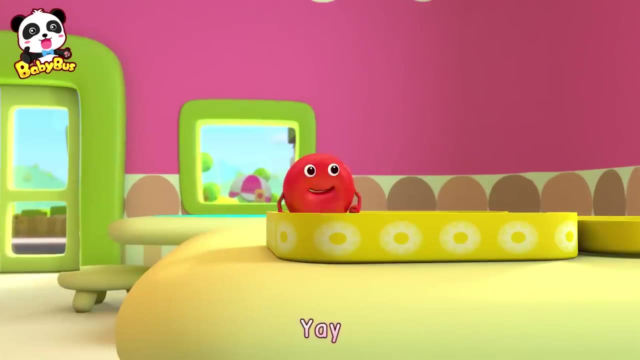 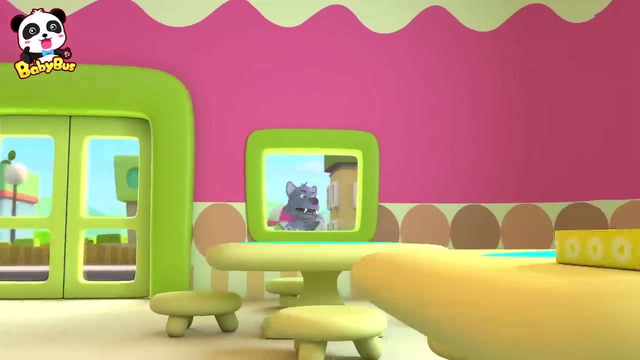 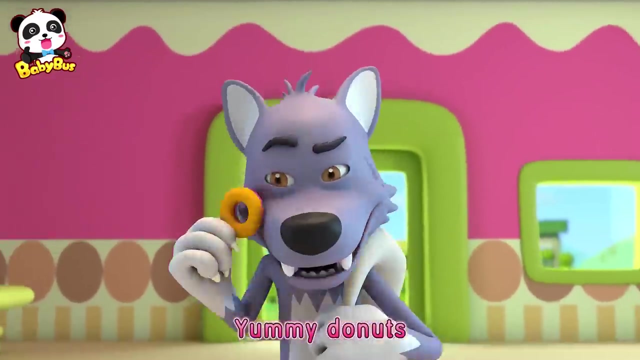 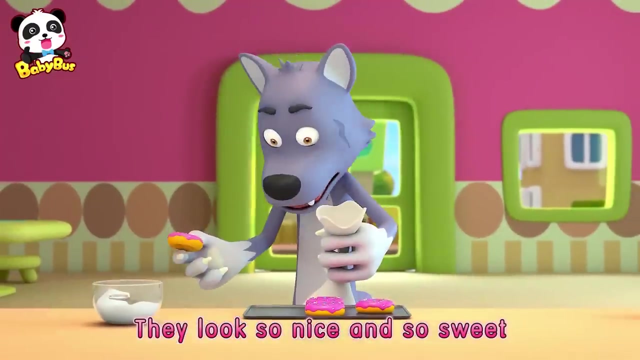 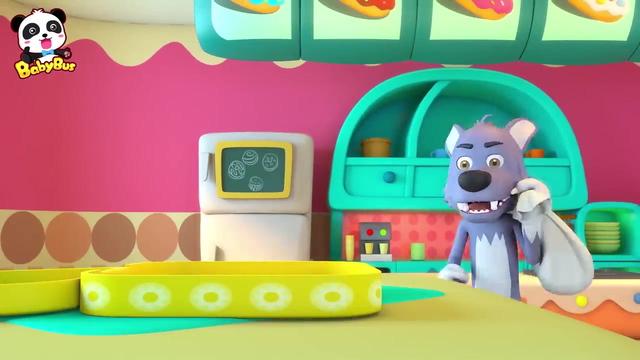 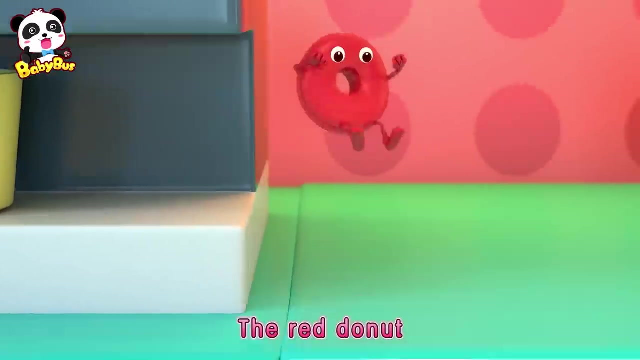 ல. All right, everyone. Yummy donuts. I want to take them all. They look so nice And so sweet. I want to eat them all. Run everyone. No donuts here. The red donut Running away from Wolf. 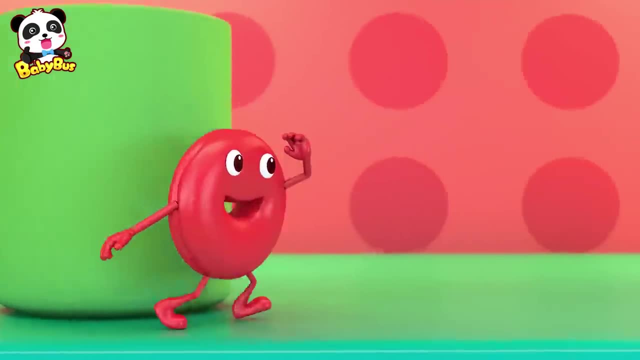 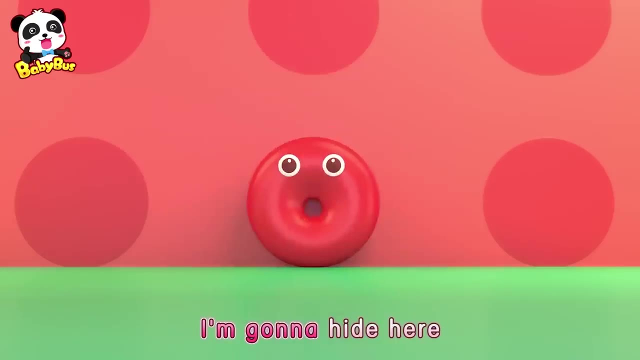 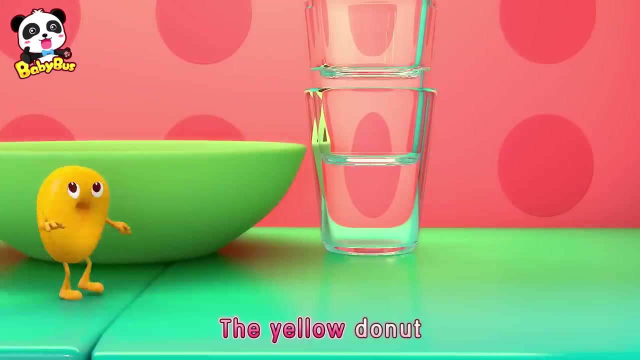 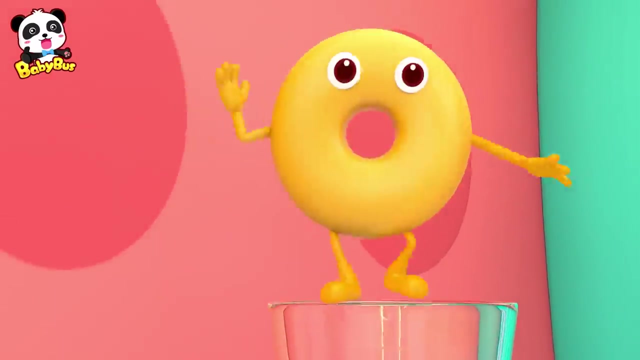 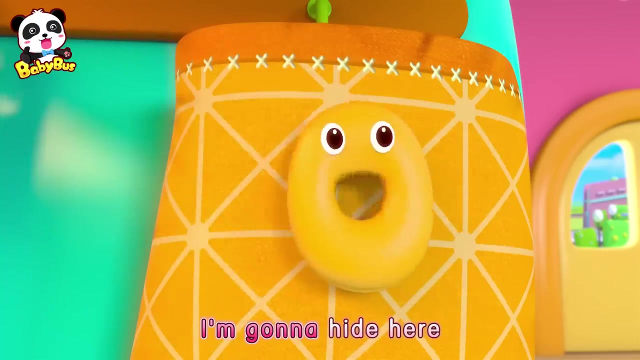 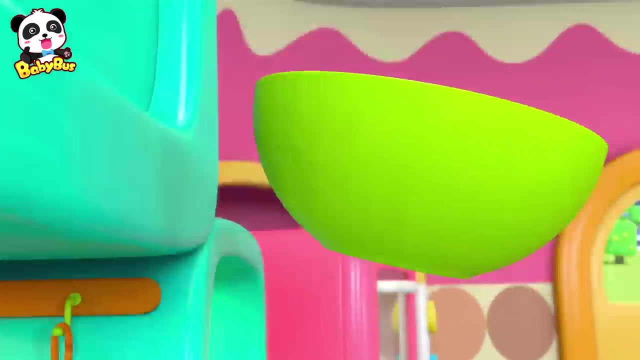 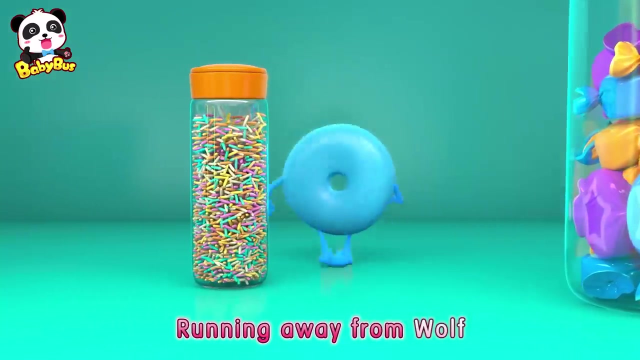 Look at this place: It's all red. I'm gonna hide here. Where are the donuts? The yellow donut Running away from Wolf. Look at this place, It's all yellow. I'm gonna hide here. The blue donut Running away from Wolf. 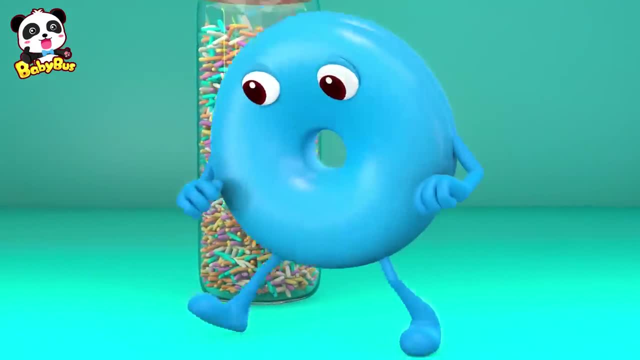 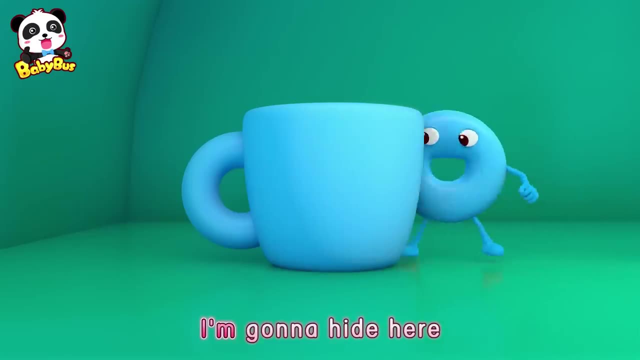 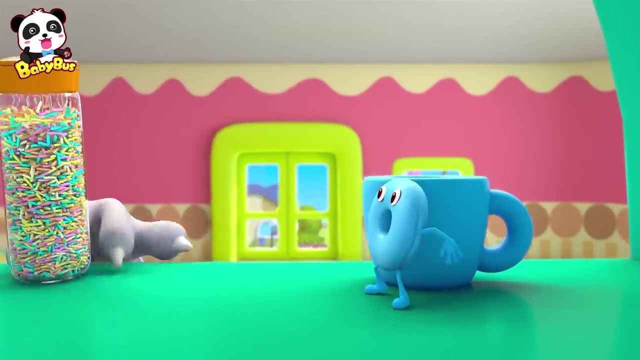 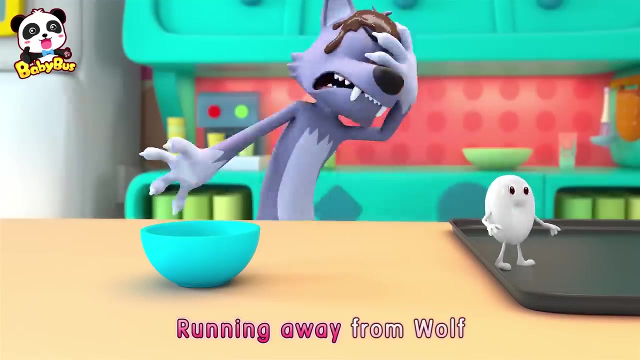 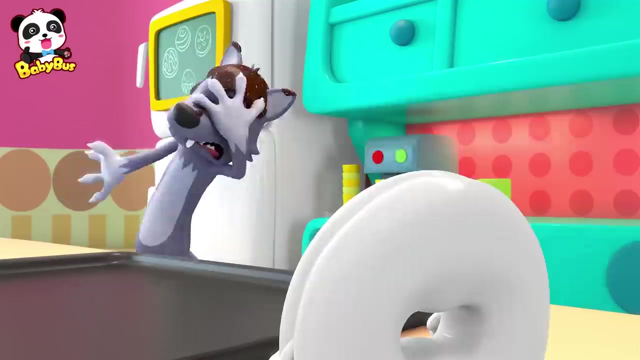 Look at this place, It's all blue. I'm gonna hide here. I'm gonna hide here Here. Ah, Ow My head. The white donut Running away from Wolf Over there. I'm gonna hide Over there. Oddy is running away. 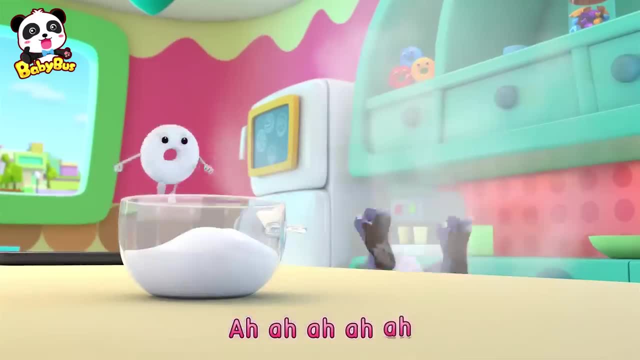 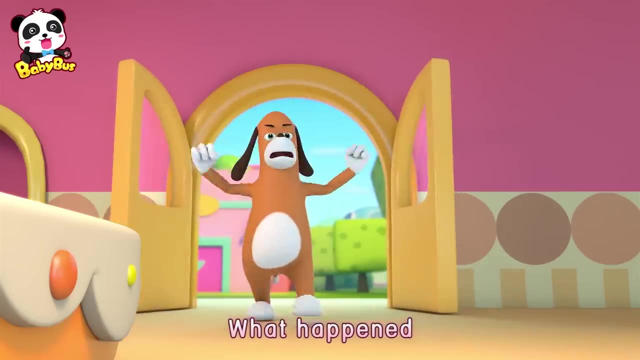 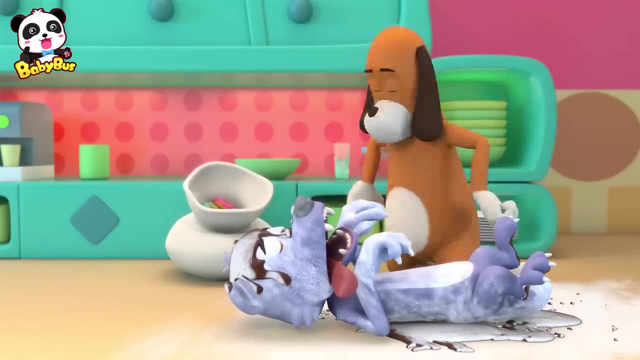 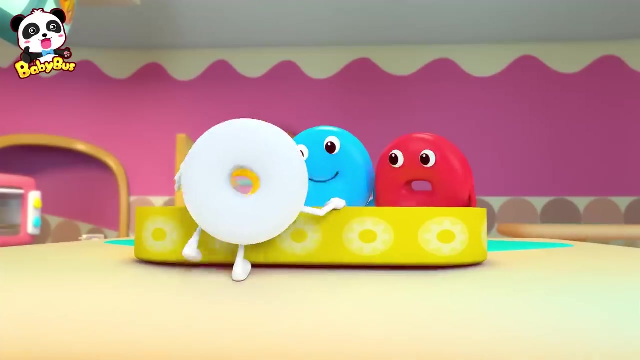 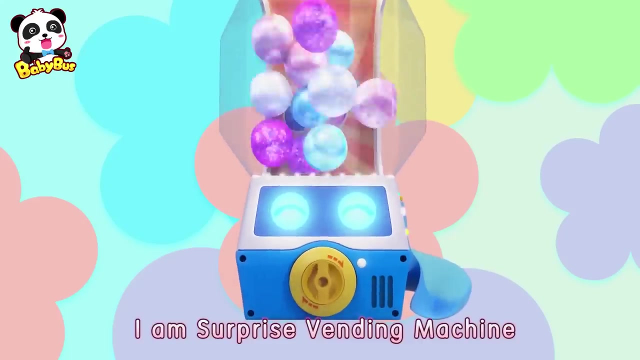 Then I'm gonna run Over there The blue donut. Run away, Run away from Wolf. I'm gonna hide Over there. P Tina, where are you? Is he gone? I am surprise. vending machine. Come and try, I will make you happy. 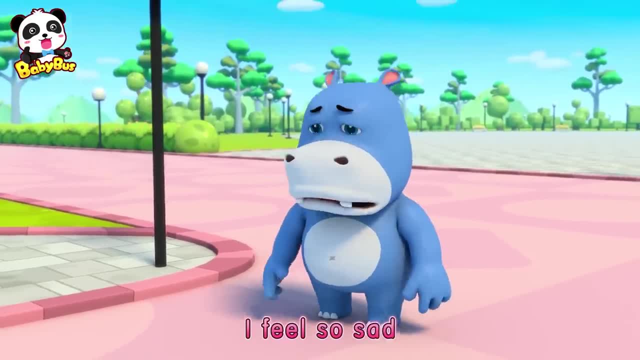 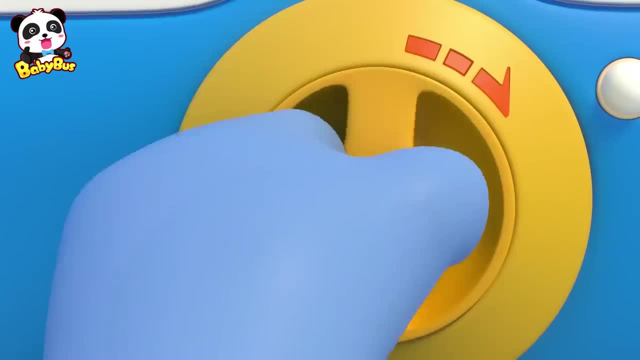 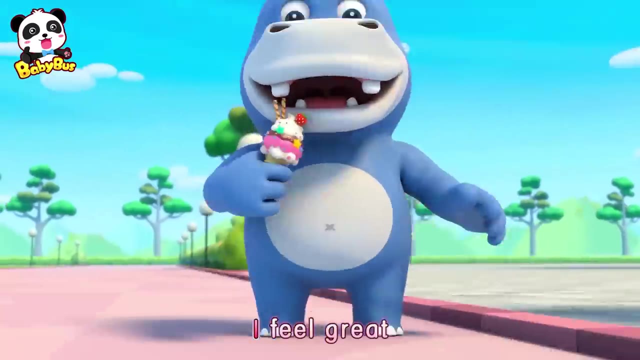 I feel sad. I feel so sad. Blue color is my mood. Here is a surprise to make you happy. Let's open it up. Wow, wow, wow. I feel great. Thank you, vending machine. Thank you, vending machine. 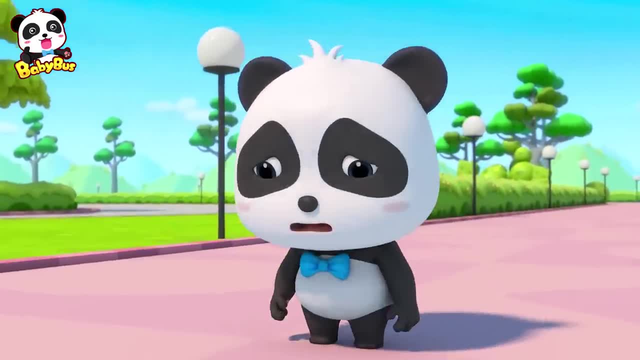 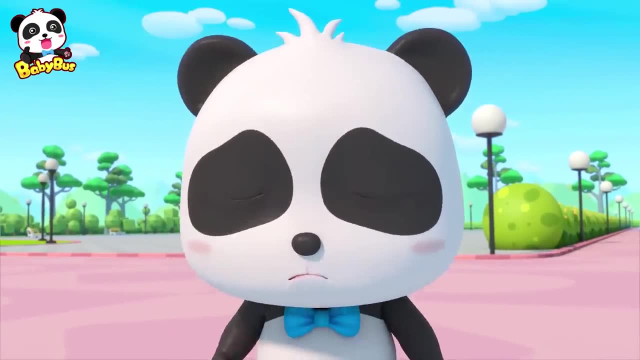 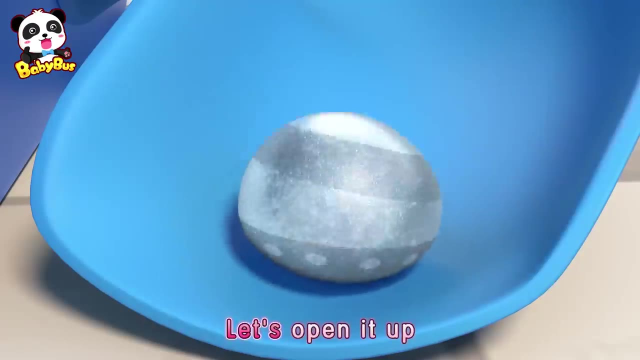 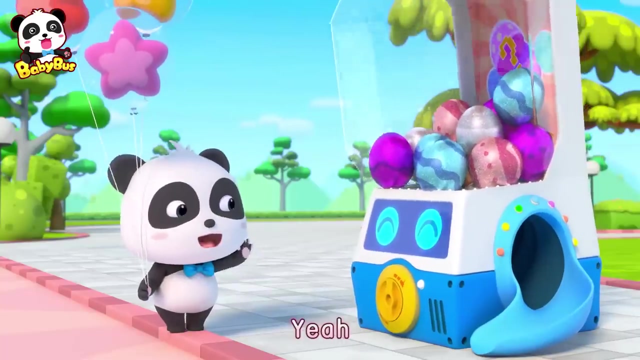 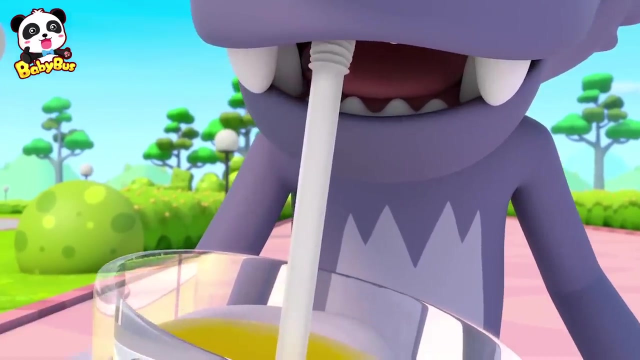 I feel upset. I feel upset. Gray color is my mood. Here is a surprise to make you happy. Let's open it up. Wow, wow, wow, I feel great. Yeah, Thank you. vending machine- What's this? 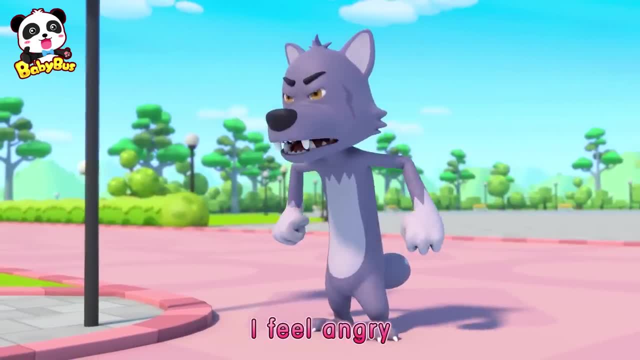 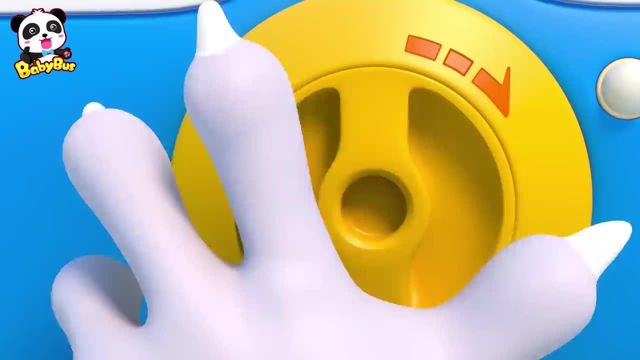 I feel angry. I feel angry. Red color is my mood. I feel scared. I feel scared. I feel scared. Purple color is my mood. I feel scared. I feel scared. Purple color is my mood. I feel scared. I feel scared. 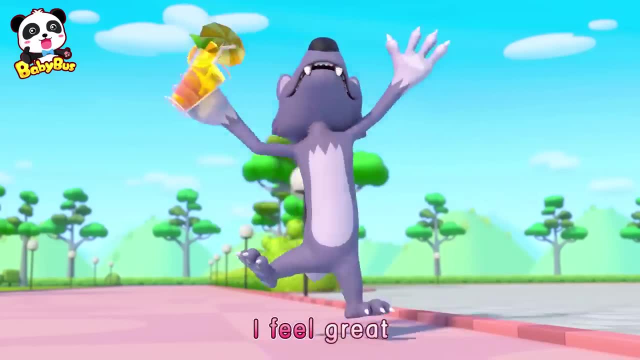 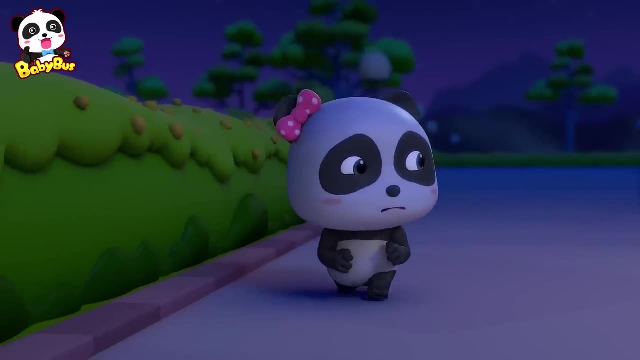 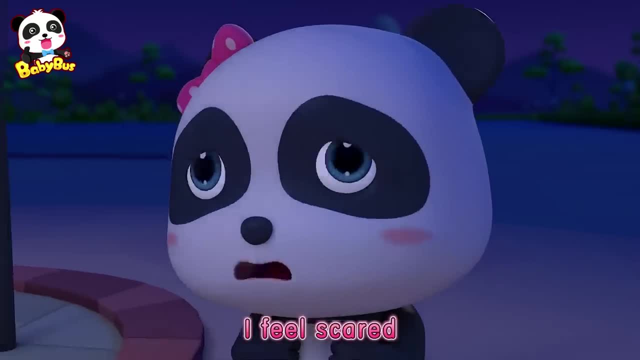 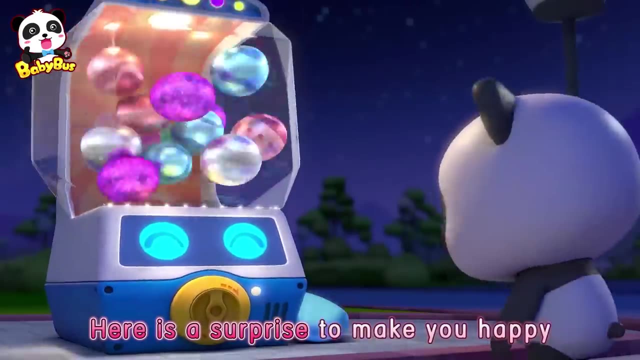 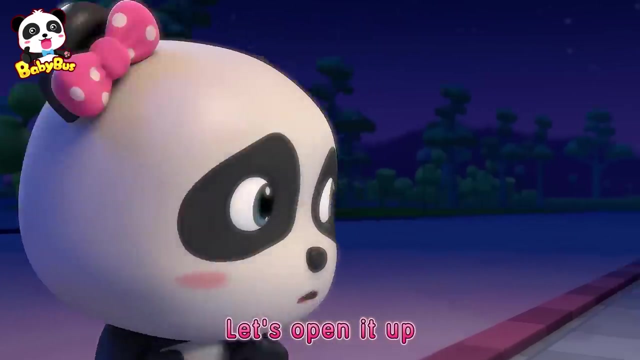 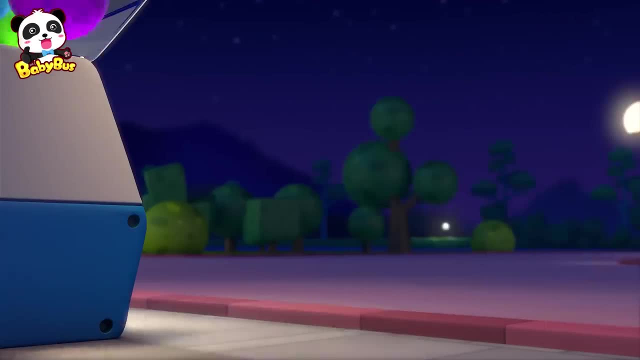 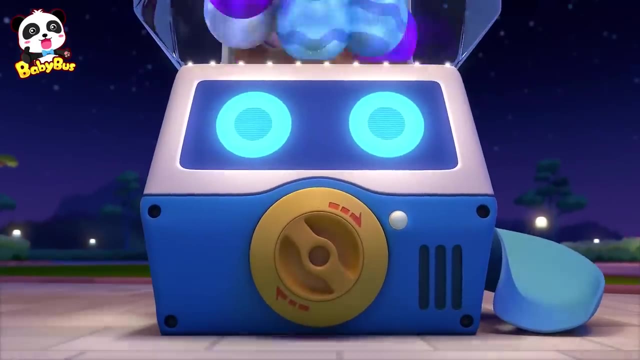 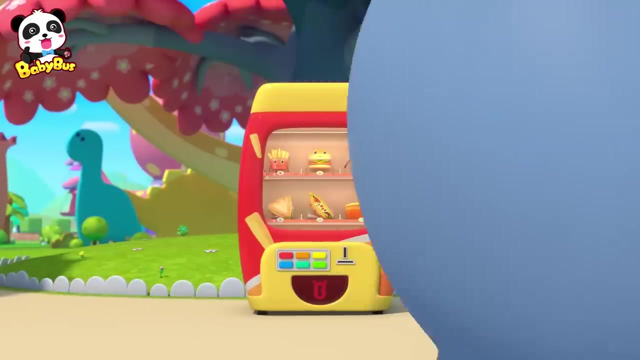 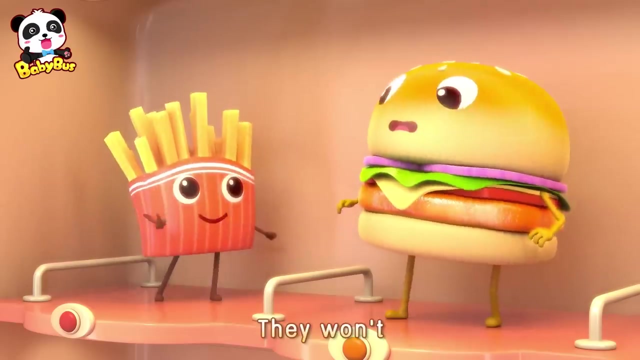 Thank you, vending machine. I feel great too. Kids, how do you feel today They're going to pick me first because I'm the best? No, they won't. They will pick me first. You two are both wrong. I'm sure they will pick me first. 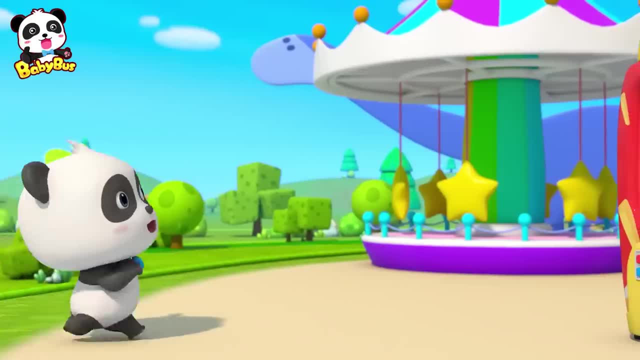 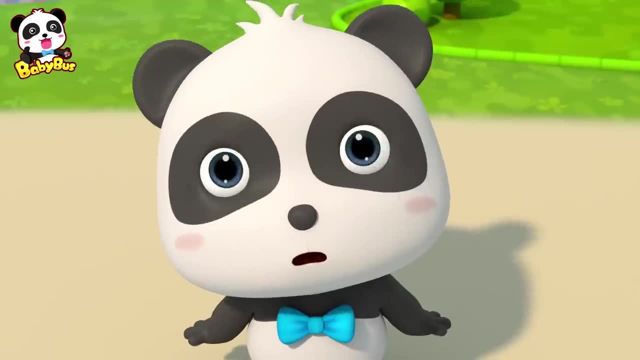 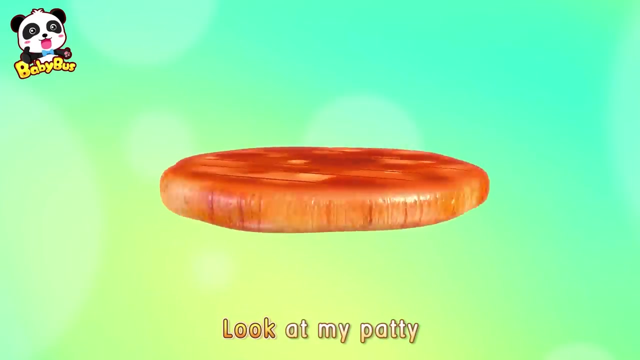 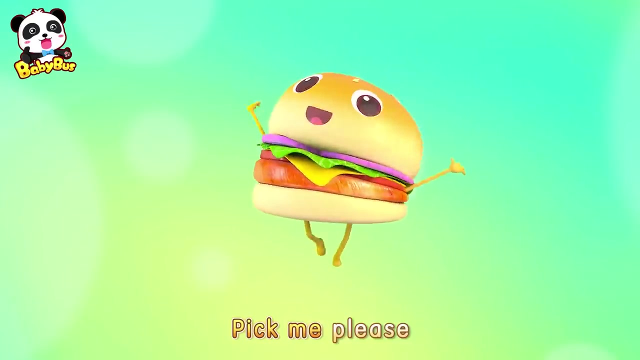 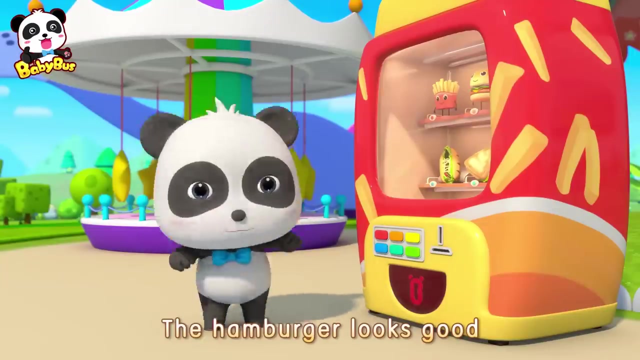 Someone's coming. Which one should I pick? Here I am the yummy hamburger. Look at my patty. It looks so good. I've been waiting for you. Pick me please. Yummy hamburger is ready to go. Wow, the hamburger looks good. 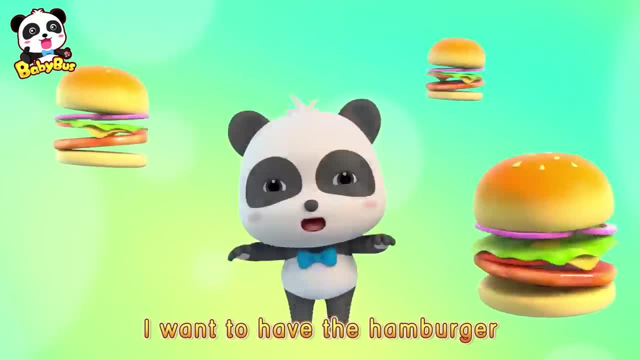 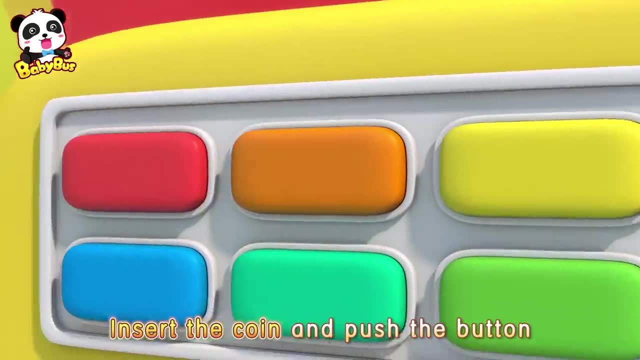 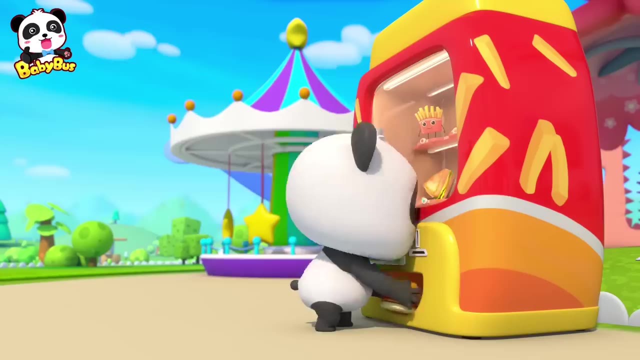 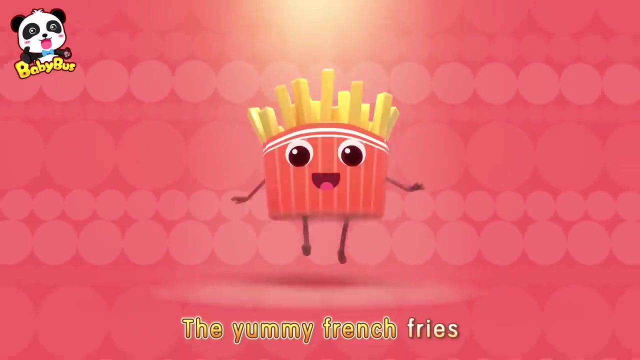 I want to have the hamburger. Look at the patty. It looks so good. Insert the coin and push the button. Yummy hamburger. please come out. Here I am the yummy french fries. I'm so crispy and I smell great. 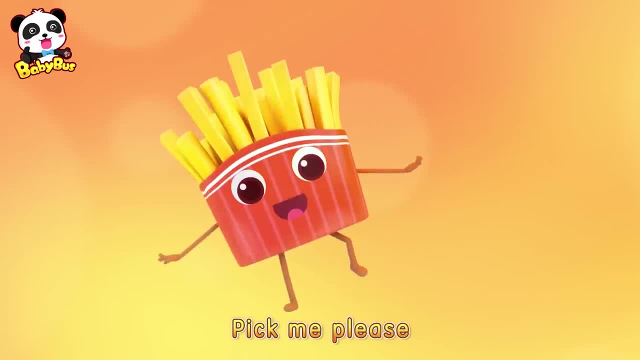 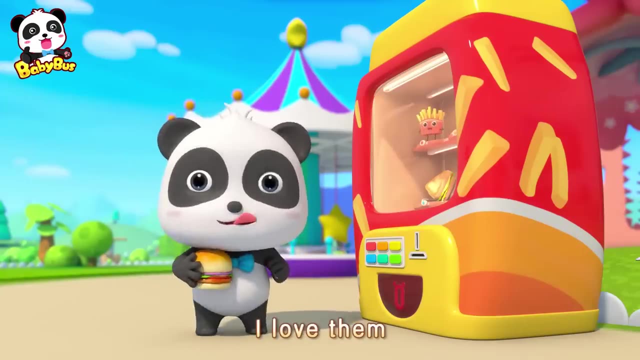 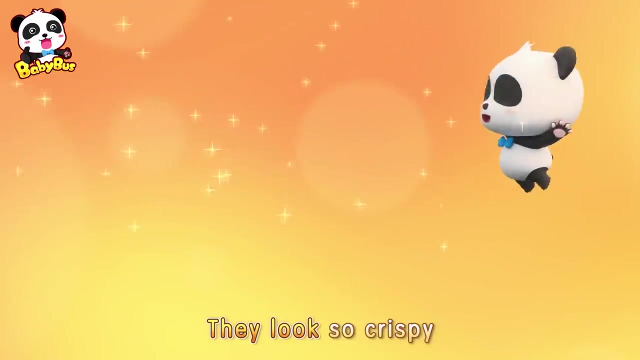 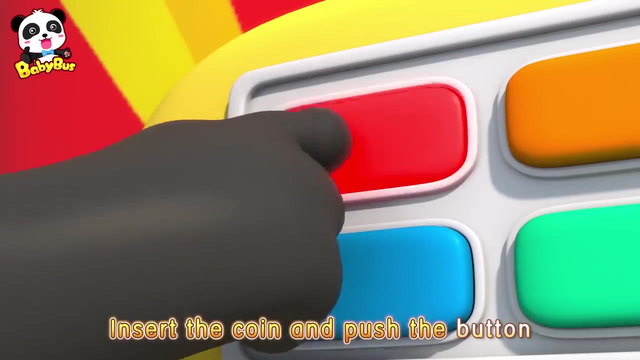 I've been waiting for you. Pick me, please. Yummy french fries. They are ready to go. French fries, I love them. I want to have the yummy french fries. They look so crispy and they smell great. Insert the coin and push the button. 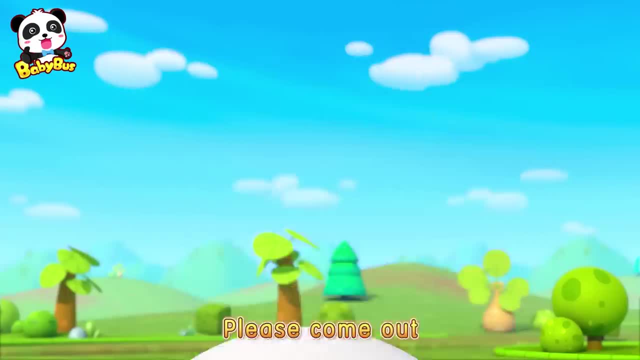 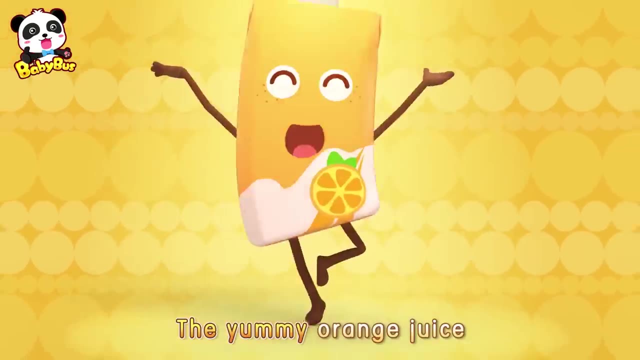 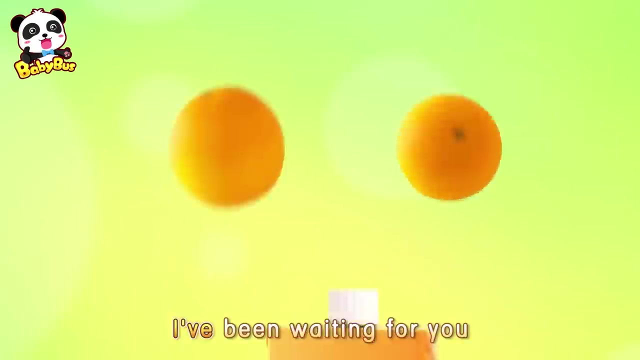 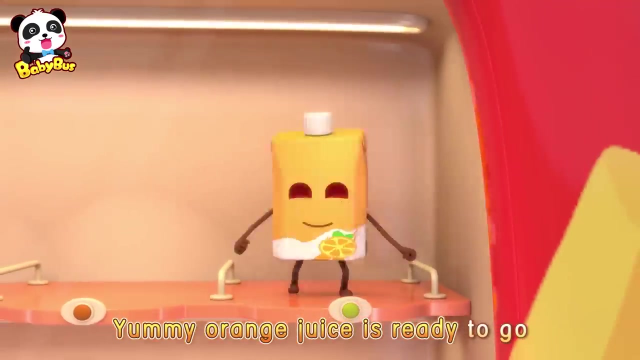 Yummy french fries. please come out. Here I am the yummy hamburger. I want to have the yummy orange juice. I'm so fresh and I'm so sweet. I've been waiting for you. Pick me, please. Yummy orange juice is ready to go. 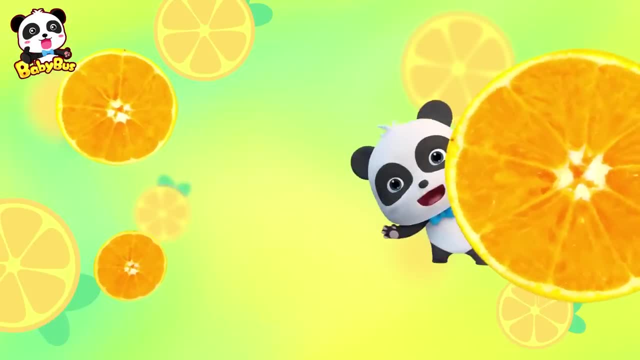 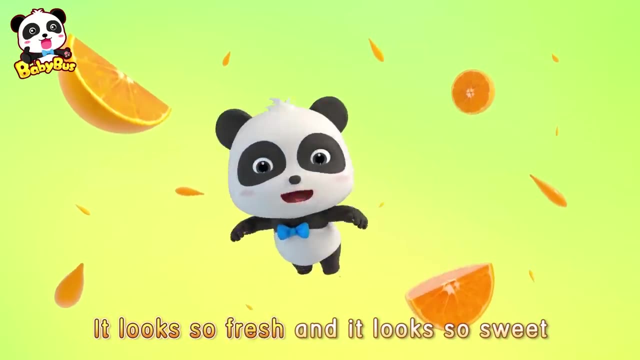 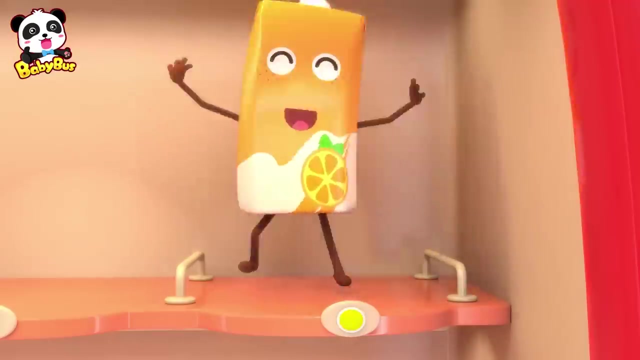 I'll have the orange juice too. I want to have the yummy juice. It looks so fresh and it looks so sweet. Insert the coin and push the button. Insert the coin and push the button. Yummy orange juice. please come out. 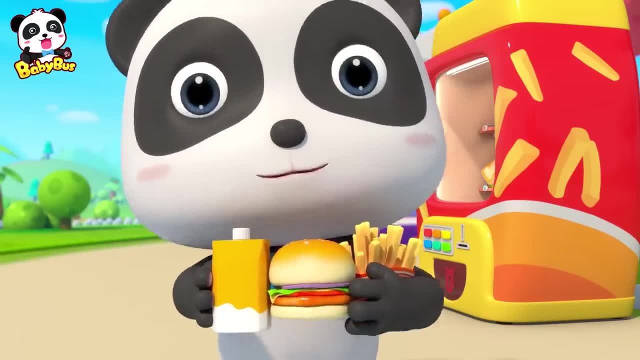 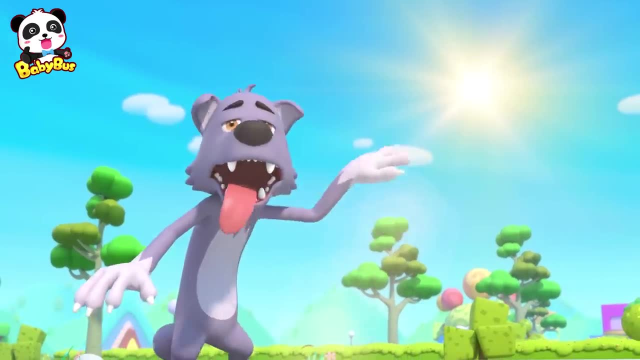 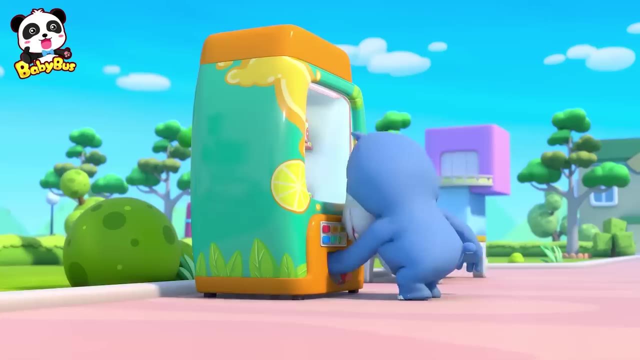 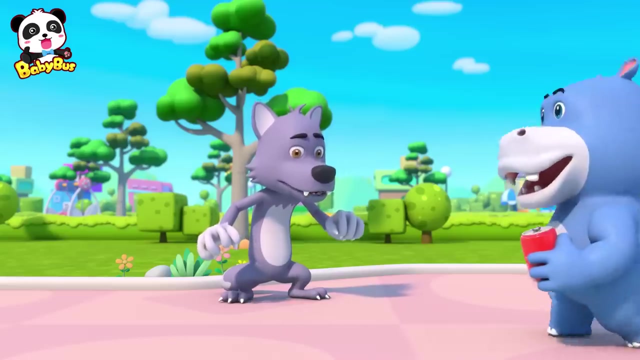 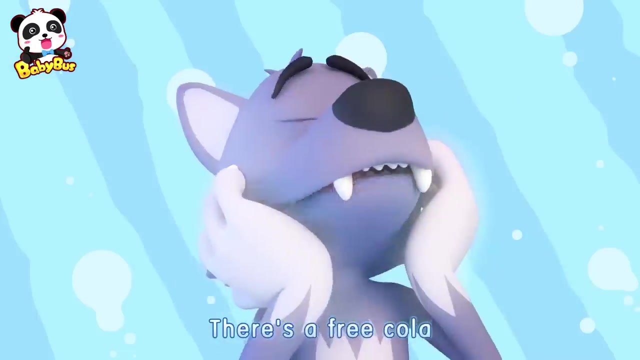 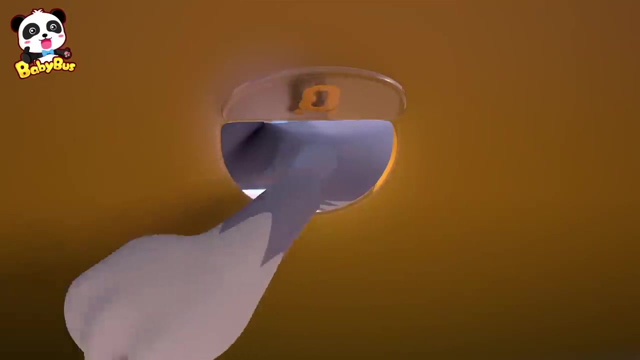 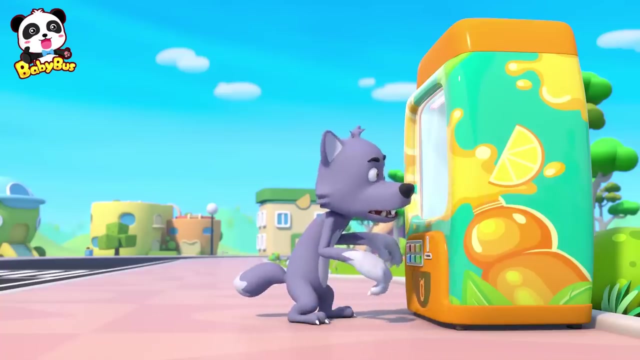 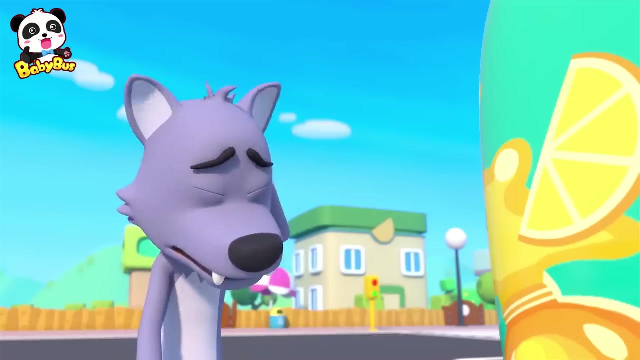 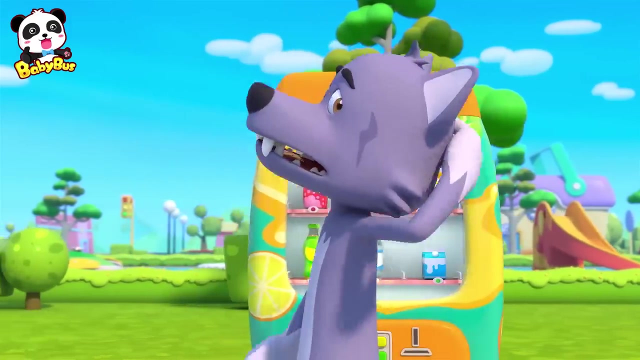 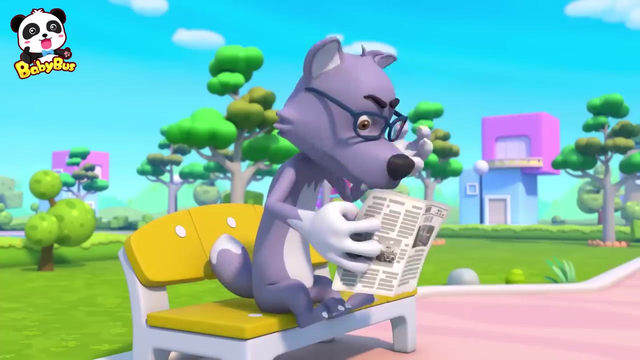 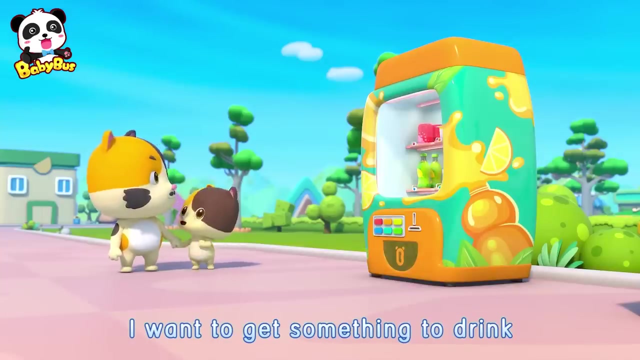 Look, I have lots of yummy food. I really want a cola. Huh, Cola cola. there's a free cola. Where is the cola? The machine must be broken. How can I get a cola, Dad? I want to get something to drink. 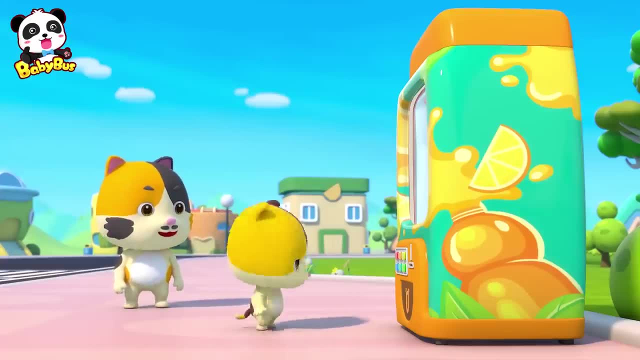 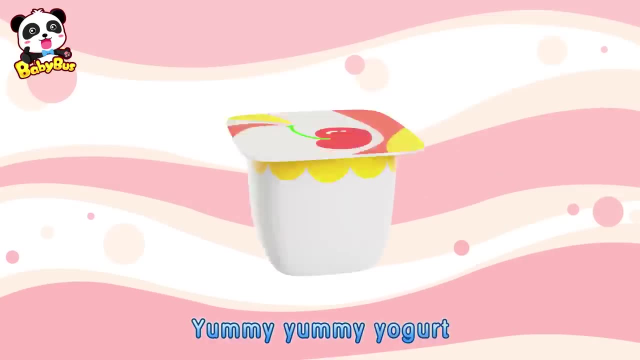 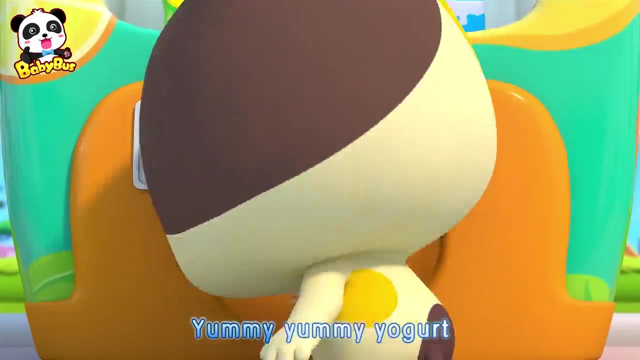 A vending machine with a lot of drinks. Wow, I'll have it. I'll have it. Yummy, yummy yogurt, yeah. Put the coin and push the button now. Rattle, rattle, rattle. Yummy yummy yogurt, yeah. 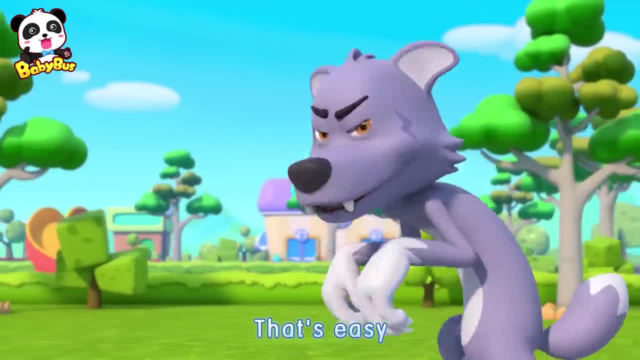 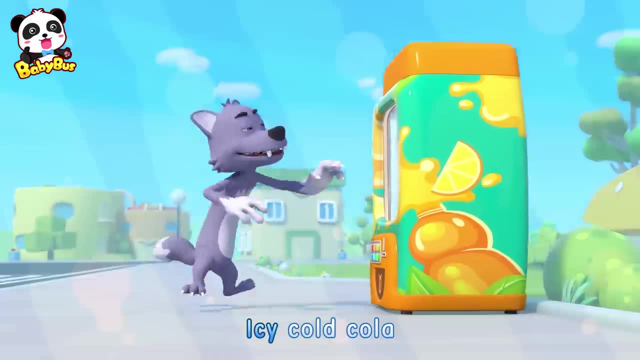 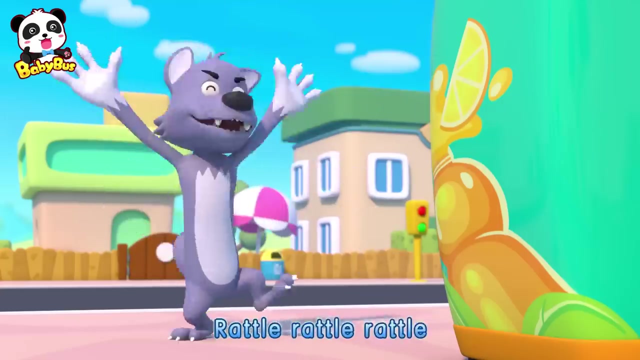 Oh, I should push the button. That's easy. A vending machine with a lot of drinks? Wow, I'll have it. I'll have it. Icy cold cola. Push the button now. Push the button now. Rattle, rattle, rattle. 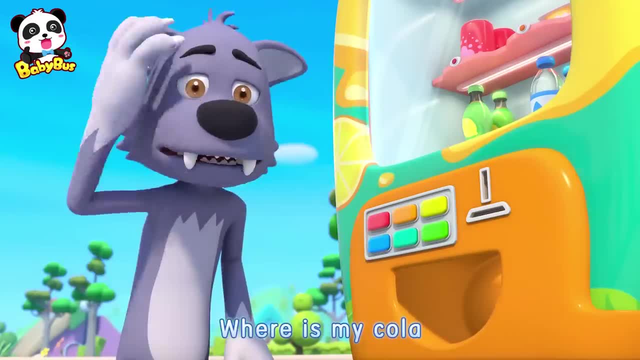 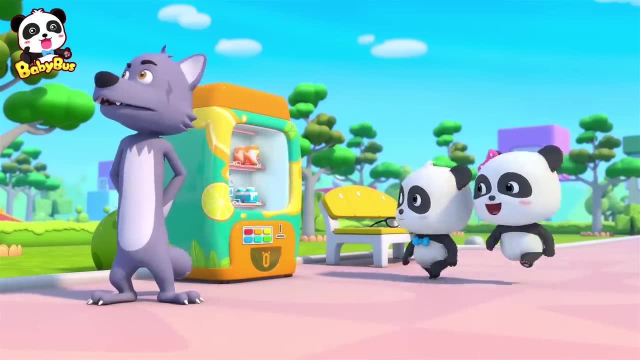 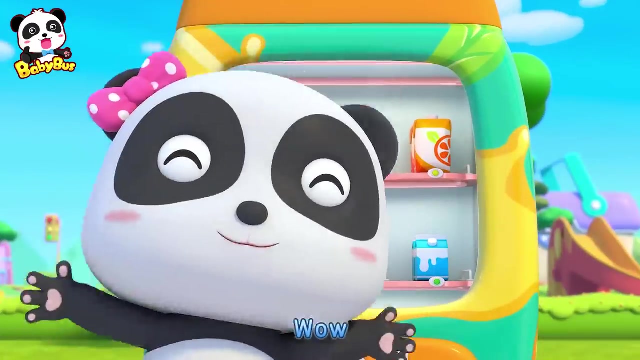 Icy cold cola. Oh, where is my cola? Here's a vending machine, A vending machine with a lot of drinks. Wow, I'll have it. I'll have it. Sweet fruit juice: yeah, Put the coin and push the button now. 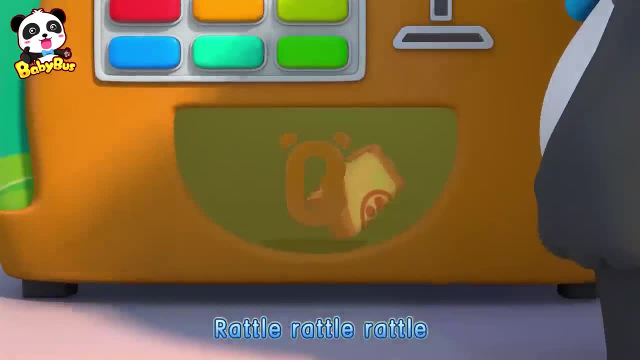 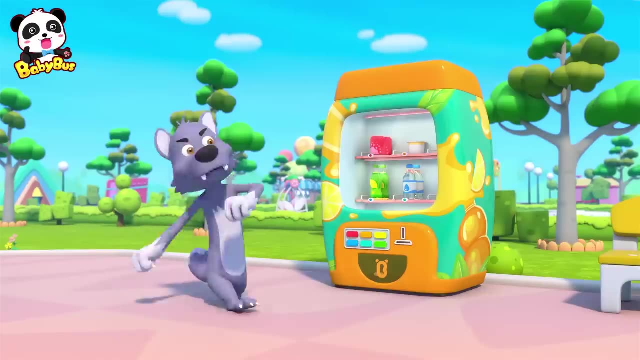 Rattle, rattle, rattle. Sweet fruit juice. yeah, I should insert the coin too. A vending machine with a lot of drinks? Wow, I'll have it. I'll have it. Icy cold cola. Put the coin in. 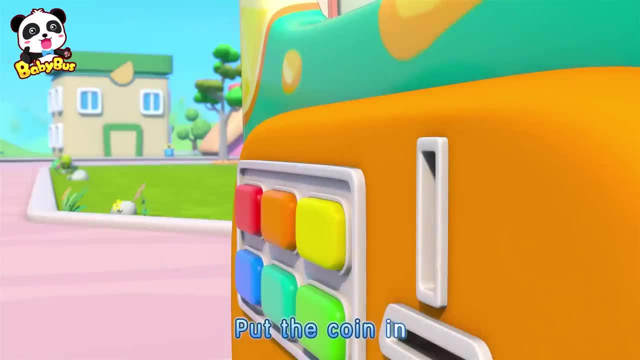 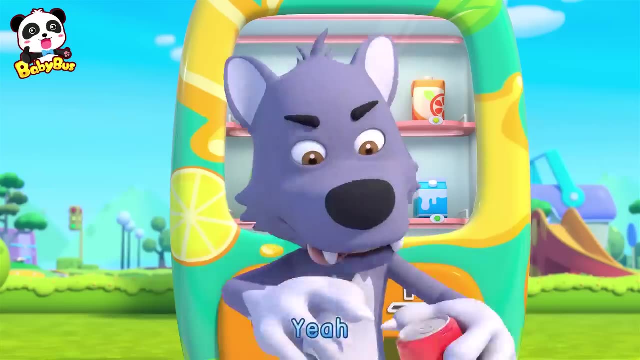 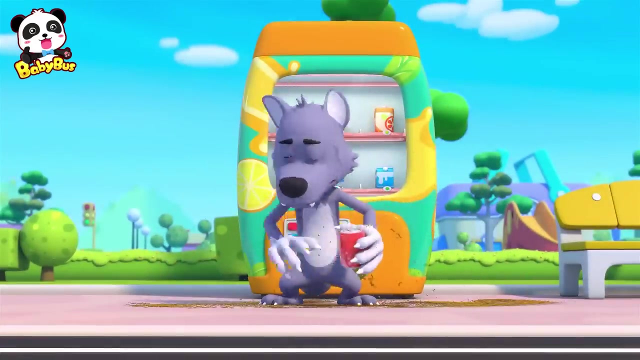 Push the button now. Rattle, rattle, rattle Icy cold cola. Yeah, Put the coin in. Push the button now. Rattle, rattle, rattle Icy cold cola. Push the button now. Icy cold cola. 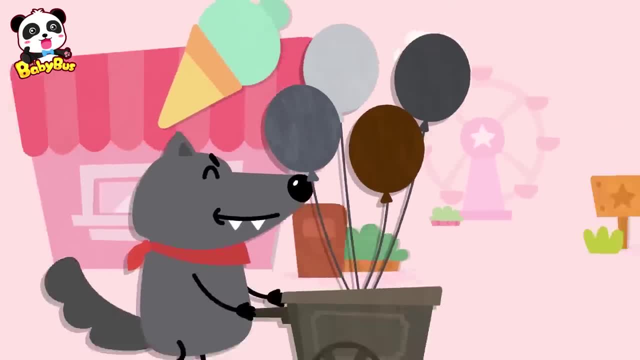 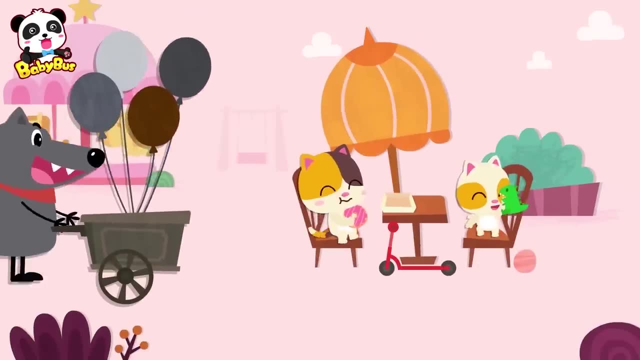 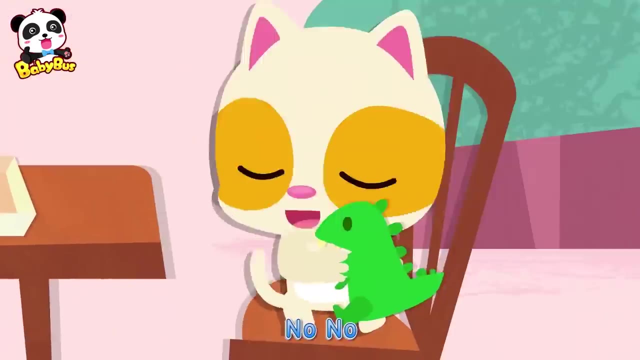 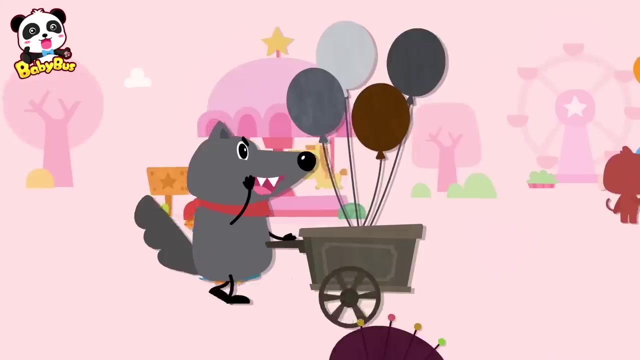 Put the coin in, Push the button now. Icy cold cola. Make sure you have it. Icy cold cola. Hey kids, Do you want some balloons? Those are not very pretty. I only like pink, No Balloons. 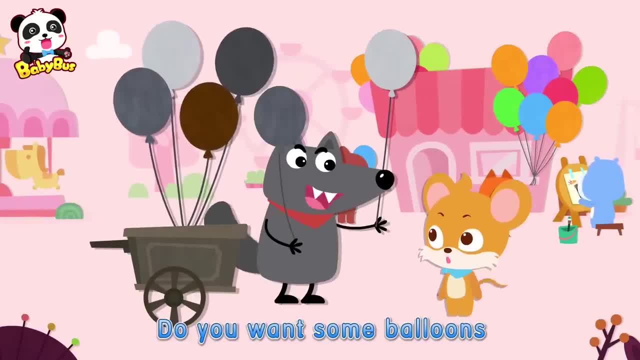 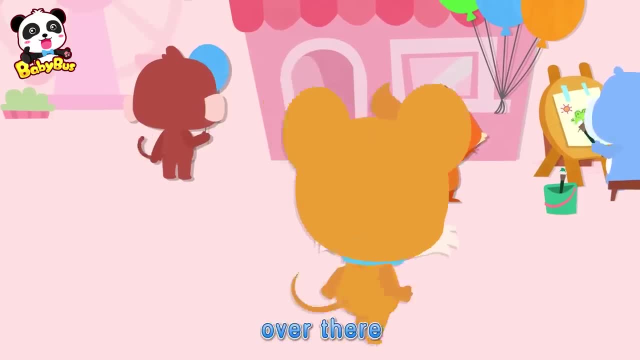 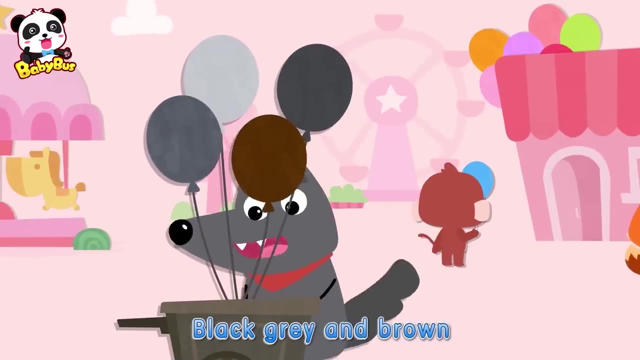 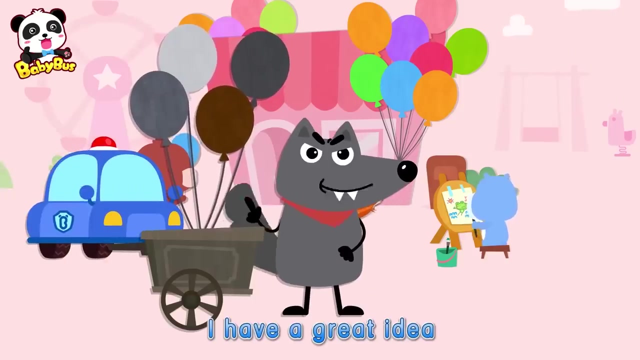 Balloons. Hey, kid, do you want some balloons? No thanks, I'm gonna buy the colorful balloons over there. Ah, colorful balloons are not pretty. Black, gray and brown are much prettier. Ah-ha, I have a great idea. 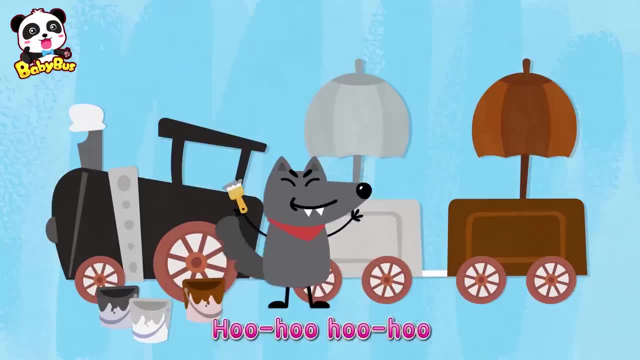 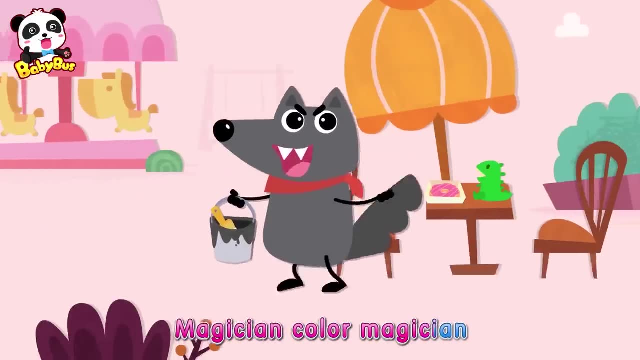 Hoo-hoo-hoo-hoo change, Hoo-hoo-hoo-hoo change. I'm gonna change all colors to black, gray and brown. Magician, color magician, the color of the donut. change, change, change. 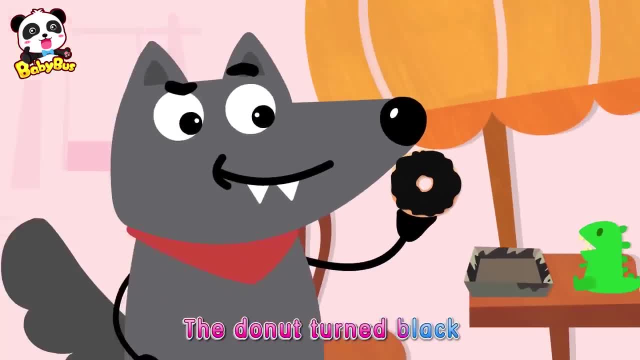 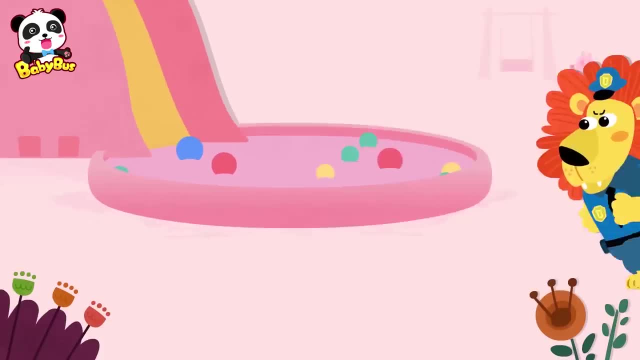 Ya-ha, ya-ha, The donut turned black. Police car, police car, find somewhere to hide. Ha-ha-ha-ha, Ha-ha. Where are you? where are you, Hey wolf, come out now. 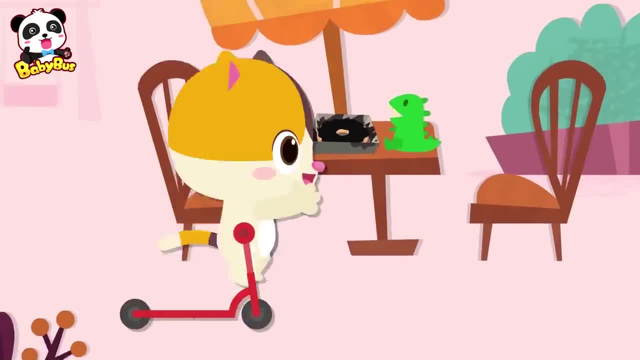 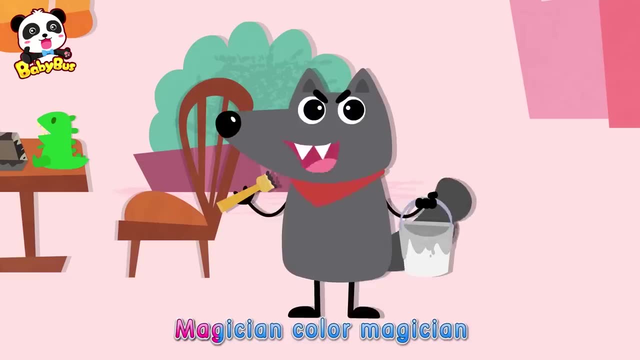 Ah, that was close My donut. Why did it turn black? Ha-ha-ha-ha, Magician, color magician, the color of the dino, change, change, change, Ya-ha, ya-ha. 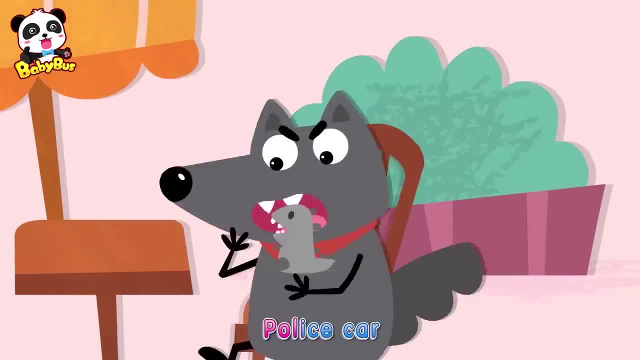 The dino turned gray Police car, police car, find somewhere to hide. Hoo-hoo-hoo-hoo, Ha-ha-ha-ha, Ha-ha-ha-ha, Ha-ha-ha-ha, Hoo-hoo-hoo-hoo. Hoo-hoo-hoo-hoo, Hoo-hoo-hoo, Hoo-hoo-hoo-hoo, Hoo-hoo-hoo-hoo, Hoo-hoo-hoo-hoo, Hoo-hoo-hoo-hoo. 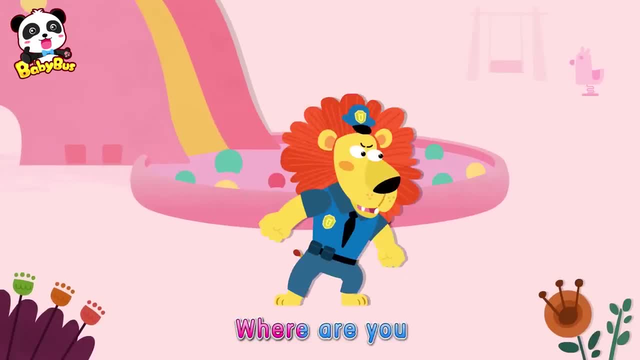 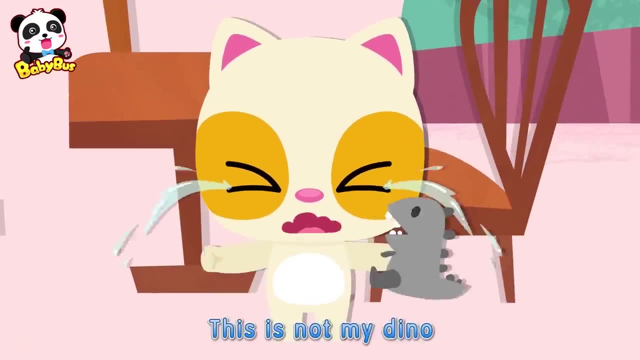 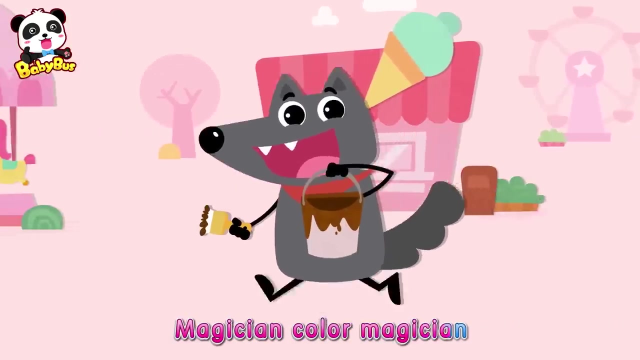 Ho, ho, ho, ho, ho, ho ho. where are you? Where are you? Hey wolf, come out now. Ah, that was close. This is not my dino Magician, color magician, the color of the merry-go-round change. 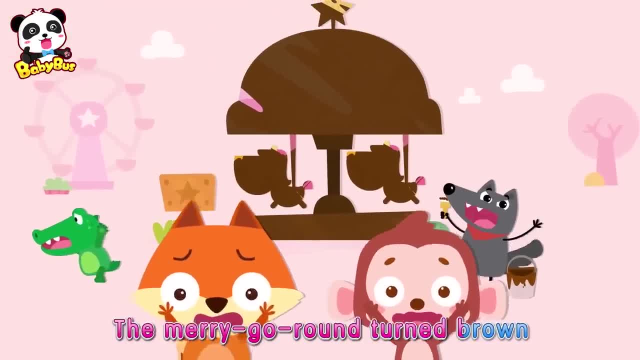 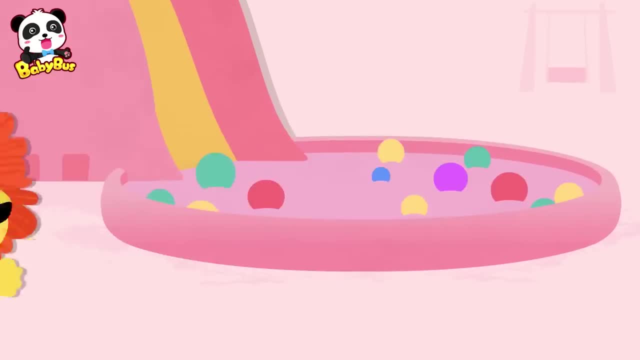 Ya-ha, ya-ha, the merry-go-round turn brown Police car, police car, find somewhere to hide. Ho ho, ho, ho, ho, ho ho. where are you? Where are you? Hey wolf, come out now. 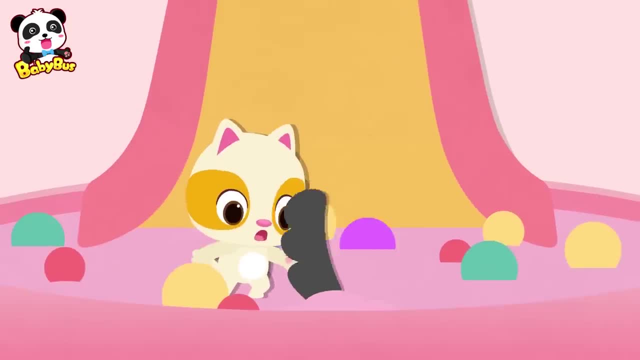 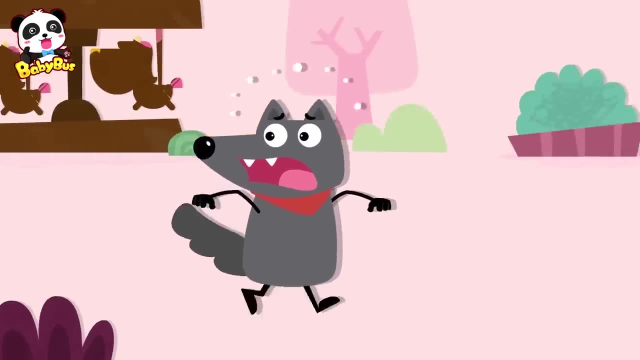 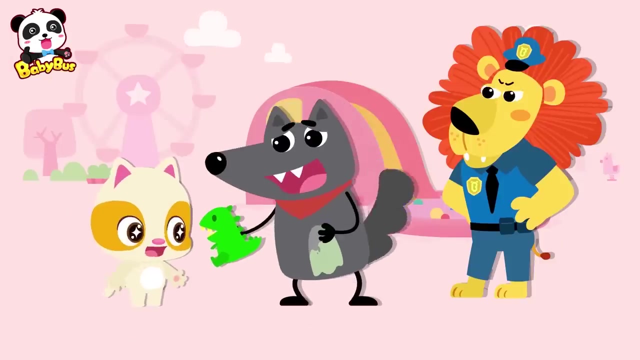 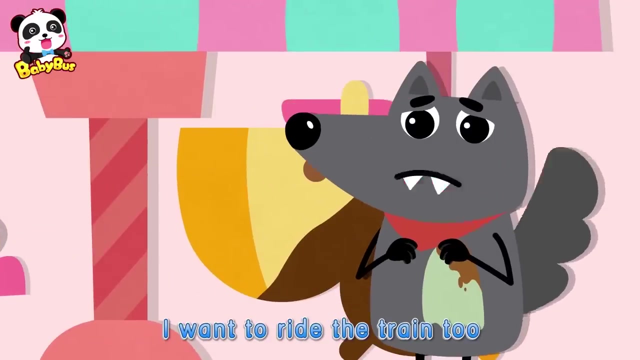 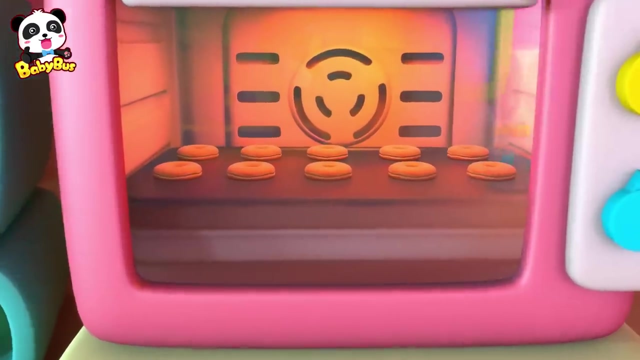 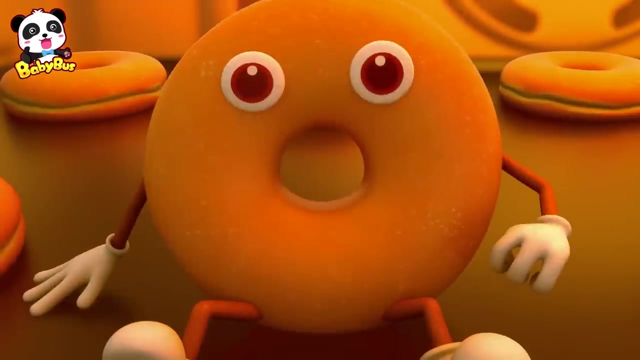 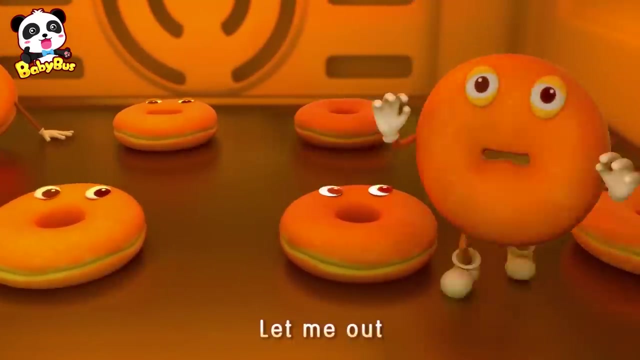 Ah, that was close. What's this? It's the wolf. Oh, they found me. Huh, I'm so tired. I want to ride the train too. Huh, Oh ow, my butt is burning. It's so hot in here. Help, Let me out. Let me out. 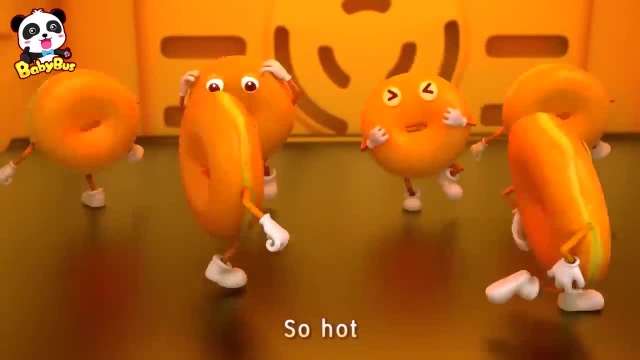 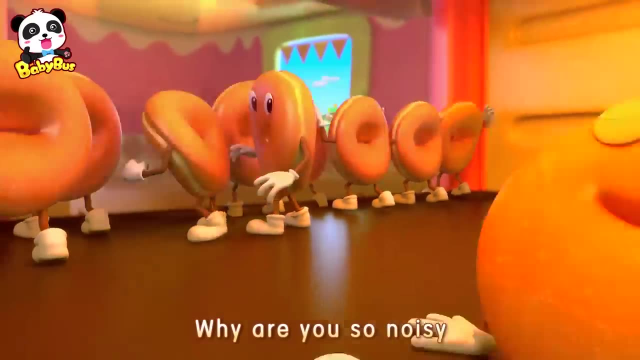 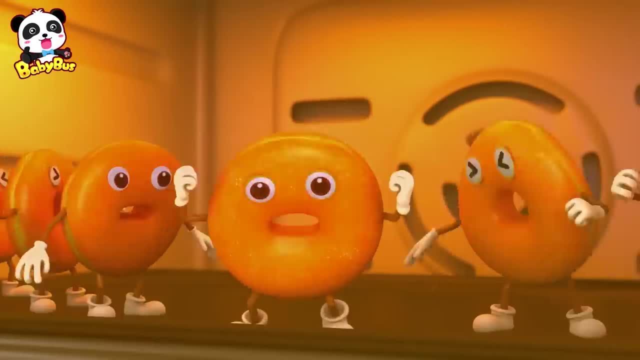 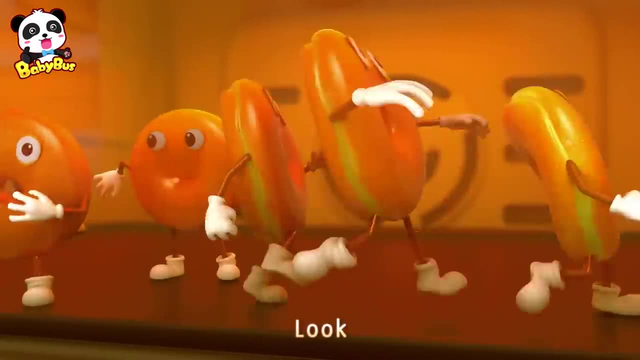 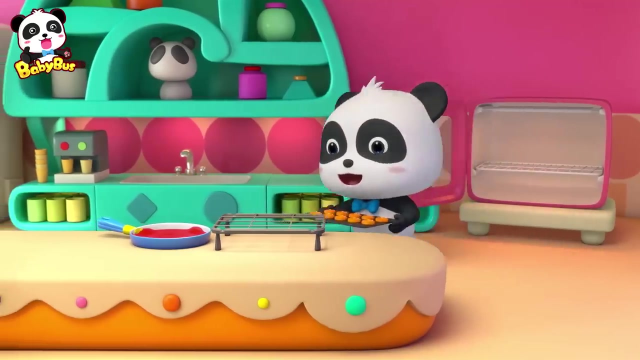 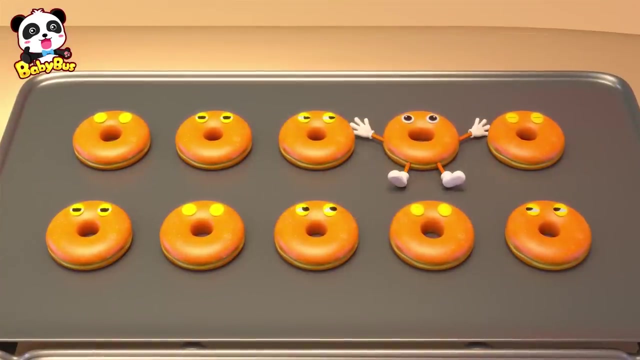 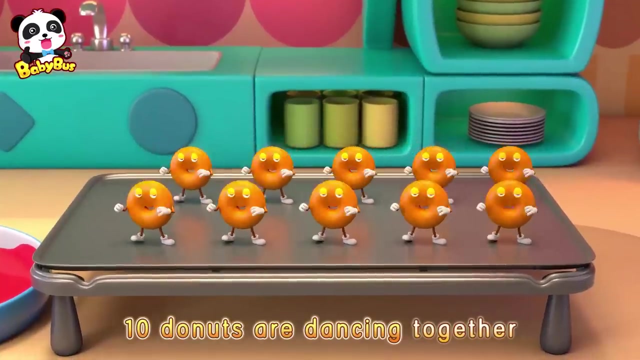 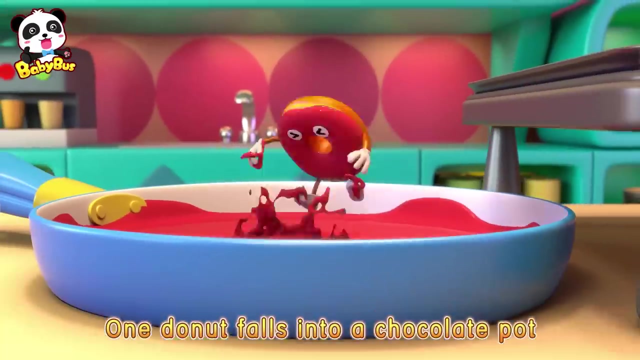 It's so hot, Let me out, Let me out, Let me out. Look somebody's coming. Shall we dance. Ten doughnuts are dancing together. Turn around, turn around. One doughnut falls into a chocolate pot. Red. Nine doughnuts are dancing together. 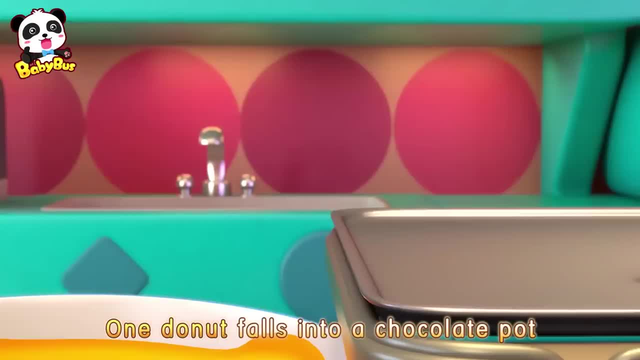 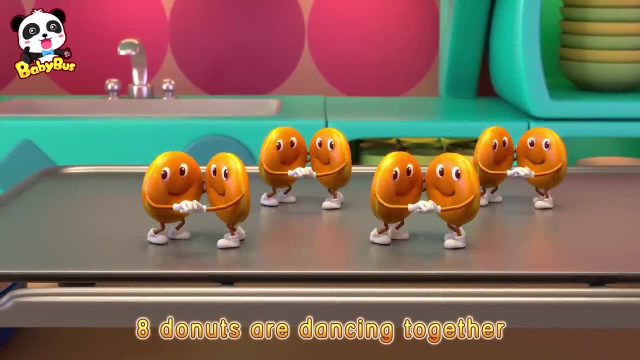 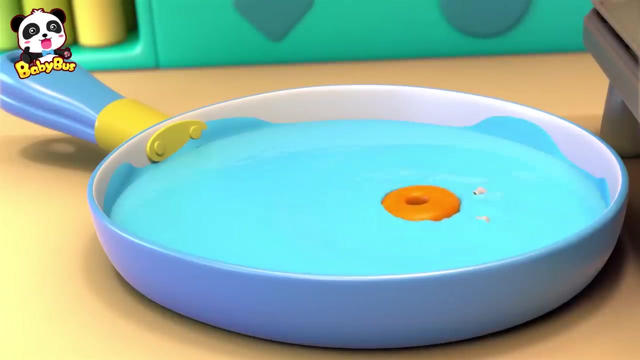 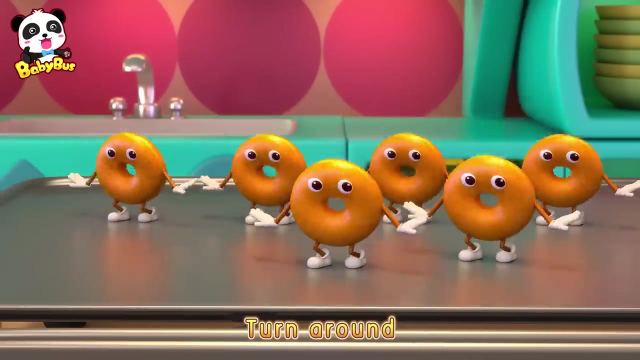 Roll over, roll over. One doughnut falls into a chocolate pot. Yellow: Eight doughnuts are dancing together, Turn around, turn around. One doughnut falls into a chocolate pot. Blue: Seven doughnuts are dancing together, Turn around, turn around. One doughnut falls into a chocolate pot. 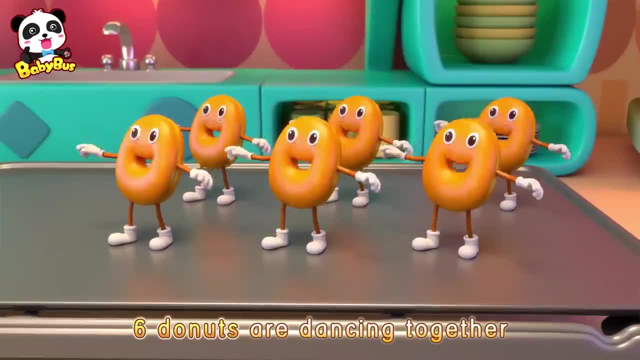 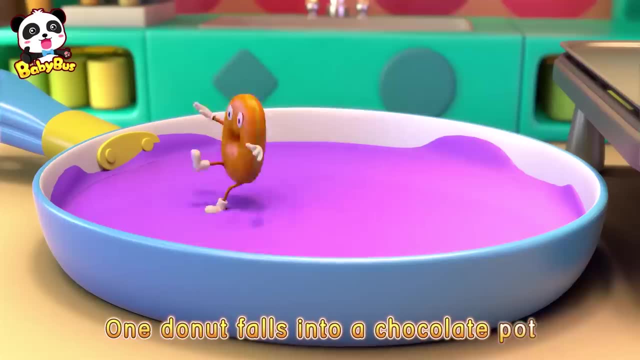 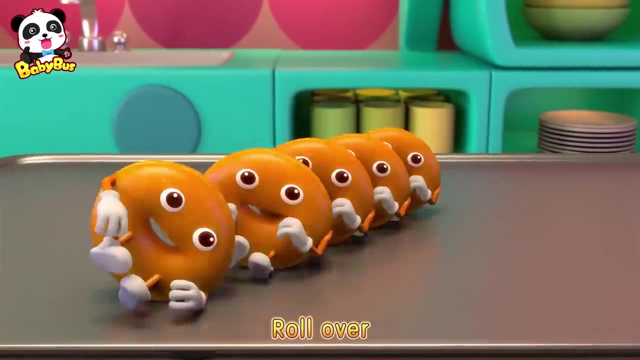 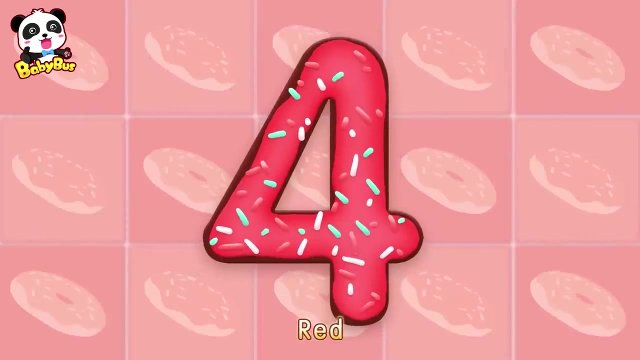 Green: Six doughnuts are dancing together, Turn around, turn around. One doughnut falls into a chocolate pot. Purple: Five doughnuts are dancing together, Roll over, roll over. One doughnut falls into a chocolate pot. Red: Four doughnuts are dancing together, Turn around, turn around. 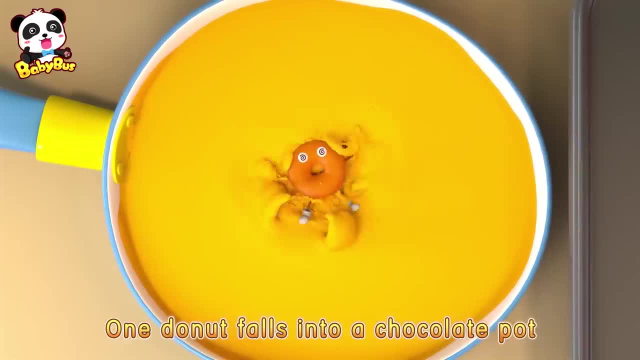 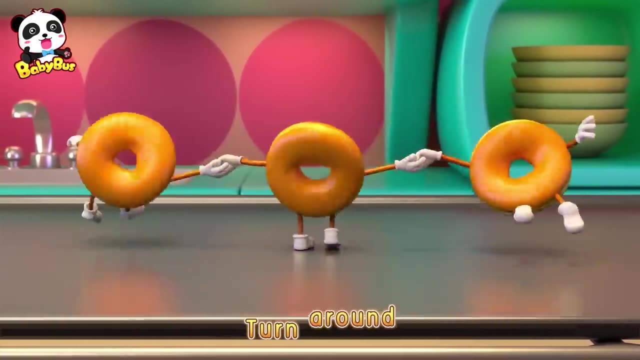 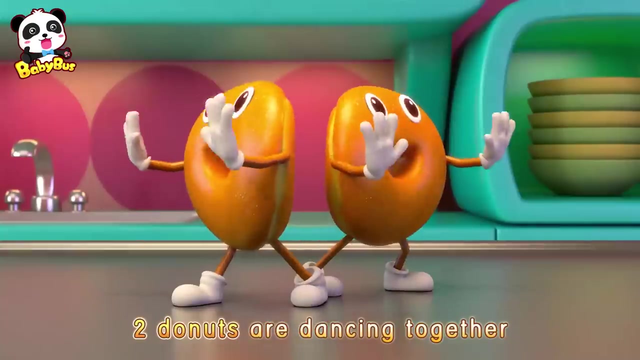 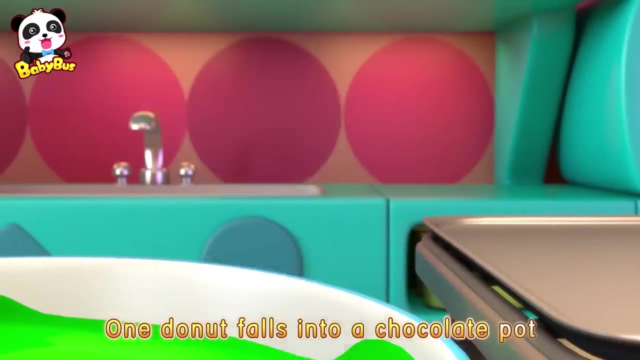 One doughnut falls into a chocolate pot. Yellow: Three doughnuts are dancing together, Turn around, turn around. One doughnut falls into a chocolate pot. Blue: Two doughnuts are dancing together, Turn around, turn around. One doughnut falls into a chocolate pot. Green: One doughnut falls into a chocolate pot. 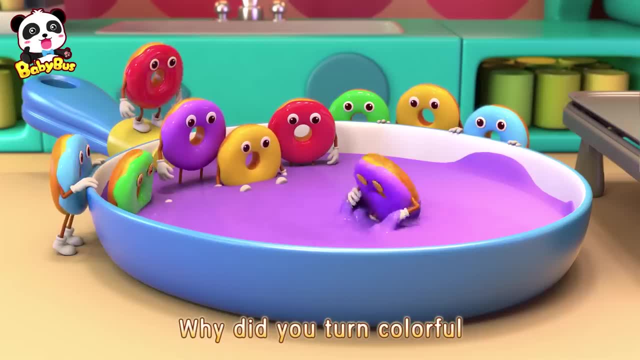 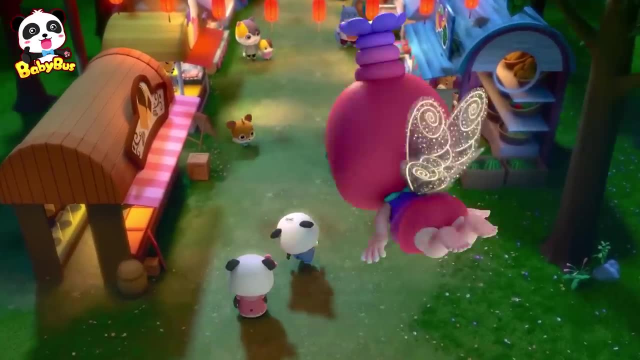 Why did you turn colorful? Because you would elude people. Leave a comment to let me know So that I don't write stupid letters. Let me know if you have any unlucky impertinences. See you next time. 2, Three, As expected. there's something called red. 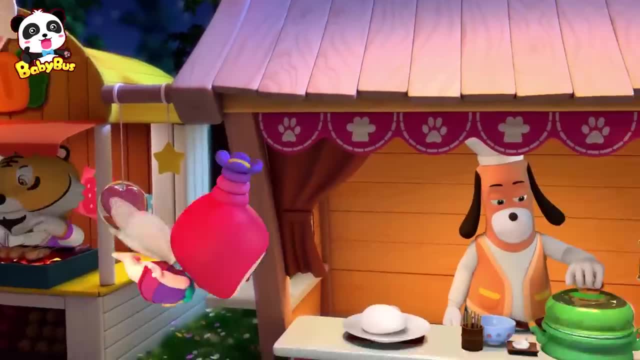 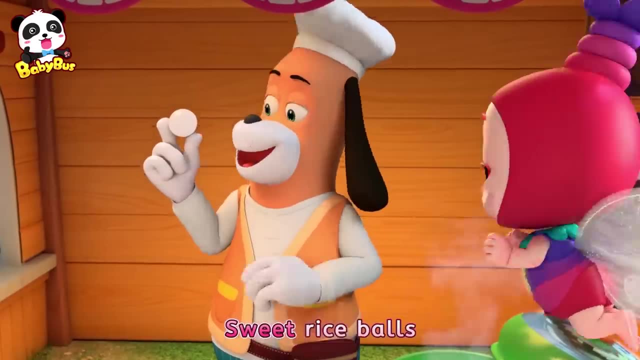 If you can't put it in, You just have to put right here. Maybe if you try this You'll find your way. Can it hold? three follows, Three, No, three, No A whole. Who wants to ride a horse? Street food- What would that be? 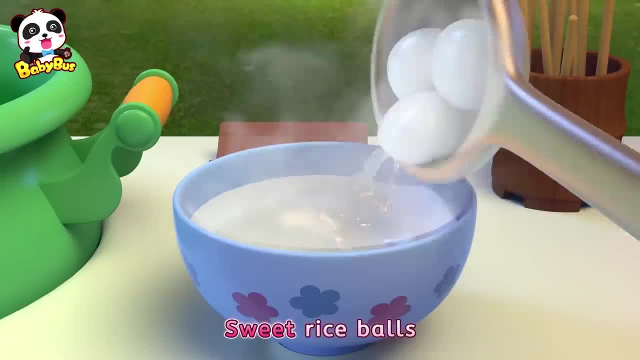 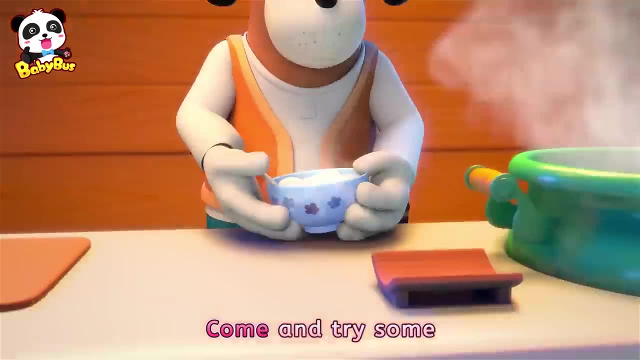 I don't know. Middletown Sweet rice balls, sweet rice balls. Do you wanna have some sweet rice balls? A bowl of round and sweet rice balls. Come and try some, you'll like them. Rice balls, rice balls- round and sweet. 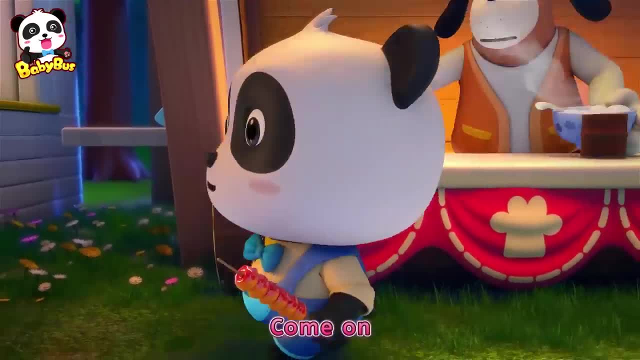 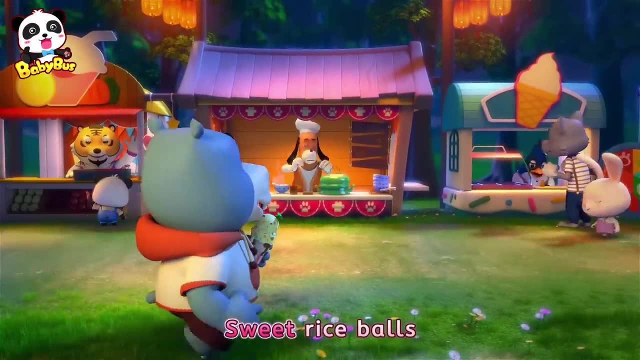 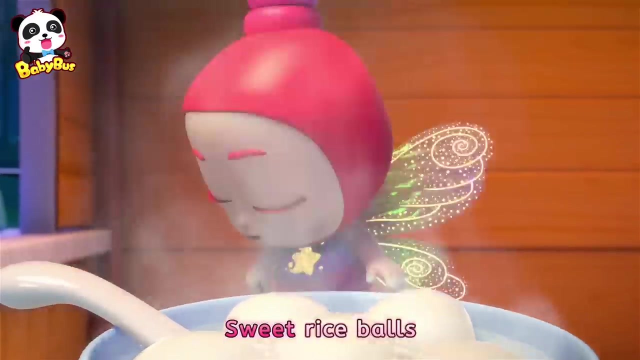 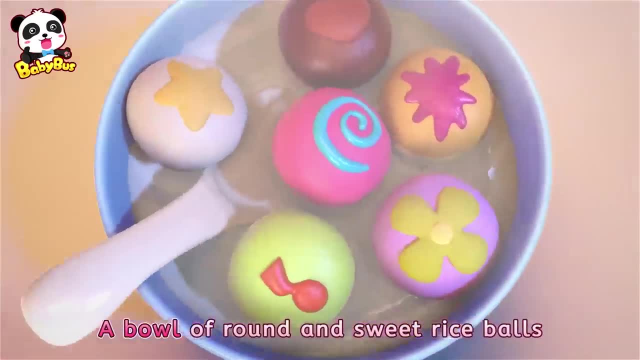 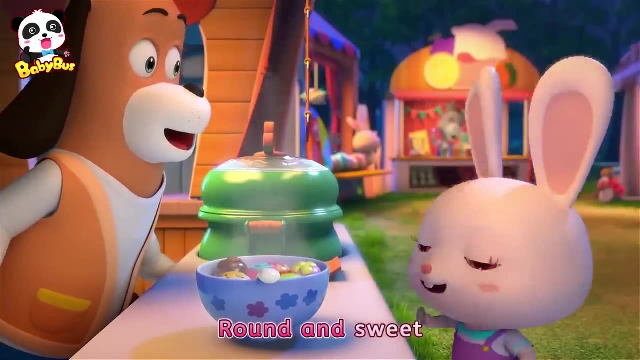 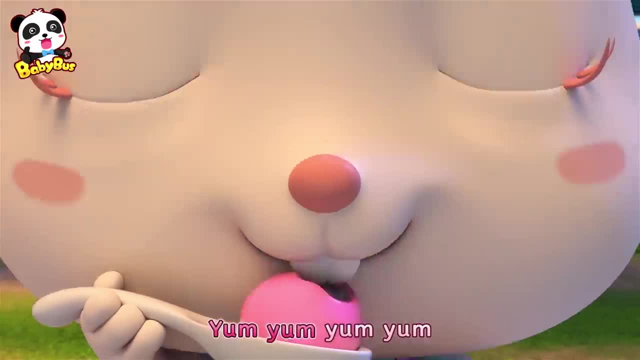 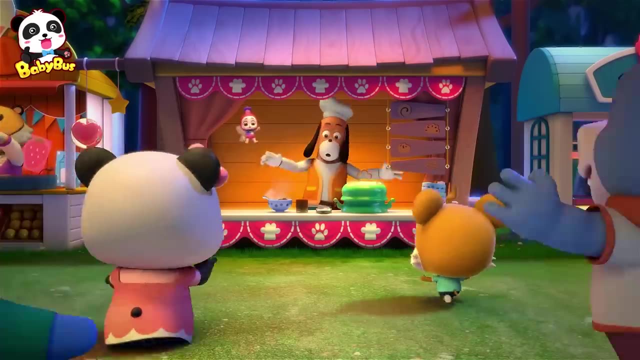 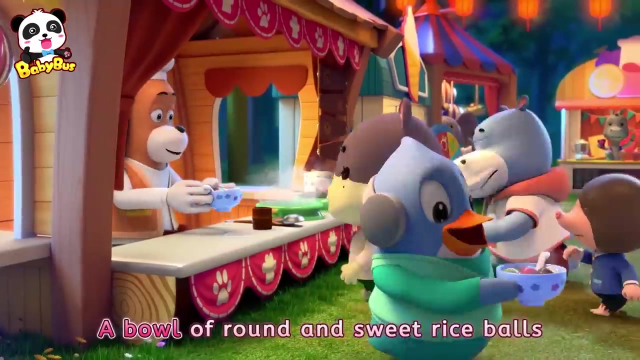 Rice balls, rice balls, round and sweet. Yum yum, yum, yum yum, sweet, Sweet rice balls. Sweet rice balls, sweet rice balls. Do you wanna have some sweet rice balls? A bowl of round and sweet rice balls. Come and try some. you'll like them. 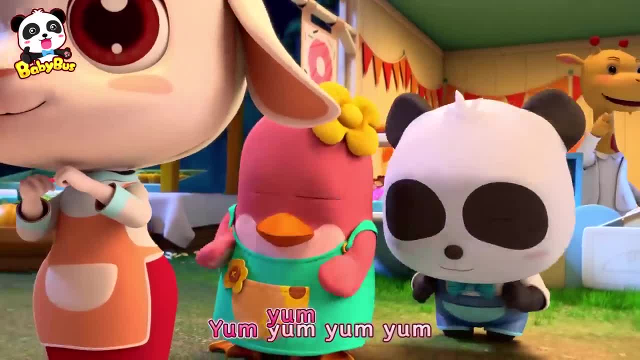 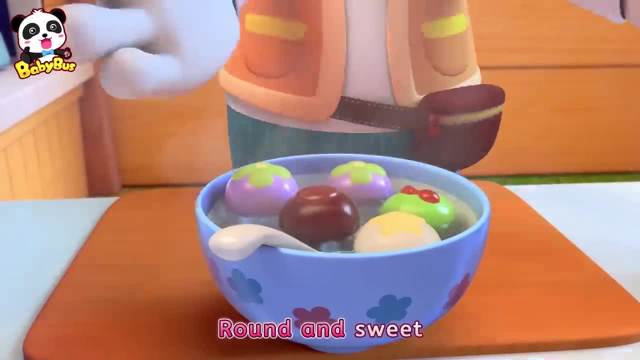 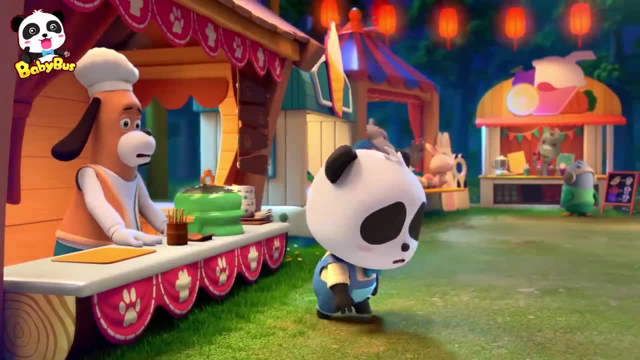 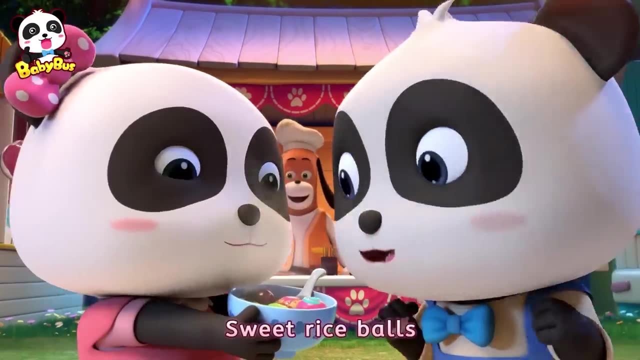 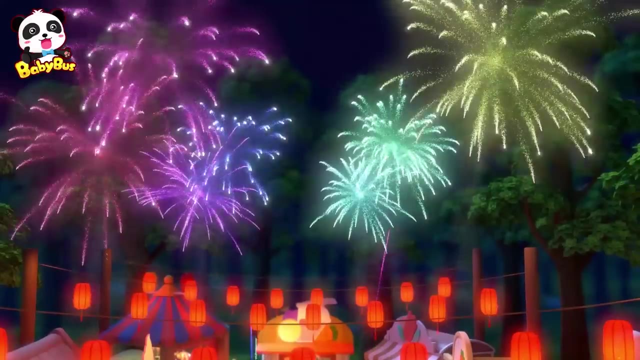 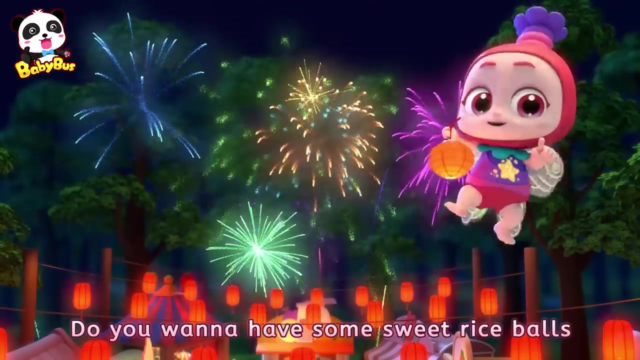 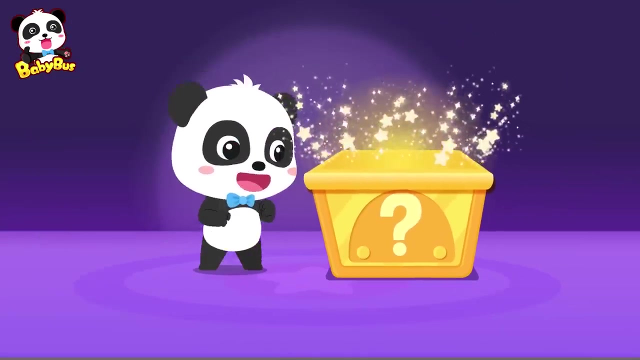 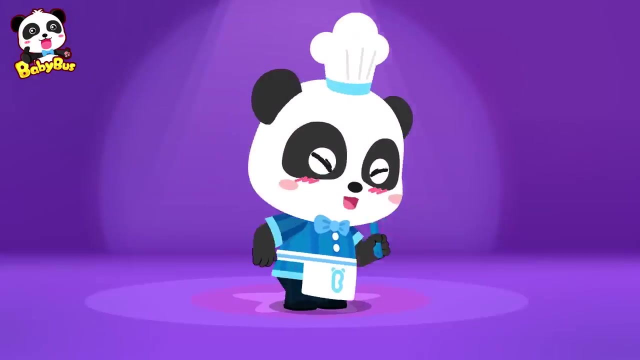 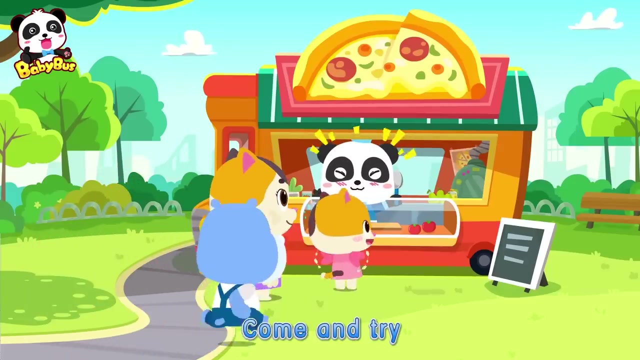 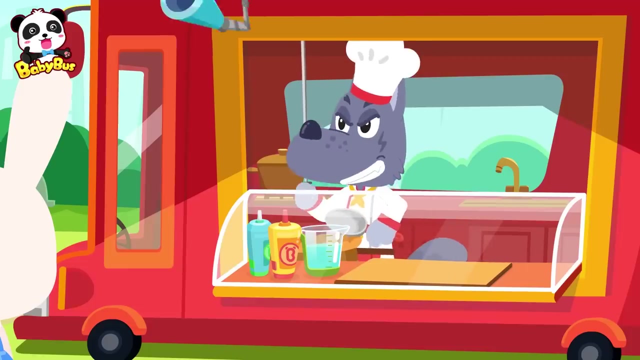 Rice balls, Kiki, let's share. Wow, Sweet rice balls, Yay, Wow, Kids, do you want to have some sweet rice balls? Yeah, Yummy pizza. Come and try Wow. Ah, Come to my pizza truck. 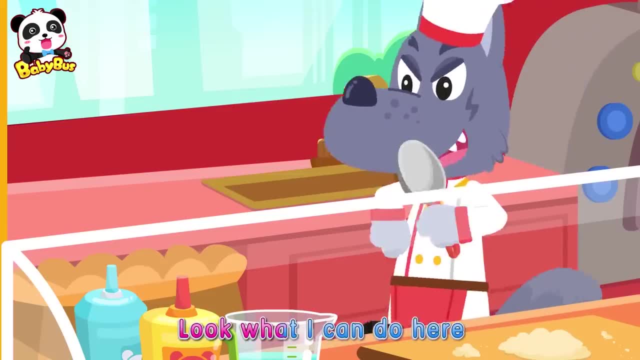 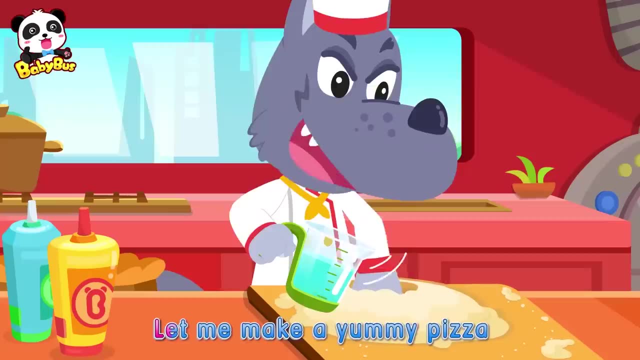 I'm a great pizza chef. Look what I can do here: Making a yummy pizza. Mix, mix, mix, mix the dough. Let me make a yummy pizza. Knead, knead, knead, knead the dough. Let me make a yummy pizza. 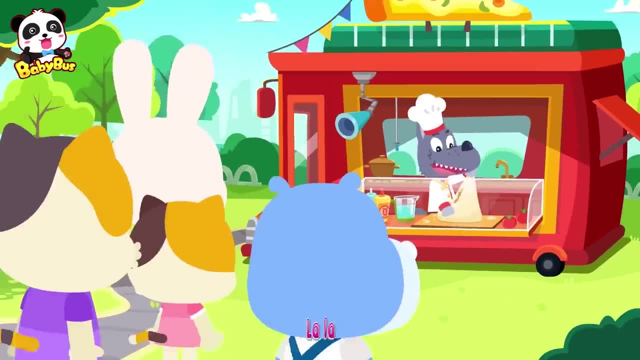 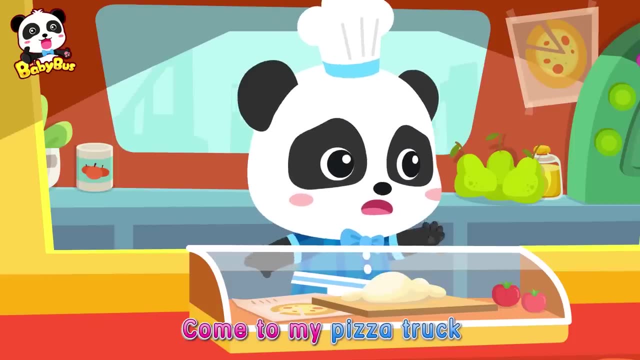 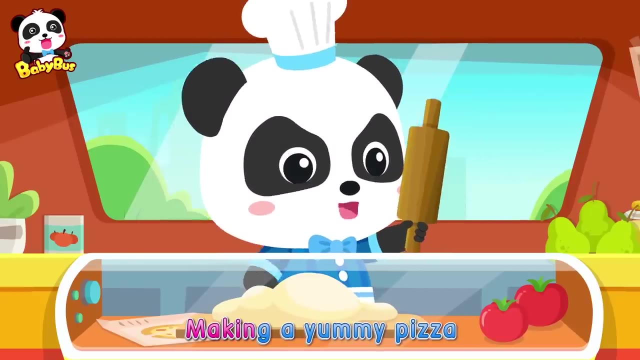 Doo doo, doo la la la, Doo doo, doo, la la. Wow, I want that pizza. Come to my pizza truck. I'm a great pizza chef. Look what I can do here: Making a yummy pizza. 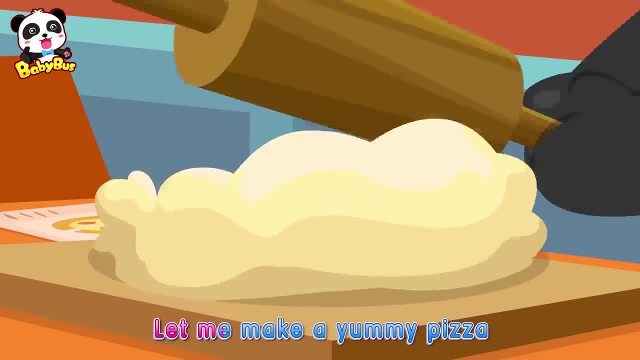 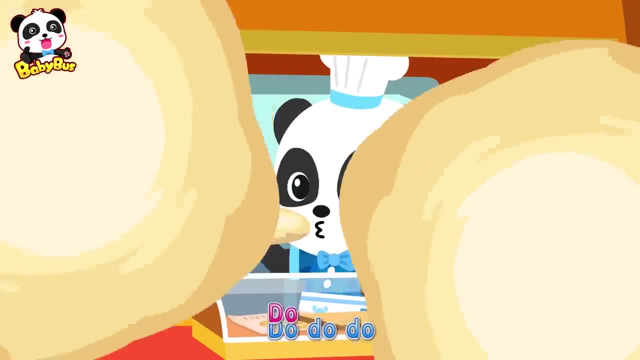 Roll, roll, roll, roll the dough. Let me make a yummy pizza. Toss, toss, toss, toss the dough. Let me make a yummy pizza. Doo doo, doo la la la, Doo, doo, doo la la. 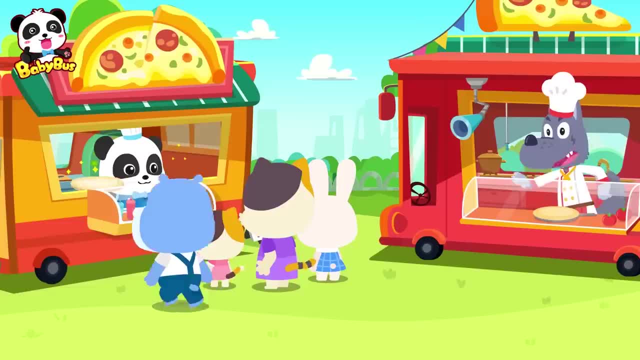 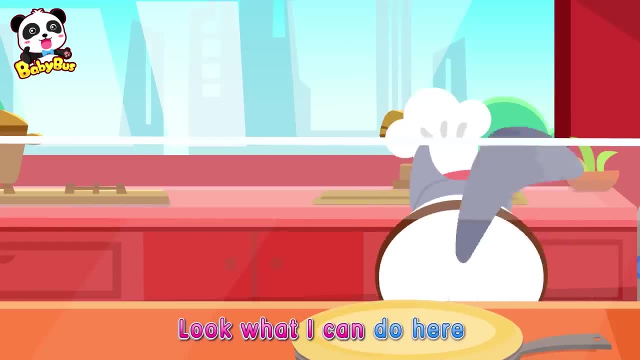 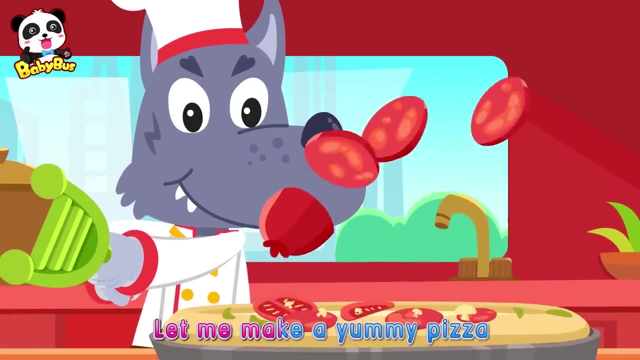 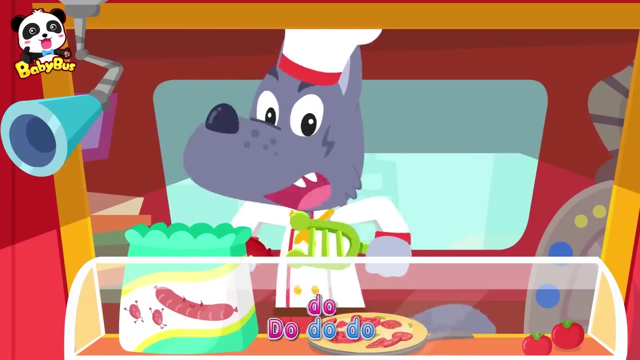 That looks even better. Come to my pizza truck. I'm a great pizza chef. Look what I can do here: Making a yummy pizza. Cut cut up some sausage. Let me make a yummy pizza. Cut, cut up some tomatoes. Let me make a yummy pizza. Doo, doo, doo, la, la, la. 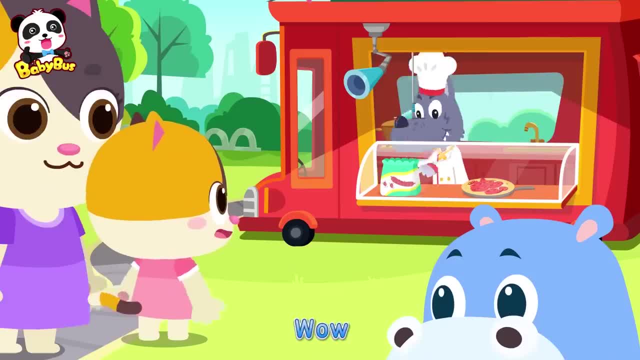 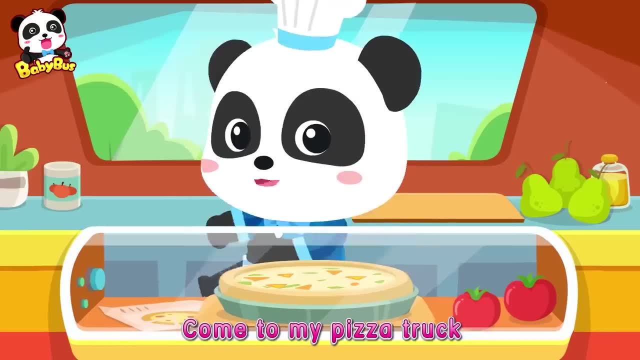 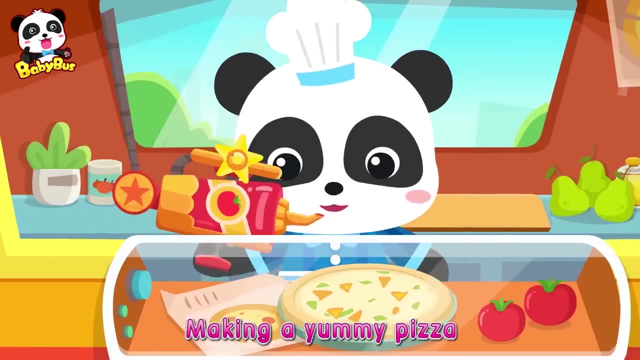 Doo, doo, doo, la la. And then the pizza is ready. for now, Come to my pizza truck. I'm a great pizza chef. Look what I can do here: Making a yummy pizza. Put, put, put some ketchup. Let me make a yummy pizza. 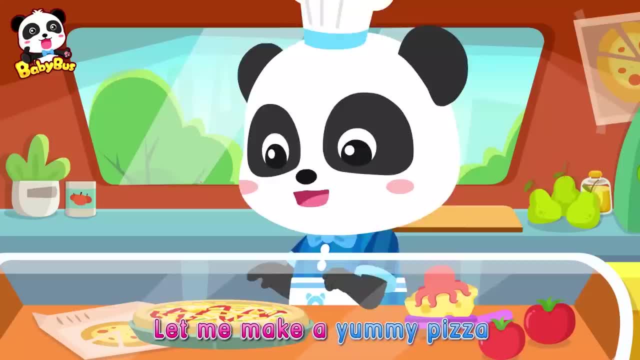 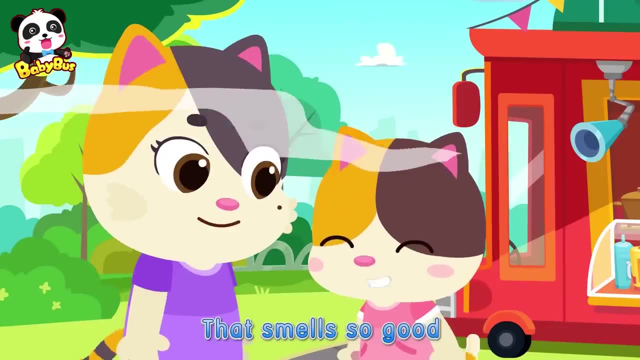 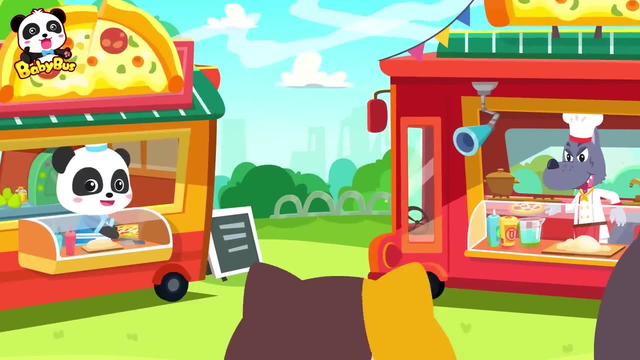 Greet, greet, greet. some cheese. Let me make a yummy pizza. Doo doo doo la la la Doo doo doo la la. Mom, that smells so good. Which one should I buy? 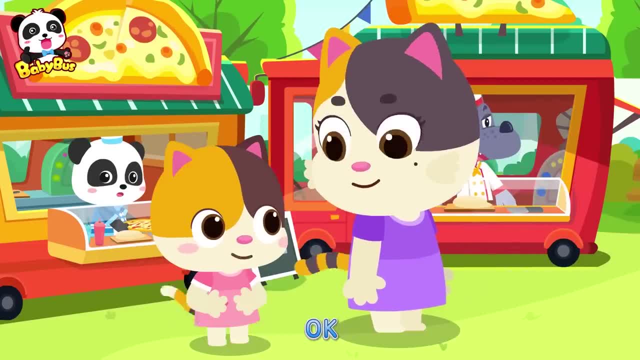 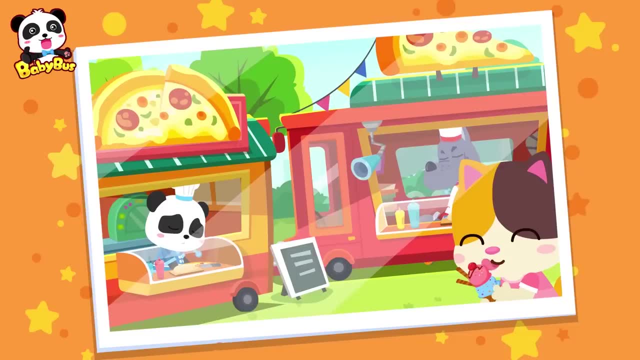 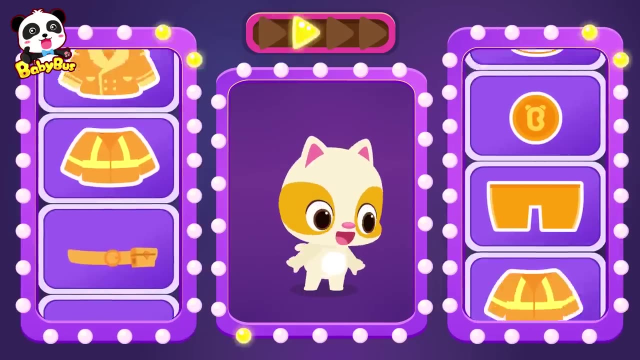 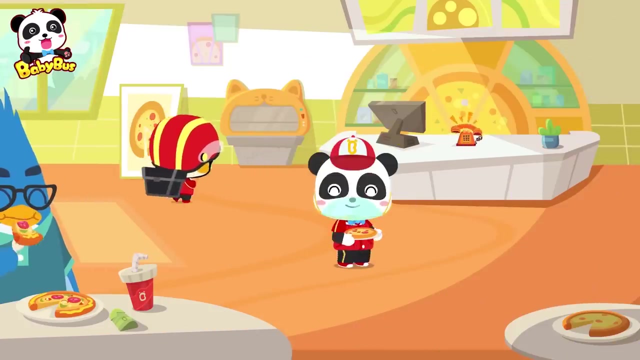 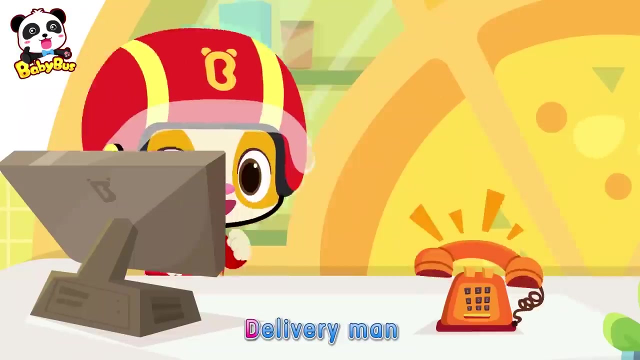 Mom, Ice cream. I want to eat ice cream. Wow Yeah, Timmy, The phone is ringing, Pick it up and take the order. Okay, Oh, delivery man Picking up the phone. Just a moment, sir. 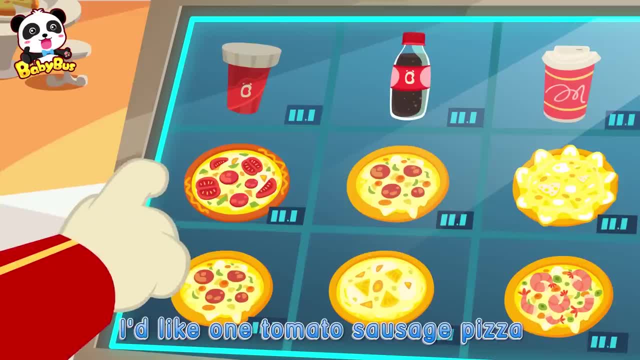 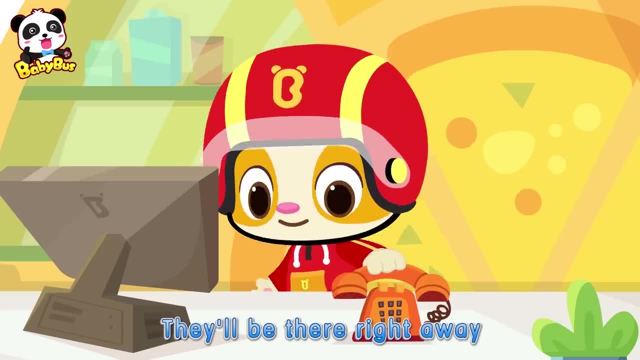 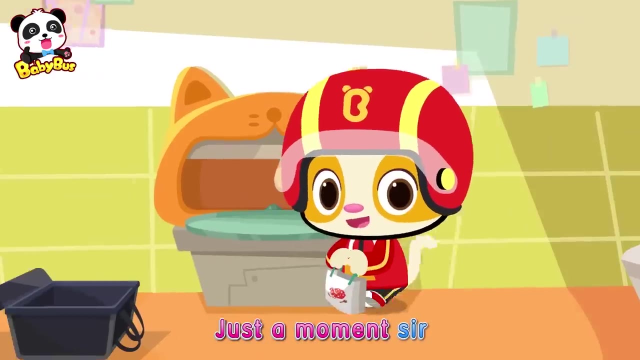 What would you like? I'd like one tomato sausage pizza, one cheese pizza and one cola. Okay, They'll be there right away. Oh, delivery man Putting the food in a bag. Just a moment, sir. I'm on my way. 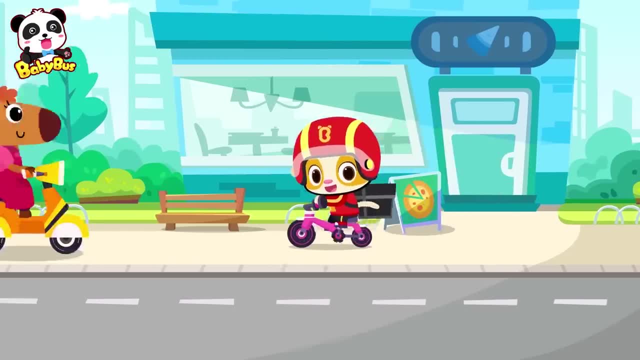 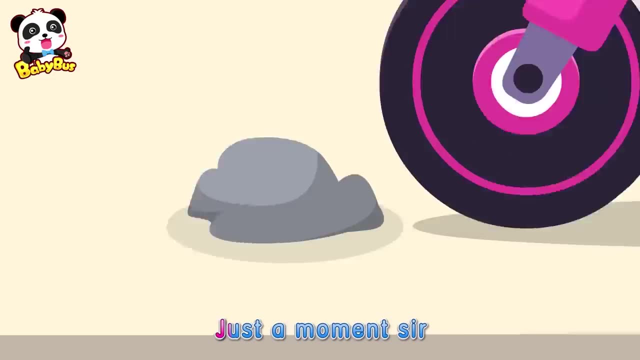 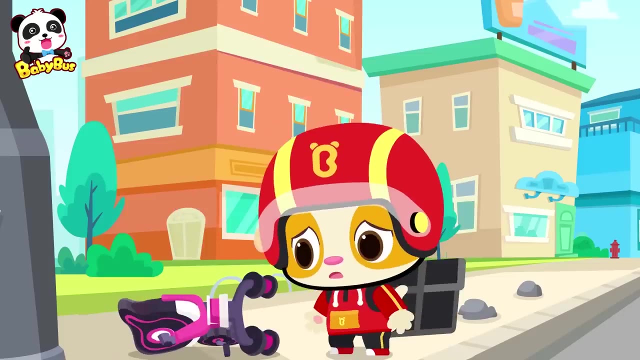 The food is all ready, Let's go. Oh delivery man Delivering food. Just a moment, sir, I'll be right there. Yeah, My bike is broken. What should I do? Oh delivery man Delivering food. 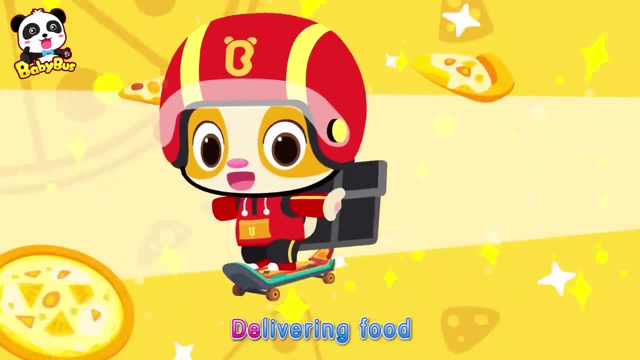 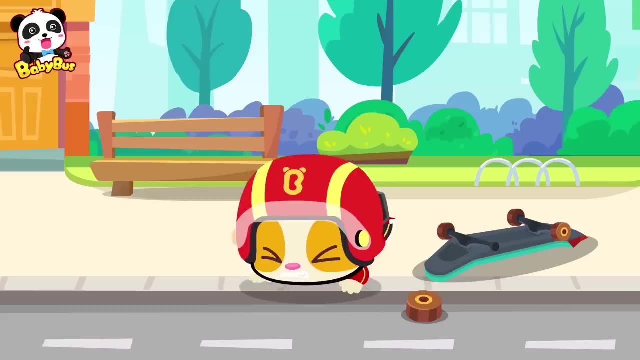 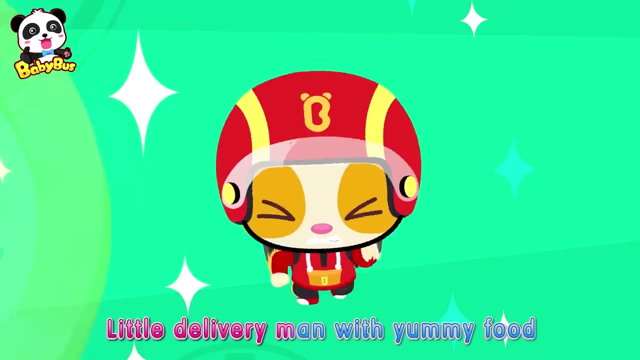 Just a moment, sir. I'll be right here soon. Ouch, Oh no, It's broken too. I have no time. What should I do? Little delivery man With yummy food. Little delivery man Delivering food. 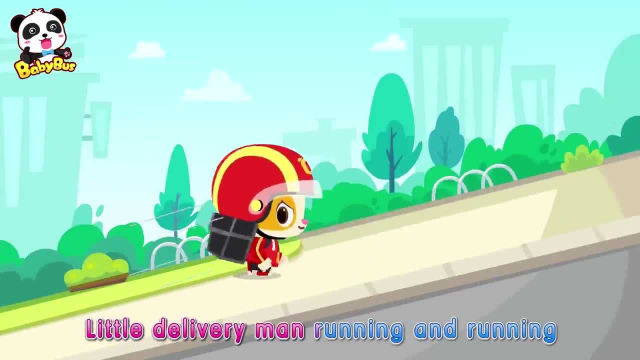 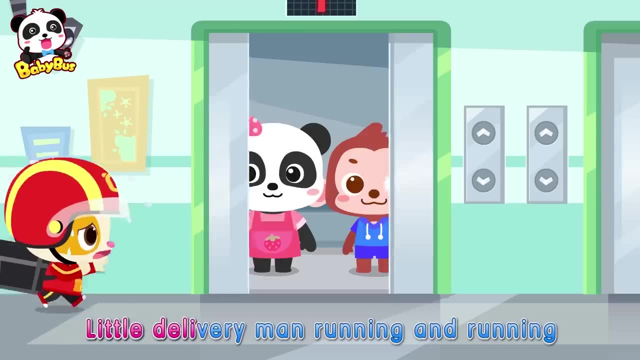 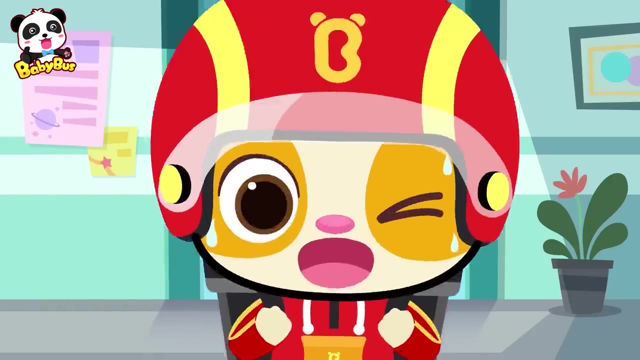 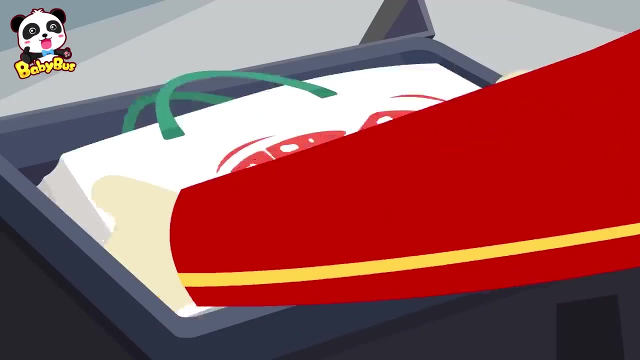 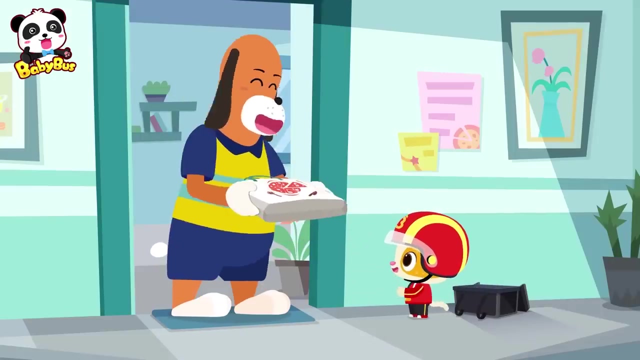 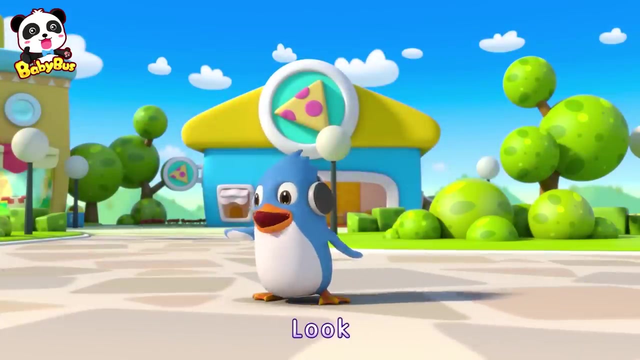 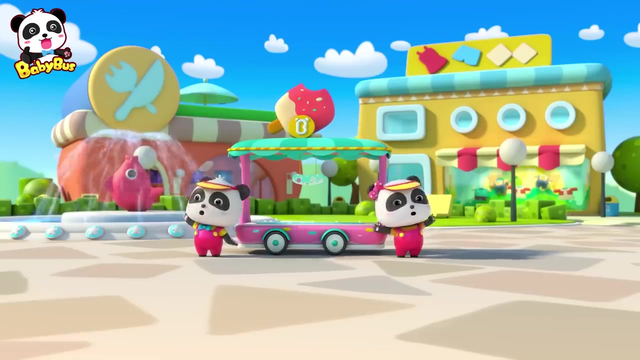 Little Delivery Man Running and Running. Little Delivery Man with yummy food. Little Delivery Man Running and Running. Oh, he made it. Here's the food you ordered. Wow, Thank you. Wow, Look, it's an ice cream truck. Oh, I like milk flavored ice cream best. 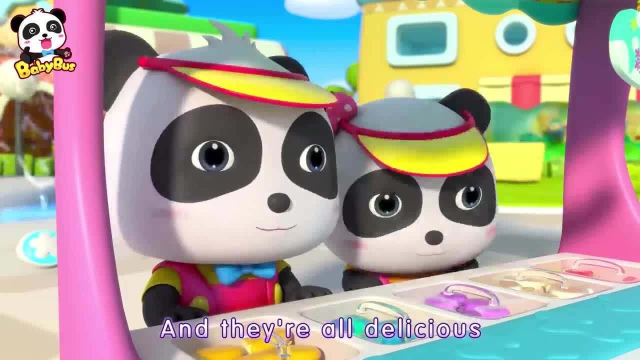 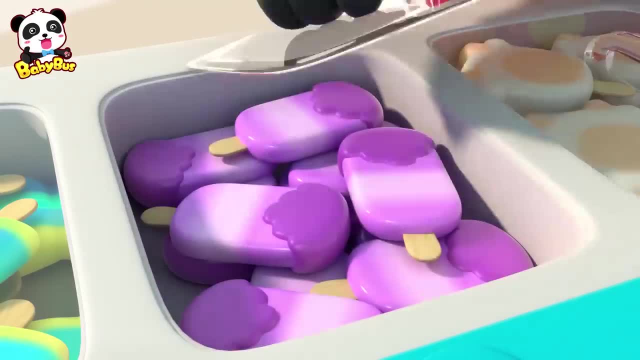 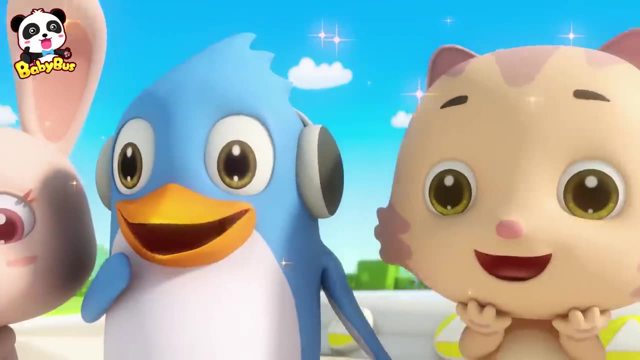 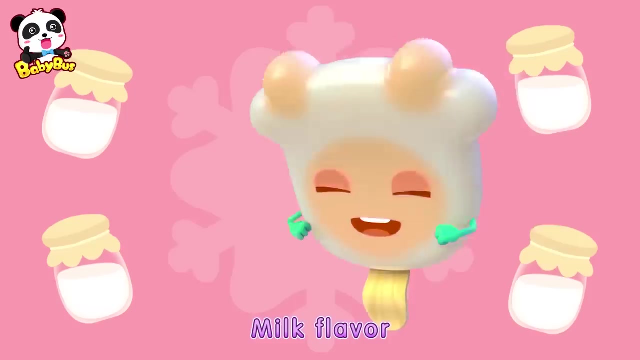 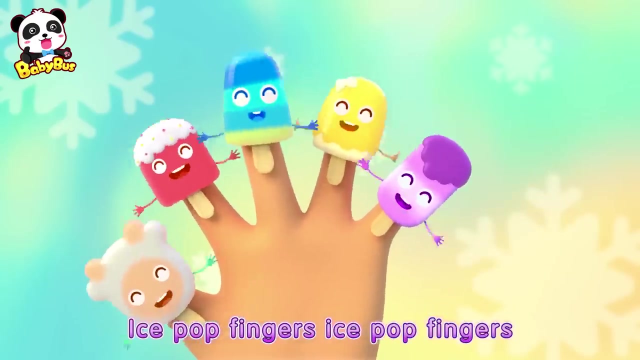 There are many other flavors here and they're all delicious. Do you guys want to try them? Sure, Ice Pop Fingers. Ice Pop Fingers. This one is white Milk flavor, Milk flavor, It's so tasty. Ice Pop Fingers. Ice Pop Fingers- This one is red. 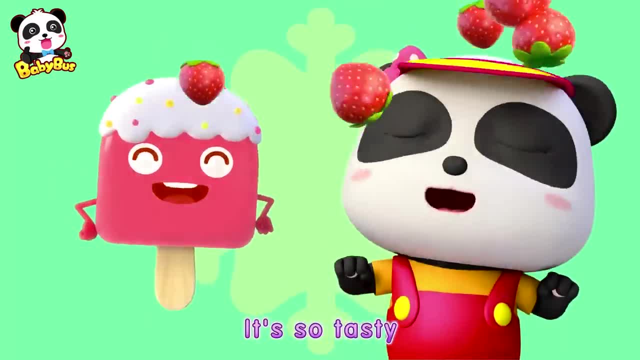 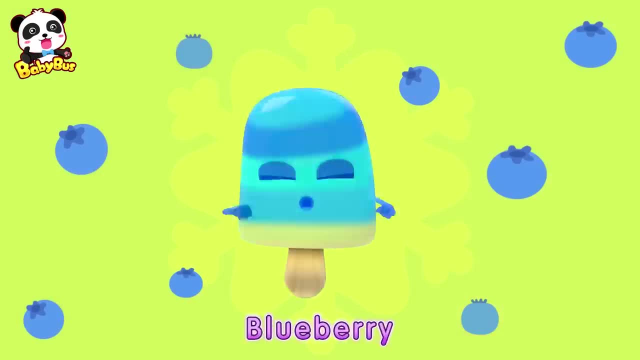 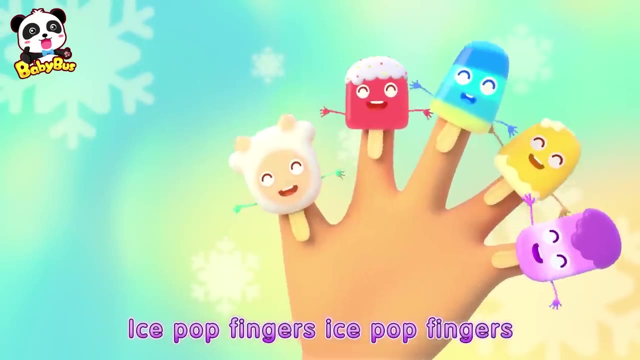 Strawberry, Strawberry, It's so tasty. Ice Pop Fingers, Ice Pop Fingers. This one is blue Blueberry, Blueberry, It's so tasty. Ice Pop Fingers. Ice Pop Fingers. This one is yellow Banana flavor- Banana flavor, It's so tasty. 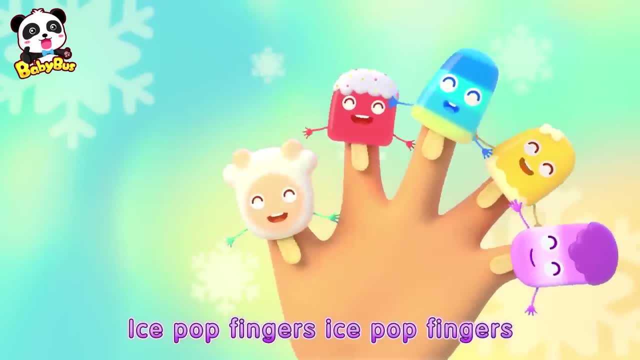 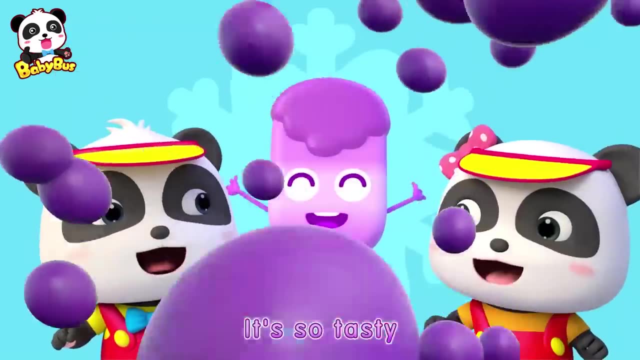 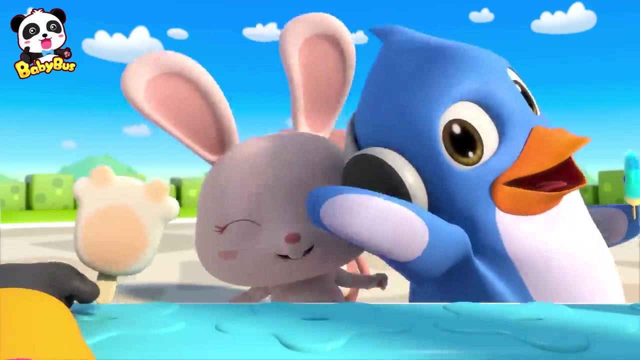 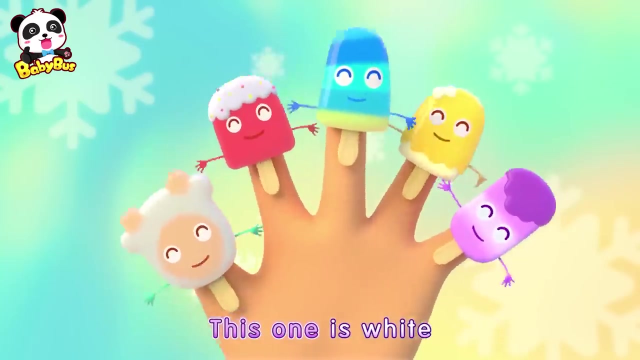 Ice Pop Fingers. Ice Pop Fingers. This one is purple Grape flavor. Grape flavor, It's so tasty. It's so tasty. Ice pop fingers. ice pop fingers. this one is white Milk flavor. milk flavor, it's so tasty. 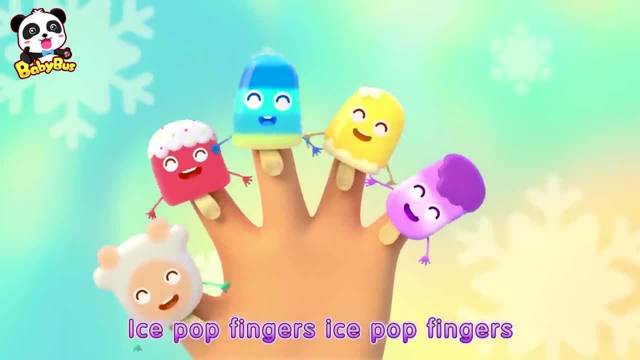 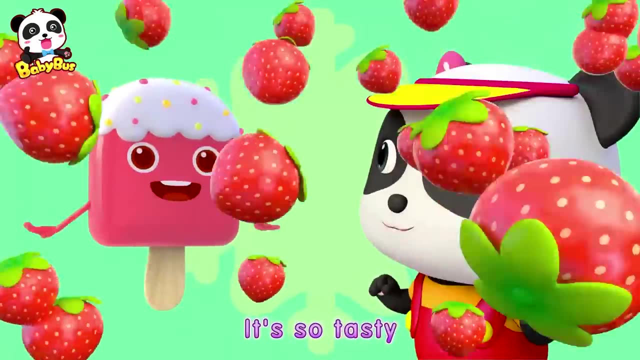 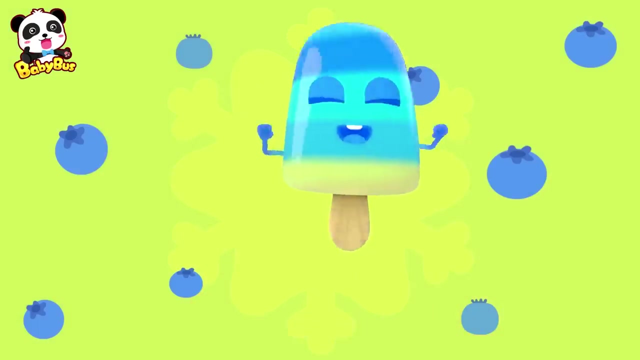 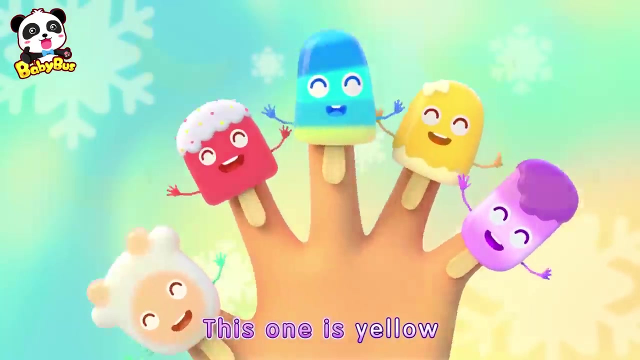 Ice pop fingers, ice pop fingers. this one is red, Strawberry, strawberry, it's so tasty. Ice pop fingers, ice pop fingers. this one is blue, Blueberry, blueberry, it's so tasty. Ice pop fingers, ice pop fingers. this one is yellow. 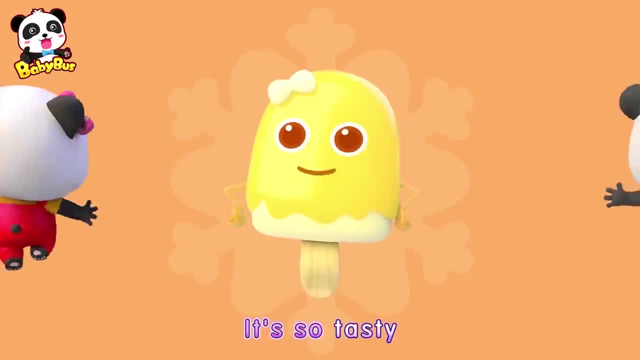 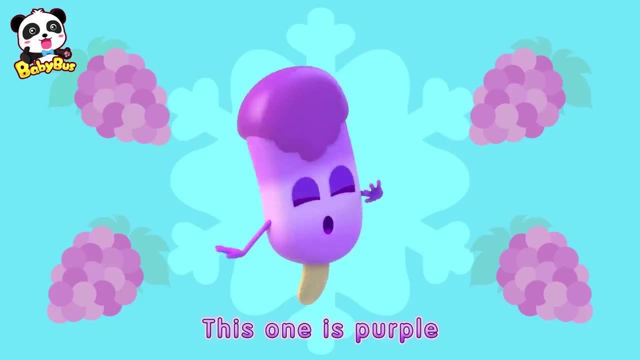 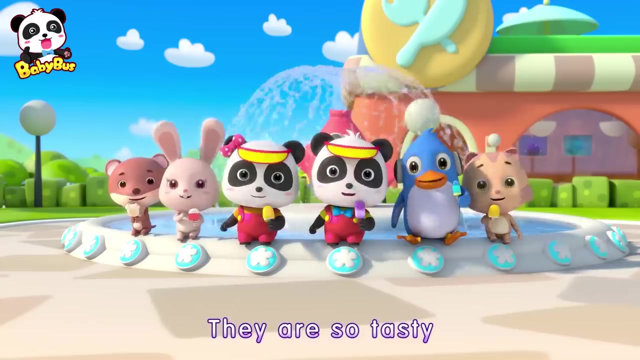 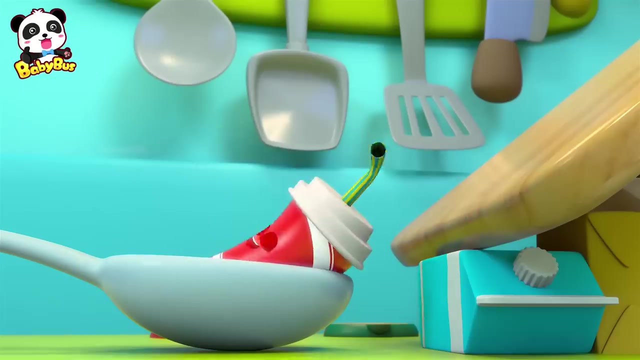 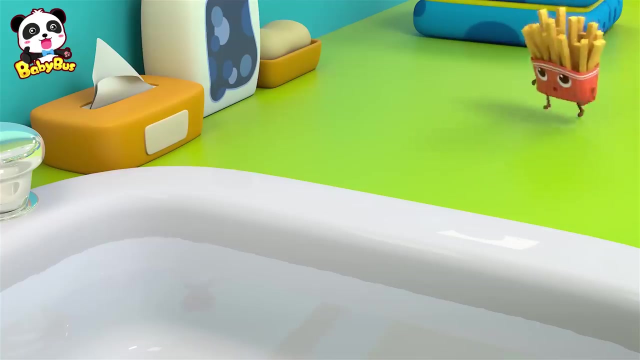 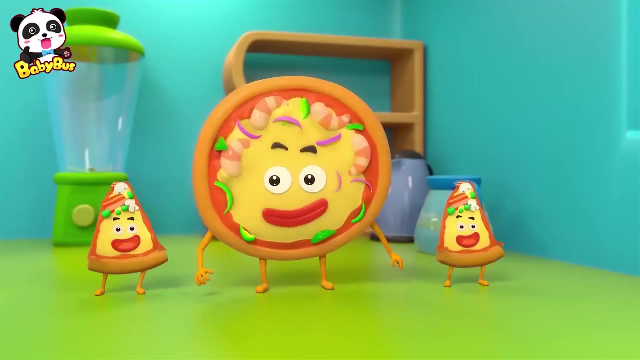 Banana flavor, banana flavor, it's so tasty. Ice pop fingers- ice pop fingers- this one is purple. Great flavor, Great flavor. It's so tasty. They are so tasty. This is so much fun. Yeah, Wow, This looks like a really fun place. We'll take it. 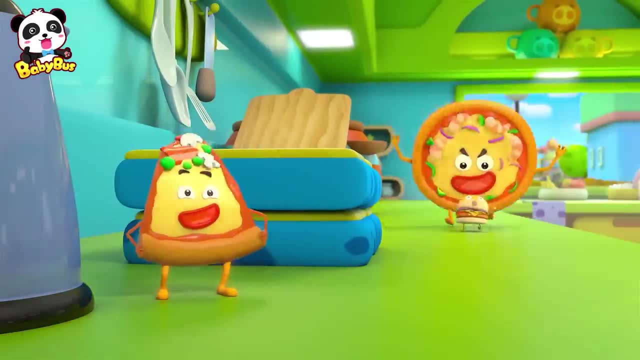 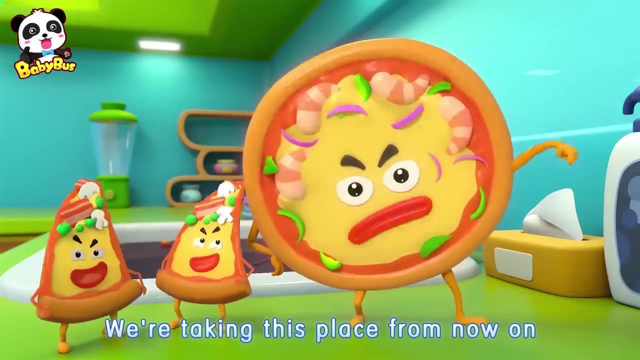 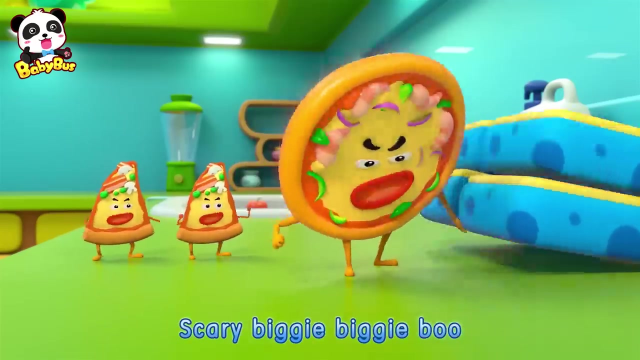 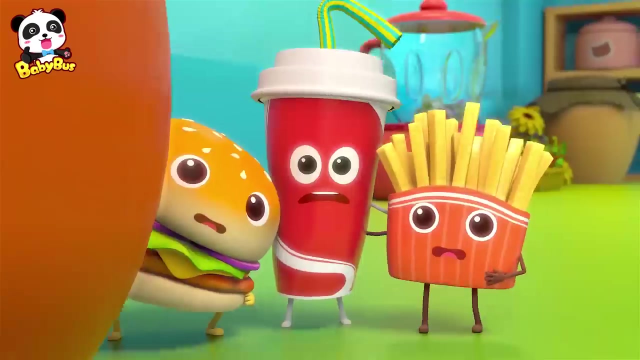 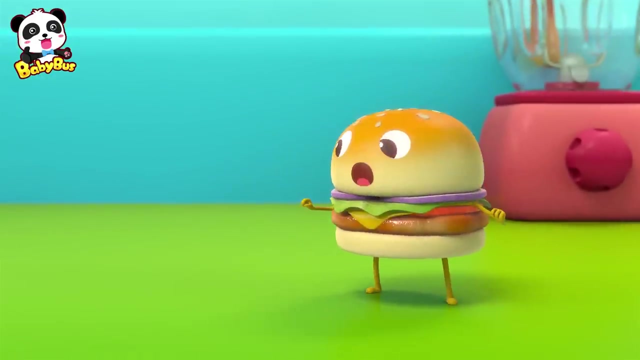 No, We're taking this place from now on. We're taking this place from now on. Scary Biggie, Biggie Boo. Scary Biggie, Biggie Boo. That pizza's here to mess around. Clever Burger says: what should I do? 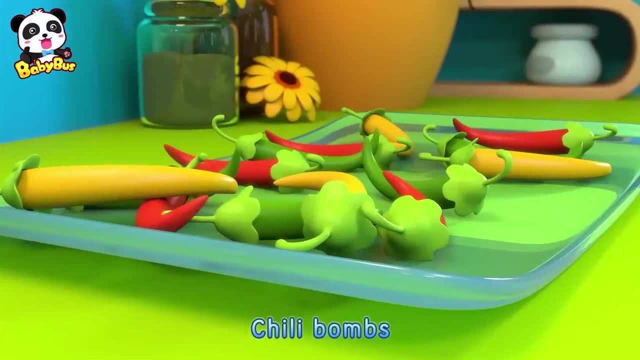 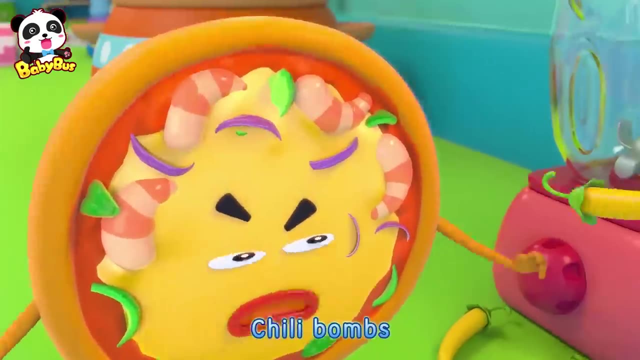 Let's see what he found out. Chili Bombs- Yippee, yippee, come on, Brave Burger. Chili Bombs- Boo, Yippee, yippee, come on, Brave Burger. Scary Biggie, Biggie Boo. 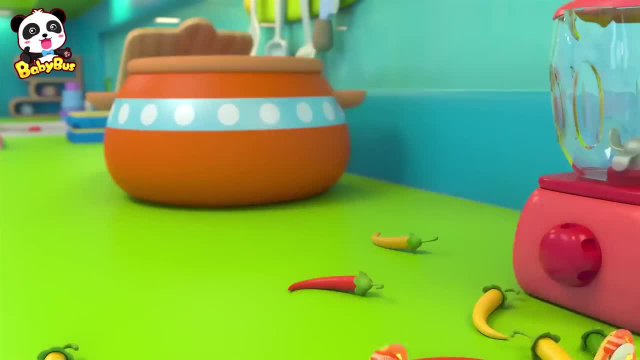 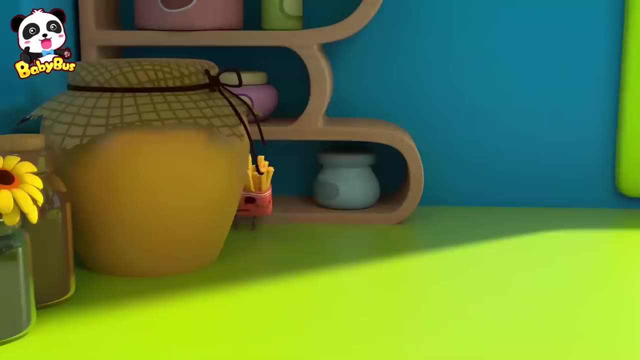 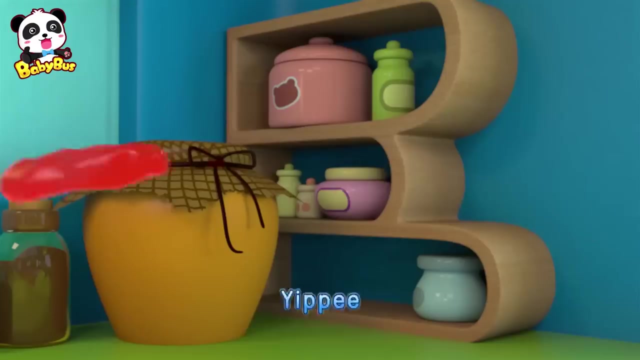 Scary Biggie, Biggie Boo. That pizza's here to mess around. Clever French Fries says: what should I do? Let's see what he found out: Ketchup Bombs. Yippee, yippee, come on. 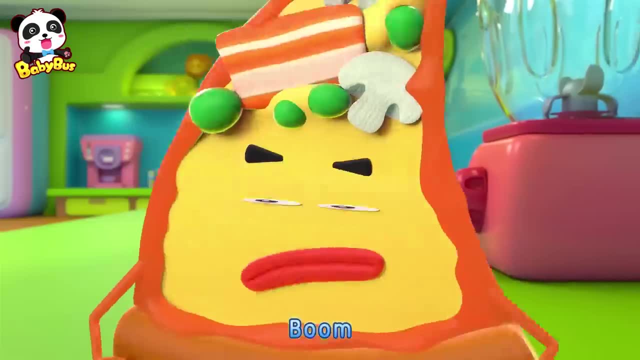 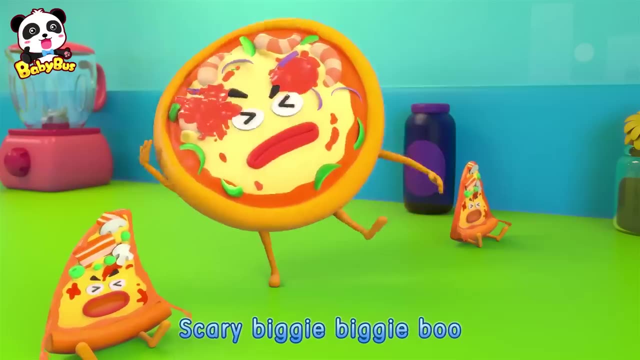 Brave French Fries. Ketchup Bombs, Ketchup, Bombs Boo, Ketchup, Bombs Boo, Yippee, yippee. come on, Brave French Fries. Scary, Biggie, Biggie Boo, Scary, Biggie, Biggie Boo. 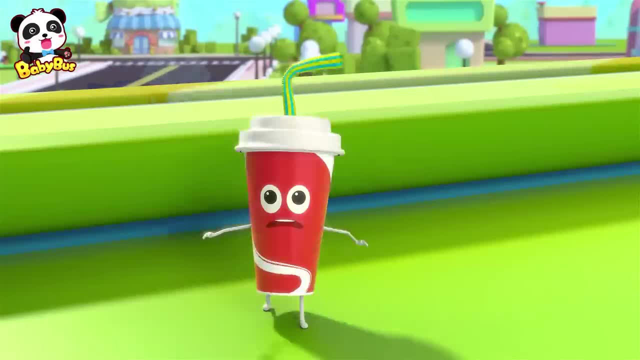 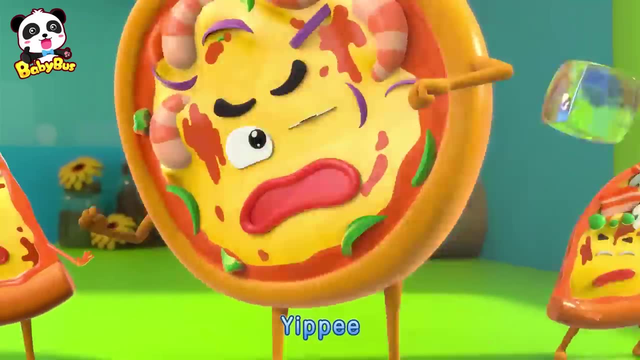 That pizza's here to mess around. Clever Cola says: what should I do? Let's see what he found out: Ice Cube Bombs. Yippee, yippee, come on, Brave Cola, Ice Cube Bombs. 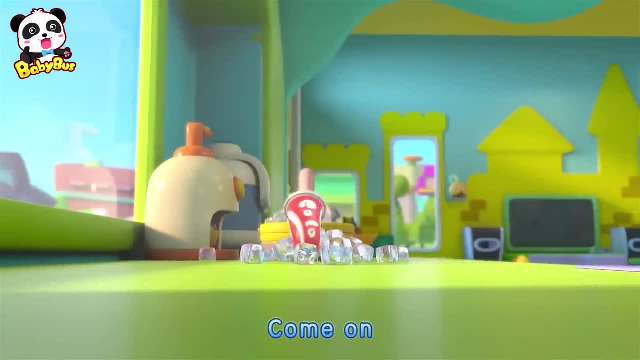 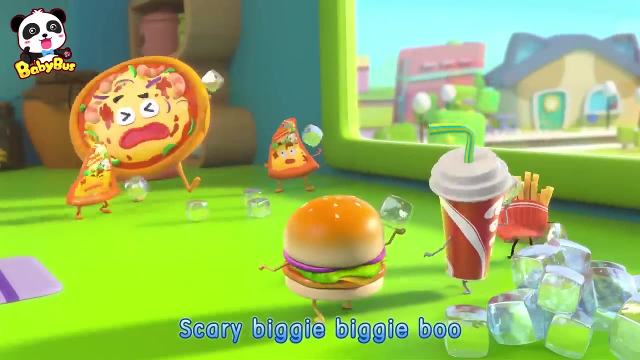 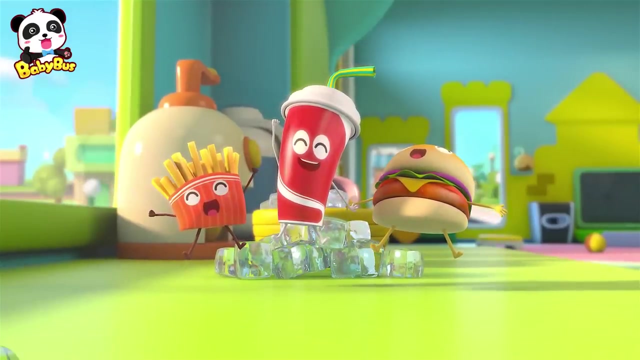 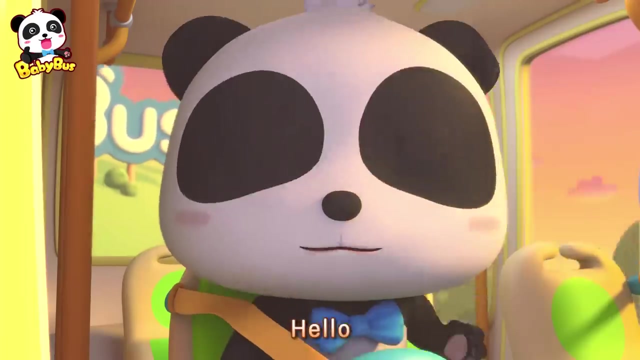 Boom, Ice Cube Bombs, Boom, Yippee, yippee, come on, Brave Cola. Scary Biggie, Biggie Boo. Scary, Biggie, Biggie Boo Boo. Yeah, Hello, I'm Kiki, I'm Mew Mew. 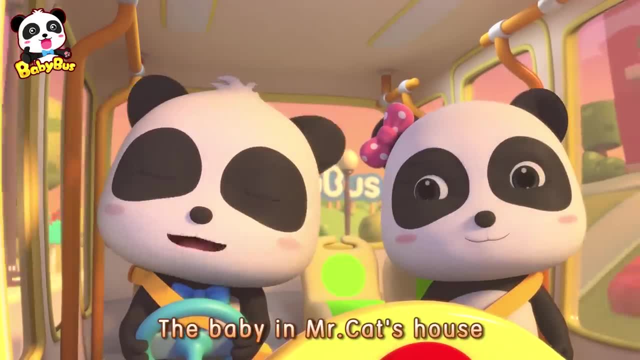 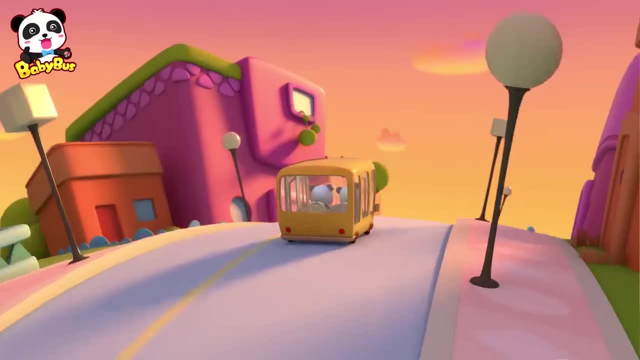 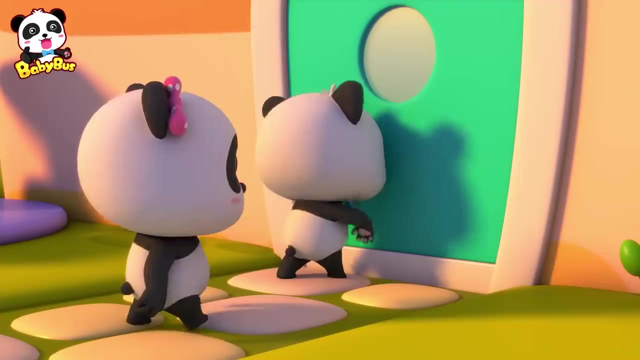 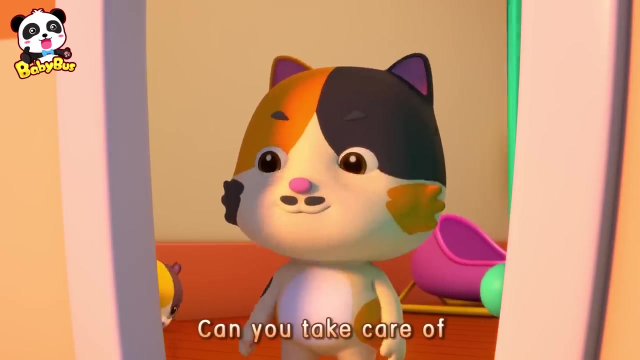 Today we're going to take care of a baby in Mr Cat's house. Let's go together. Hi Kiki Mew Mew. Hello, Mr Cat, Can you take care of my baby today? Sure, No problem. 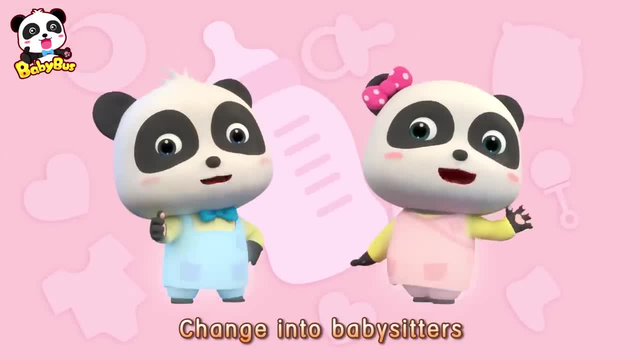 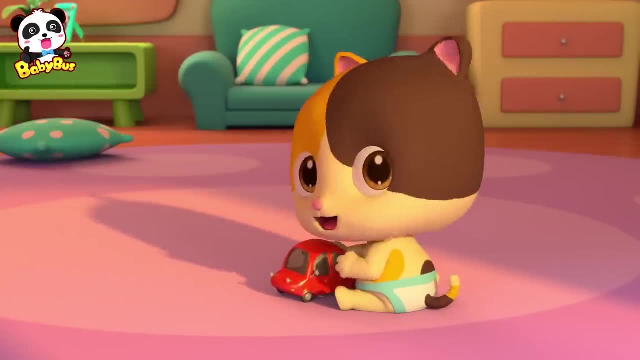 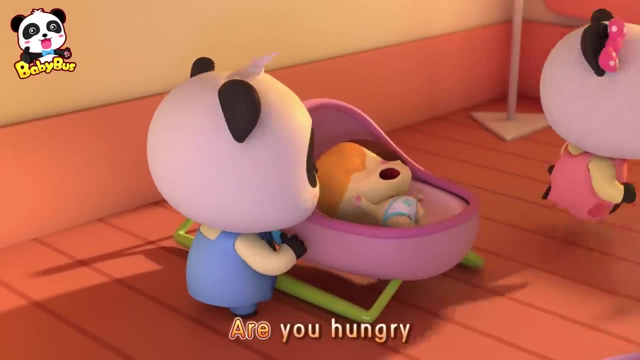 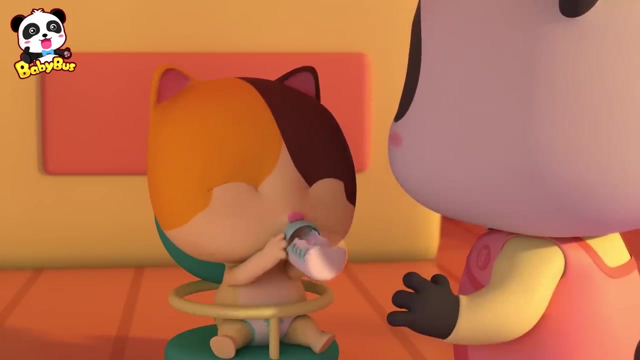 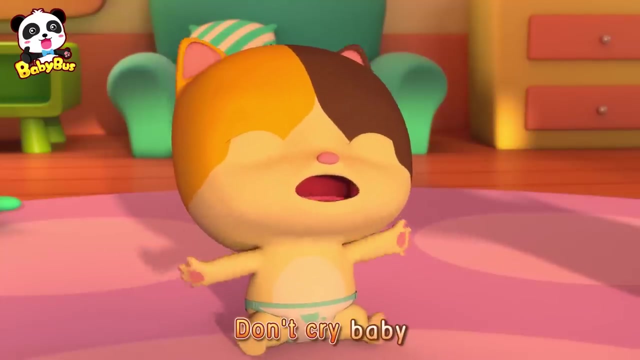 Baby Buds change into babysitters. I'm ready to take care of the baby. Don't cry baby, Are you hungry? Here's a bottle of milk, milk, milk, Lovely baby, my sweetie. Don't cry baby, Are you bored? 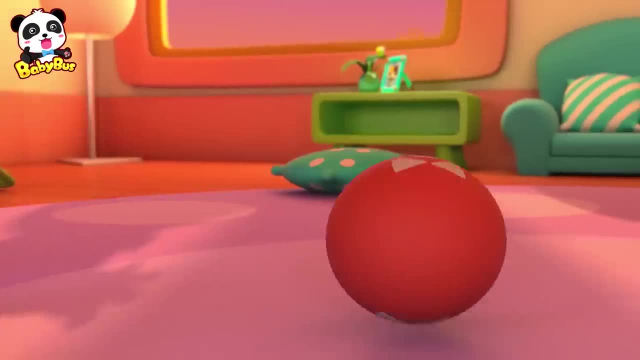 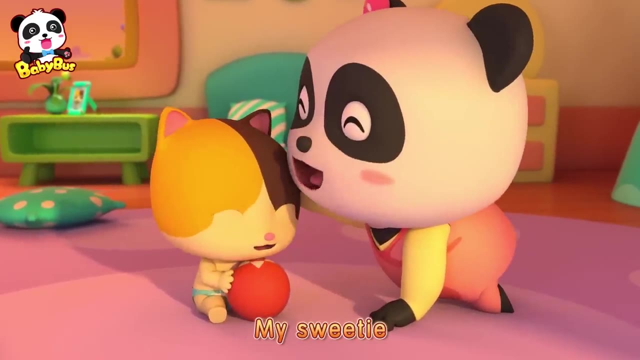 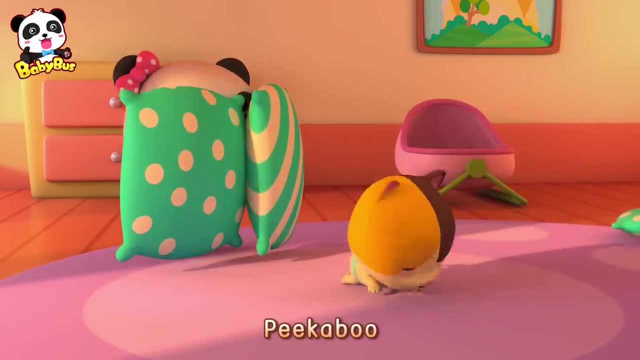 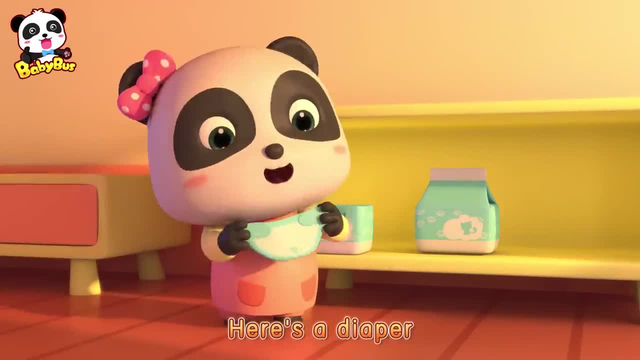 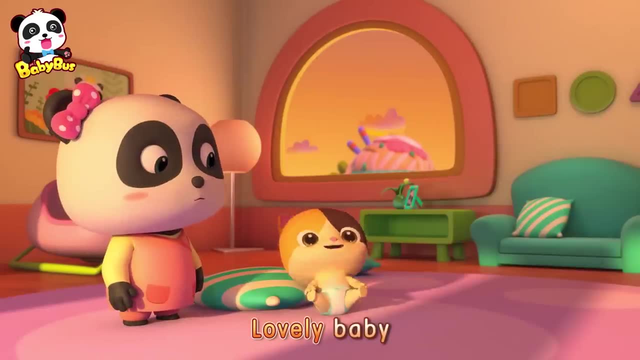 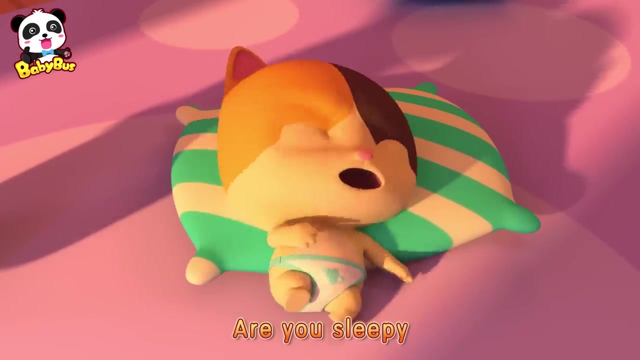 Peek-a-boo, Peek-a-boo, Did you have a pee? Here's a diaper, soft, soft, soft. Lovely baby, my sweetie, Don't cry, baby, Are you sleepy? Here's a cradle nighty-nighty-night. 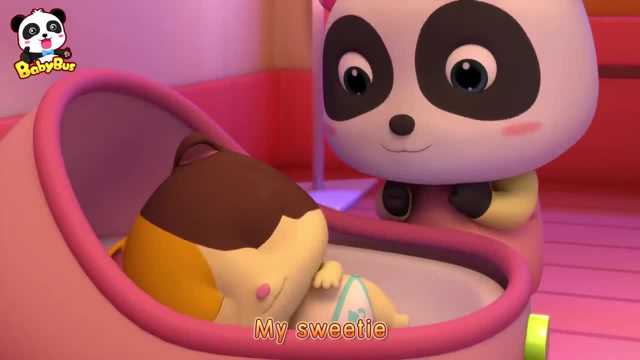 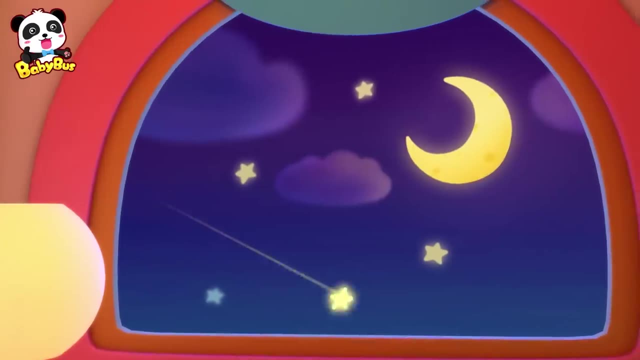 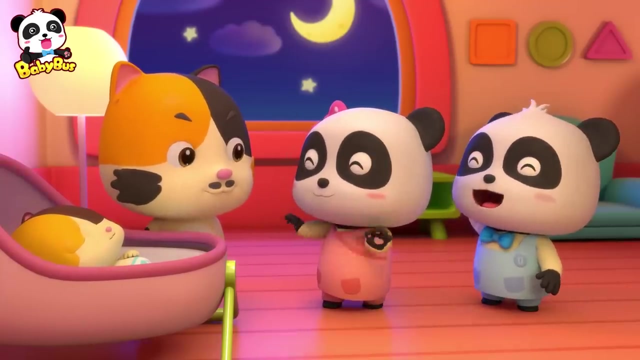 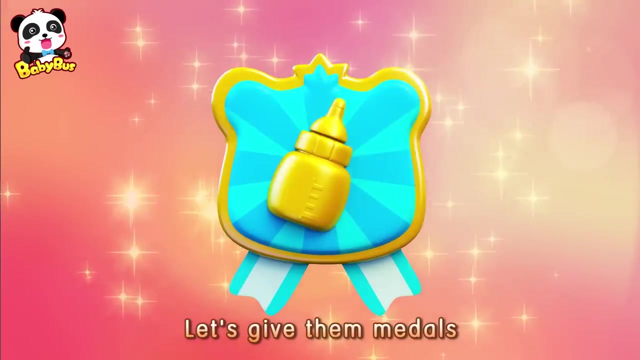 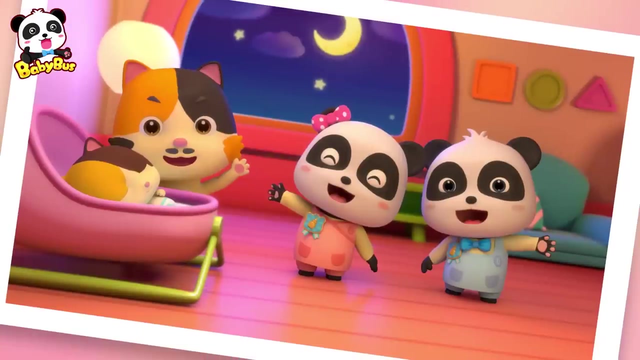 Lovely baby, Baby, my sweeetie. Wow, Thank you guys. You're welcome Today, Kiki and Miu. Miu helped Mr Cat take care of his baby. Let's give them medals. Wow, These candies are awesome, Yummy-yummy. 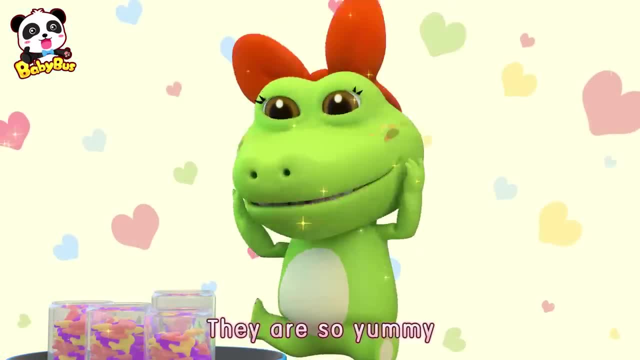 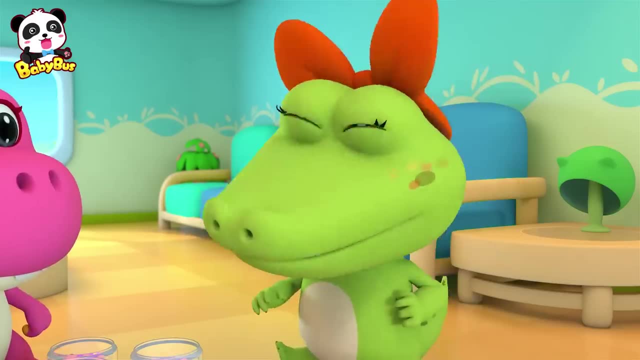 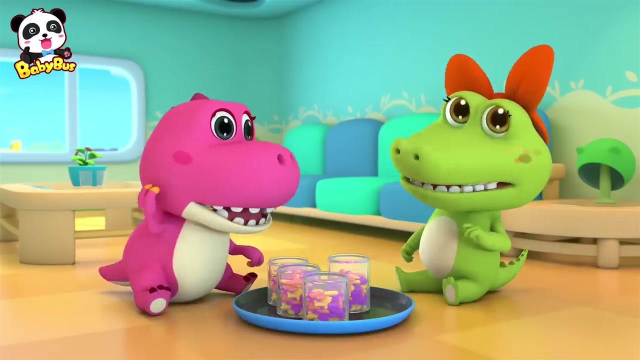 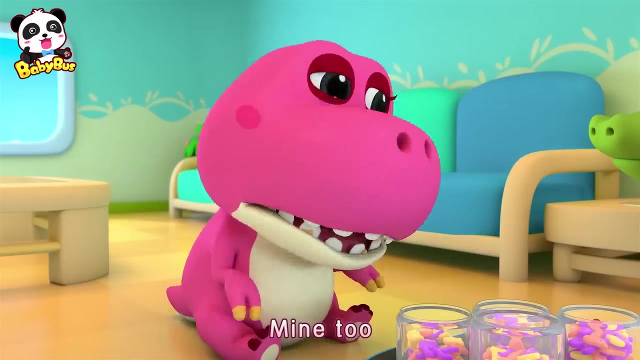 Wow, They are so yummy. This one is my favorite. Try it, Okay. So yummy. The candy is stuck in my teeth. Oh no, Oh, mine too. Then let's go brush our teeth. Alright, Let's go. 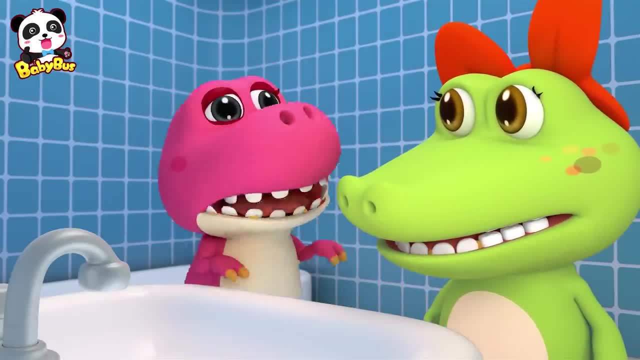 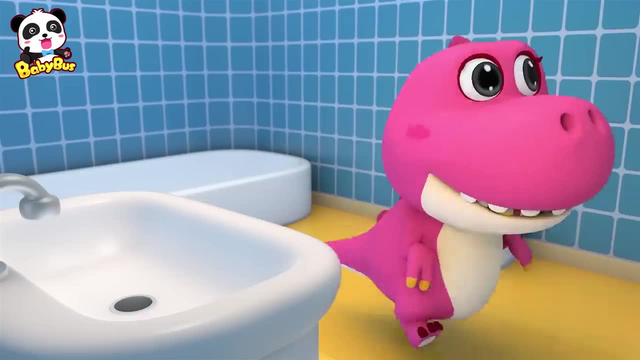 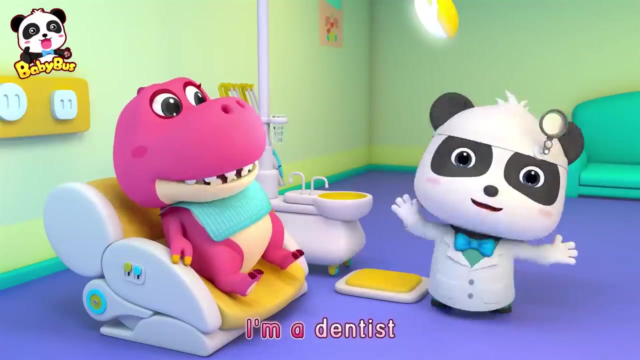 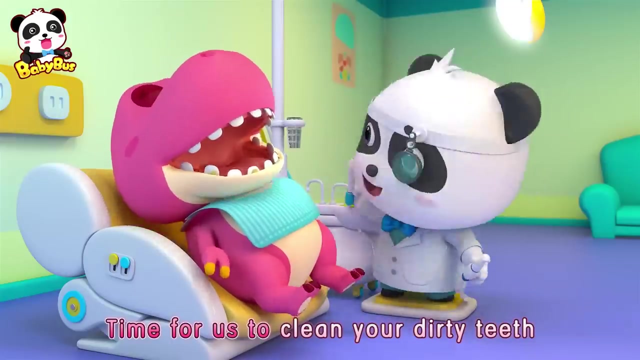 There are still some pieces stuck between my teeth. Aha, Let's go to the little dentist and ask, Ask for help. Okay, I'm a dentist. do-lu-lu, Open your mouth. say, ah, Time for us to clean your dirty teeth. Zoot, zoot, zoot, zoot, shoo, shoo, shoo. 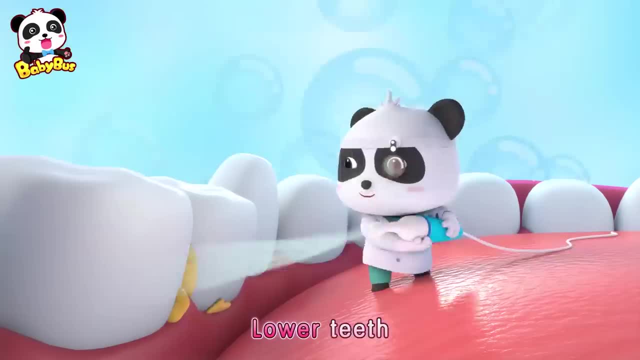 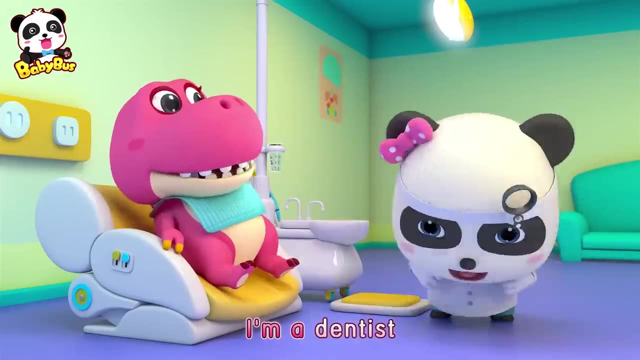 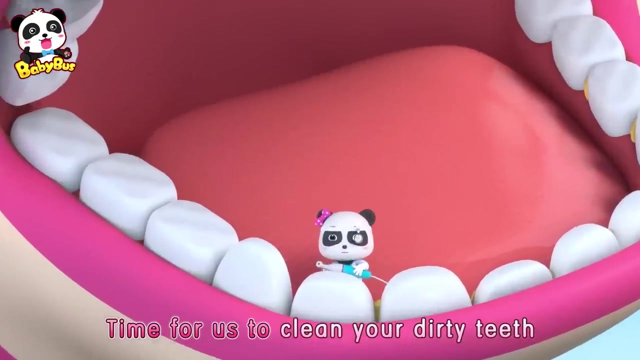 Upper teeth: upper teeth, make them clean. Lower teeth: lower teeth, make them clean. Your teeth are all clean now. I'm a dentist. do-lu-lu, Open your mouth, say, ah, Time for us to clean your dirty teeth. Zoot, zoot, zoot, zoot, shoo, shoo, shoo. 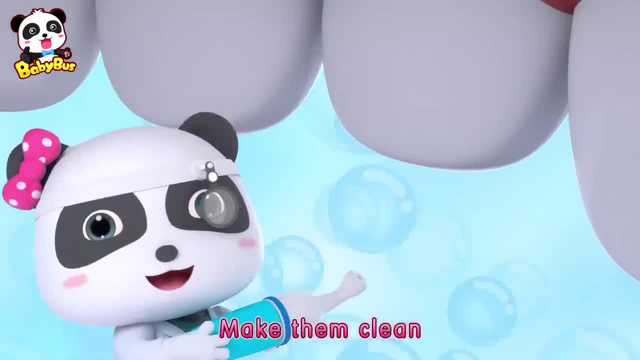 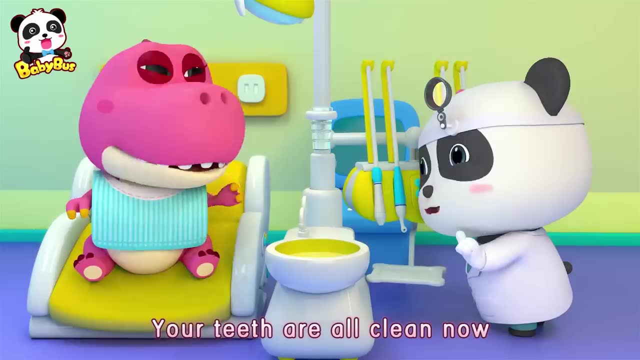 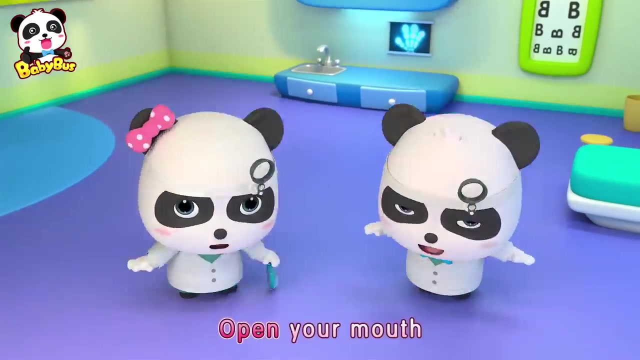 Upper teeth: upper teeth, make them clean. Lower teeth: lower teeth, make them clean. Your teeth are all clean now. I'm a dentist. do-lu-lu, Open your mouth, say ah, I'm a dentist. do-lu-lu, Open your mouth, say ah. 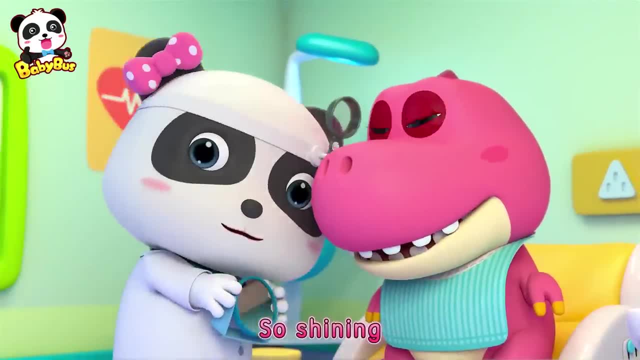 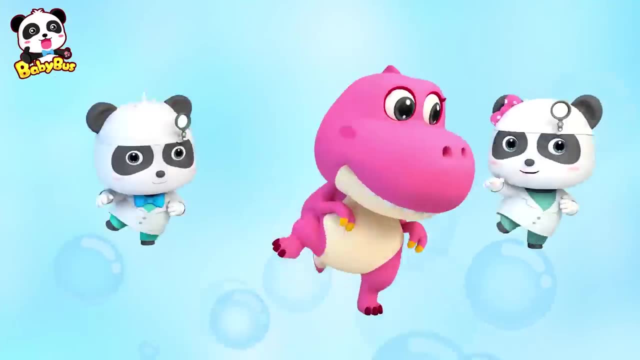 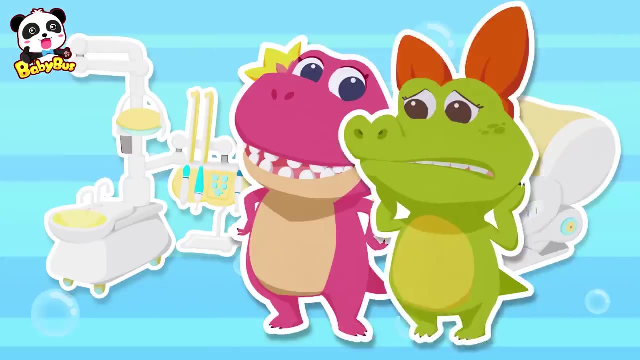 Got clean teeth, yes, So shiny sha-la-la-la, yeah, yeah, Healthy teeth, healthy teeth, let's smile. Healthy teeth, healthy teeth, let's smile Cheese. Thanks, please, I'm a dentist. do-lu-lu, Open your mouth, say ah. 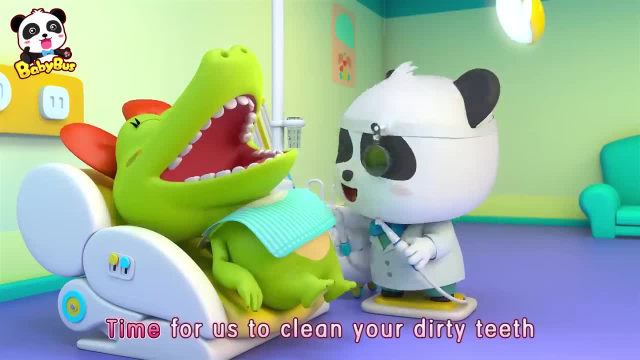 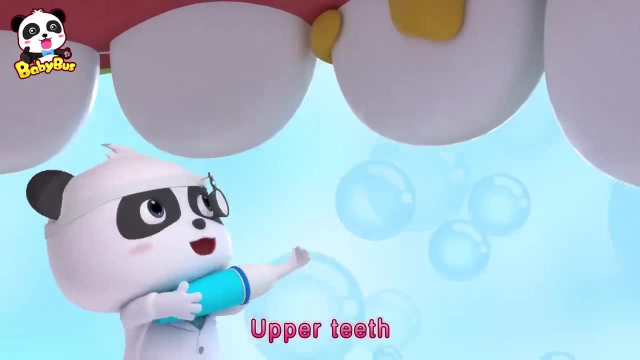 I'm a dentist. do-lu-lu, Open your mouth, say ah, Time for us to clean your dirty teeth. Zoot, zoot, zoot, zoot, shoo, shoo, shoo. Upper teeth, upper teeth, make them clean. Lower teeth: lower teeth, make them clean. 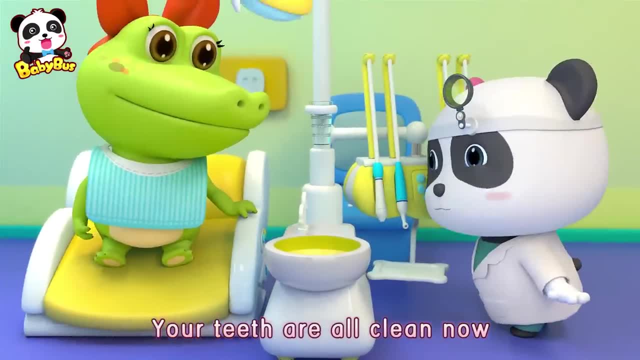 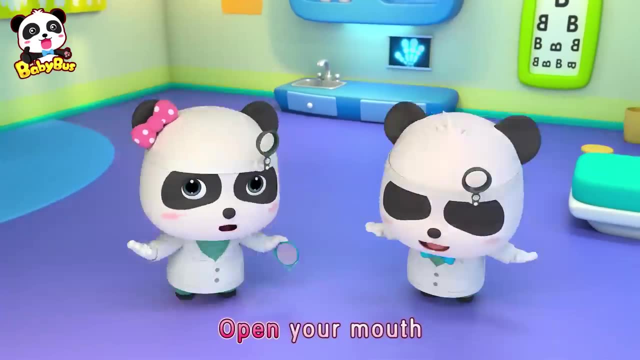 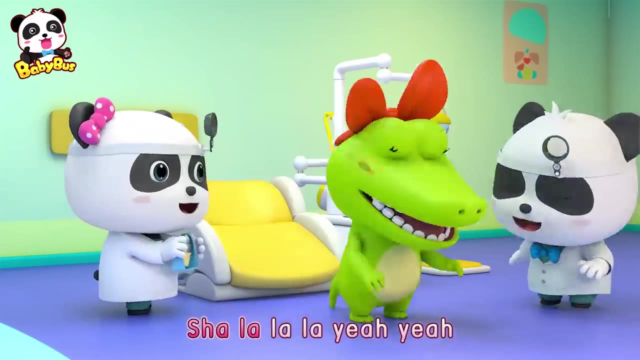 Your teeth are all clean now I'm a dentist. do-lu-lu, Open your mouth, say, ah, Got clean teeth. yes, So shiny sha-la-la-la, yeah, yeah. Healthy teeth, healthy teeth, let's smile. 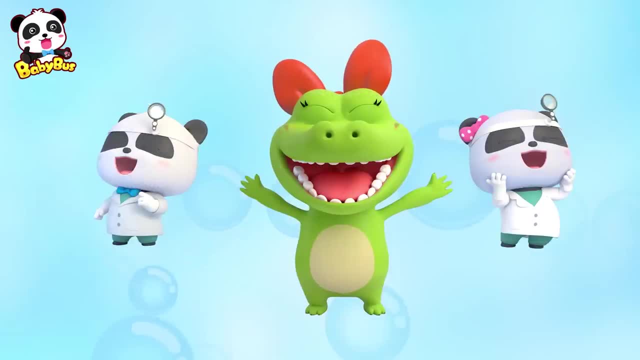 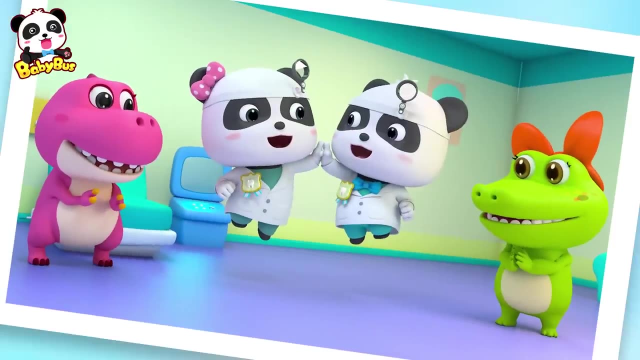 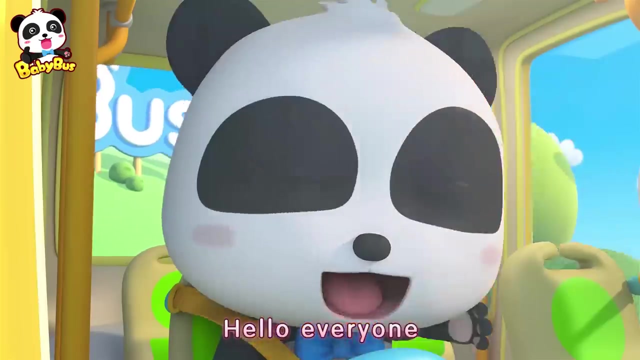 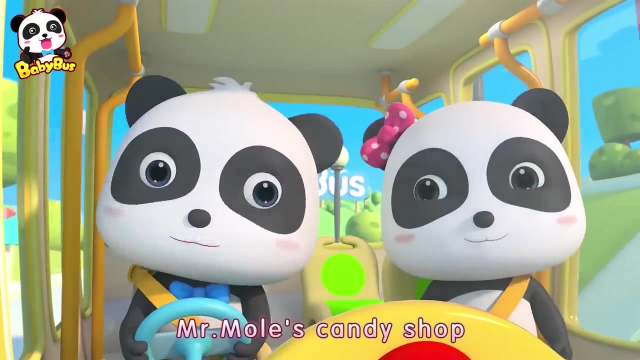 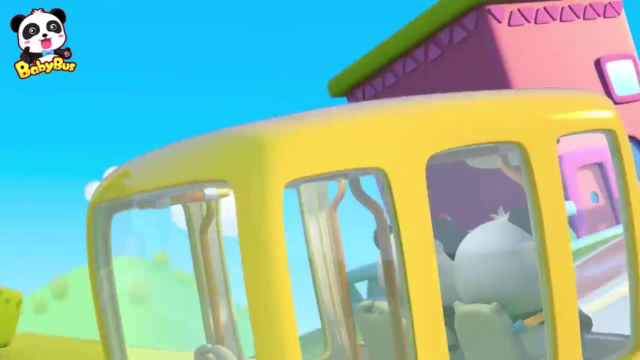 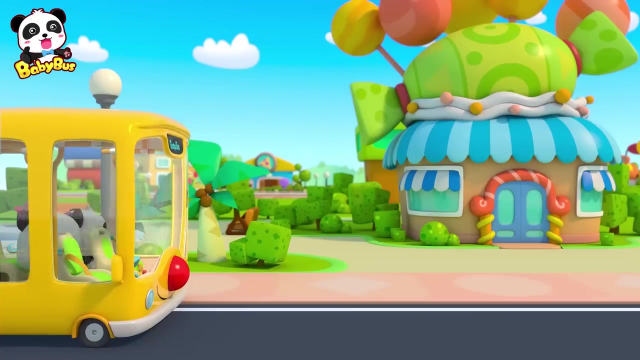 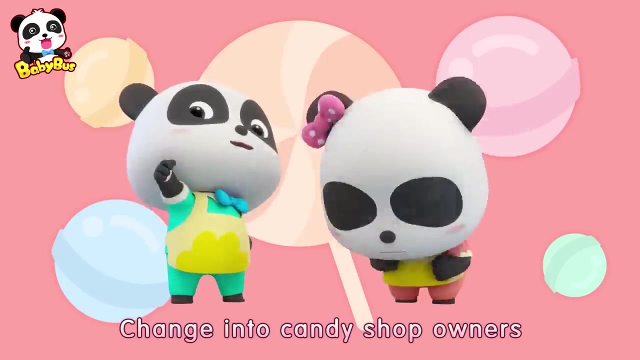 Healthy teeth, healthy teeth, let's smile. Cheese- Yeah, I'm Mew Mew. Today we're gonna visit Mr Mole's candy shop and help him. Wow, It sounds great, Let's go together. Baby Bus change into candy shop owners. 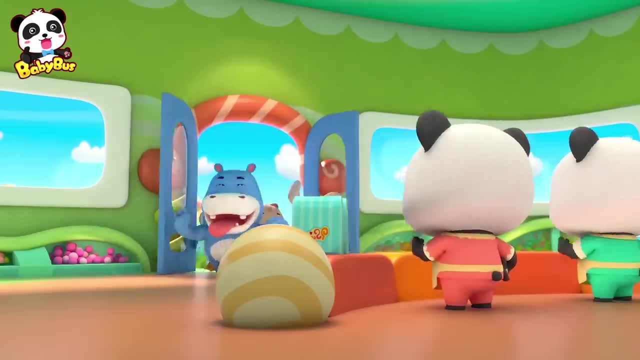 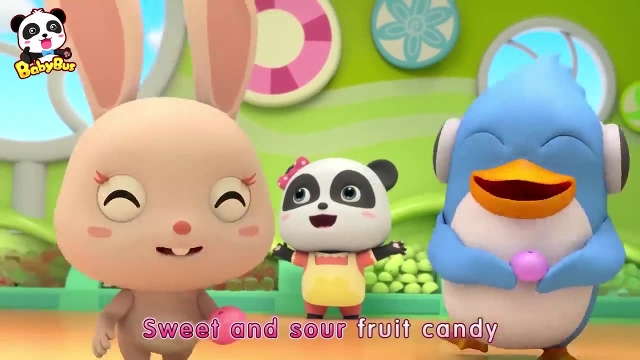 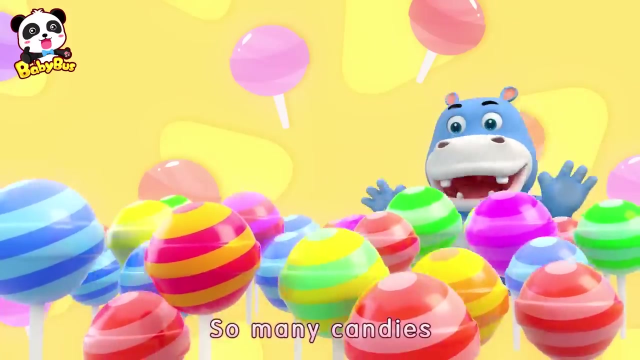 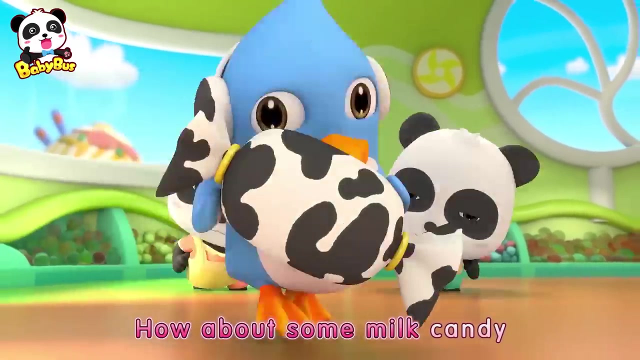 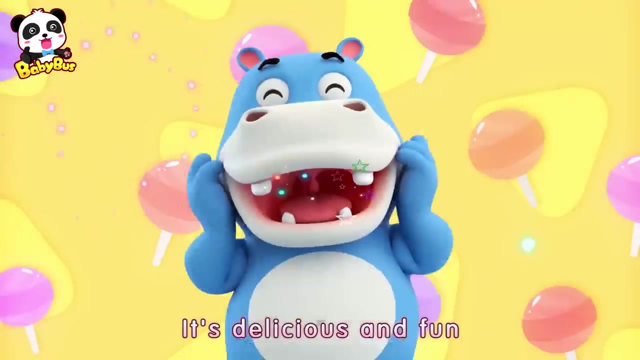 In my own candy shop. Sweet and sour fruit candy, Many colored rainbow candy And lollipops are here. Wow, So many candies. Welcome to my candy shop. How about some milk candy? How about some cotton candy? Mine is popping sugar. It's delicious and fun. 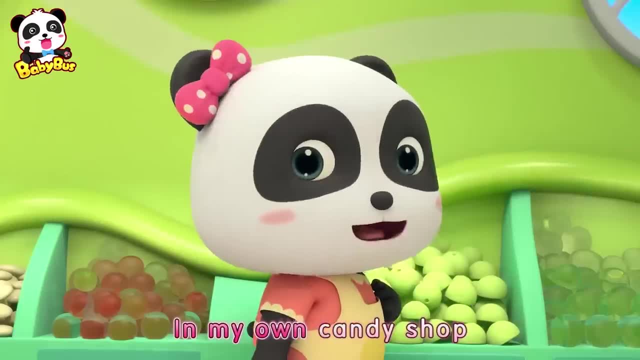 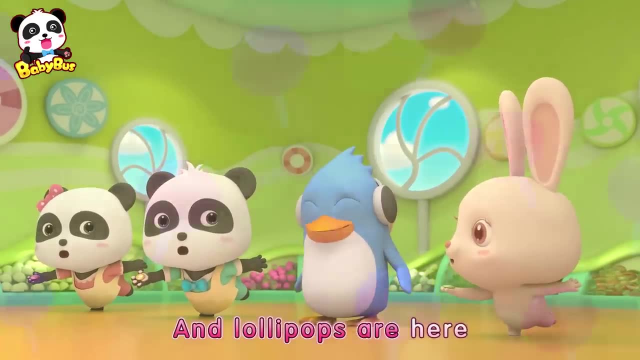 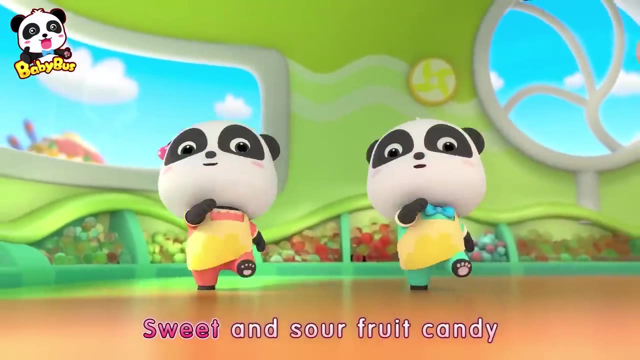 It's delicious and fun. In my own candy shop, Sweet and sour fruit candy, Many colored rainbow candy And lollipops are here. I like rainbow candies In my own candy shop: Sweet and sour fruit candy, Many colored rainbow candy. Everybody, try some please. 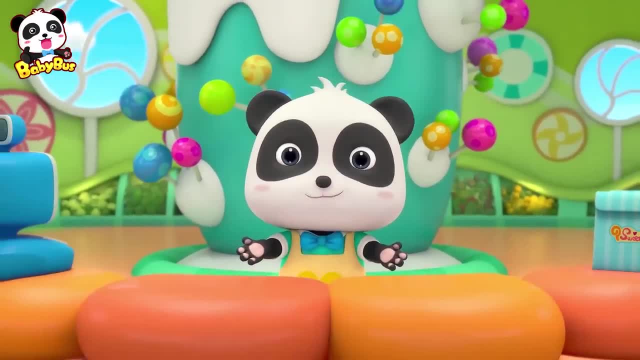 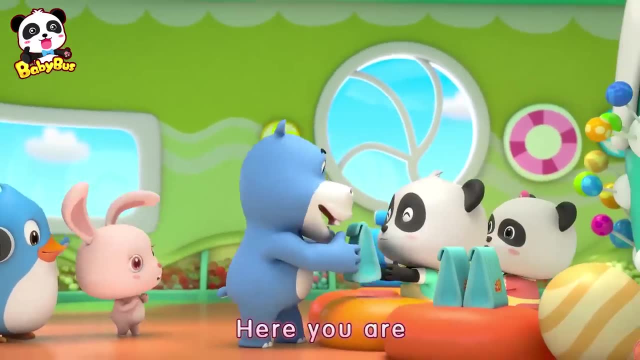 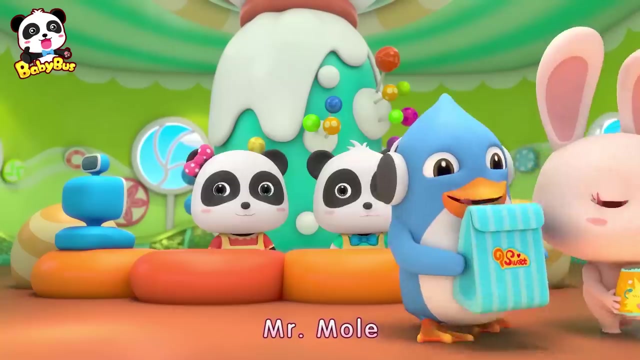 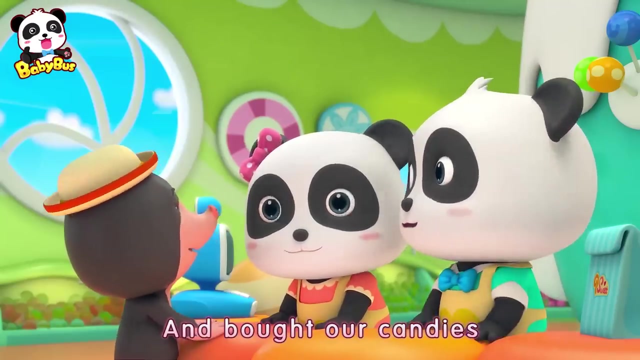 Hey guys, what do you want? Lollipops, please. Fruit candy please. Rainbow candy, please. Here you are. Please come again. Kiki Mew Mew, I'm back, Mr Mole. Many of our friends came and bought our candies. 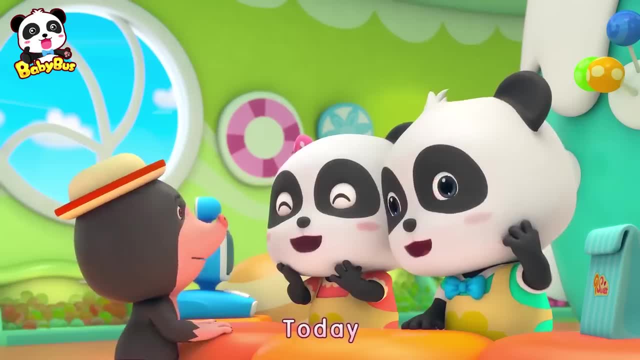 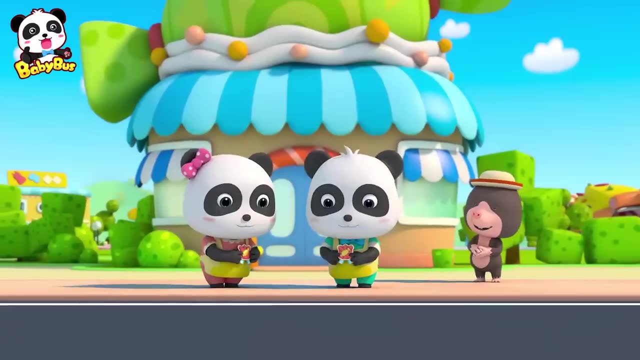 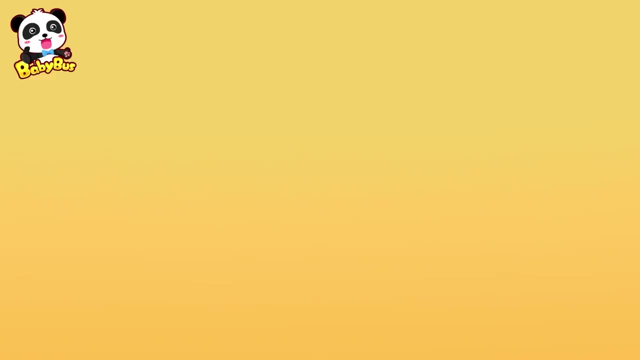 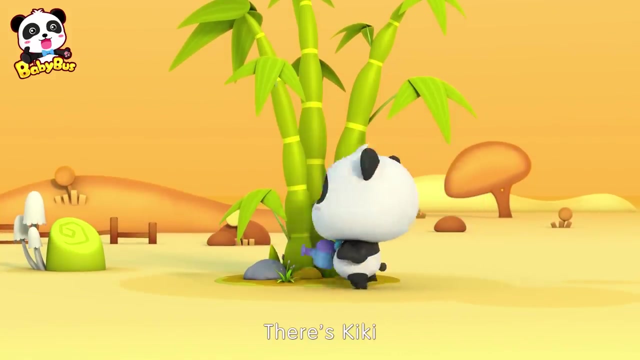 Thank you for your help today. Today, Kiki and Mew Mew helped Mr Mole. Let's give them medals. Oh, there's Kiki. Hi, Kiki, Hi, hello, What are you doing? I'm watering. 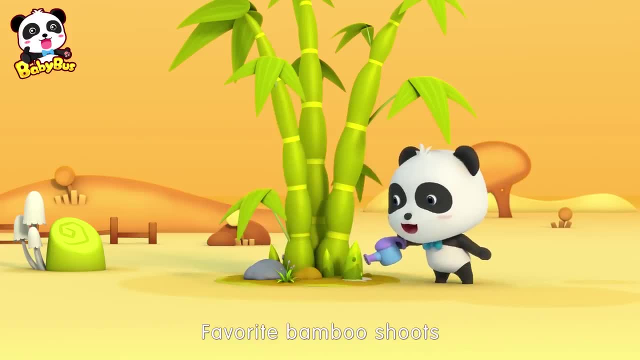 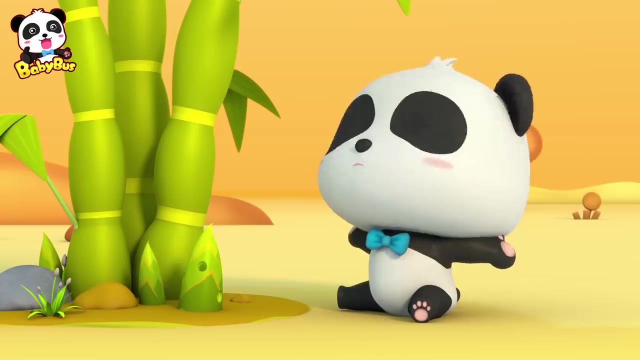 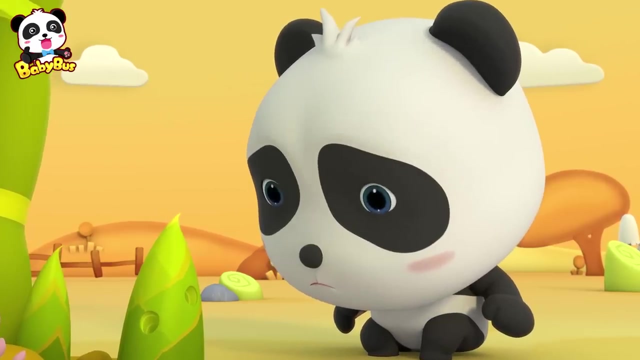 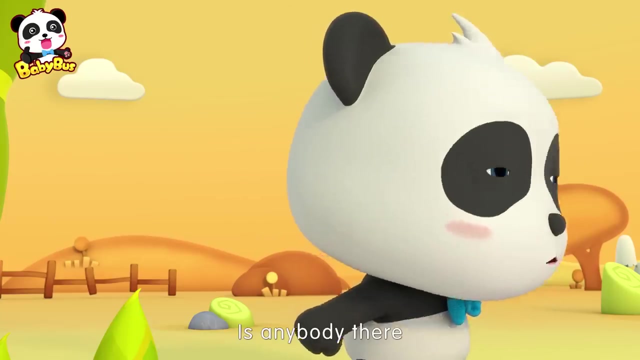 Oh, you're watering your favorite bamboo shoots. Yeah, Kiki, what's wrong? There's a hole, A hole. What happened? What happened? Did anyone take a bite out of it? Kiki, is anybody there? It's Momo. 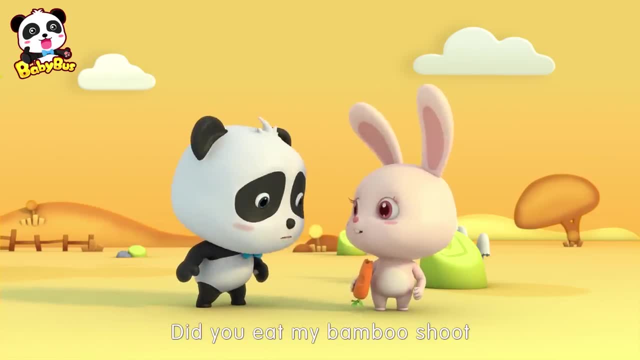 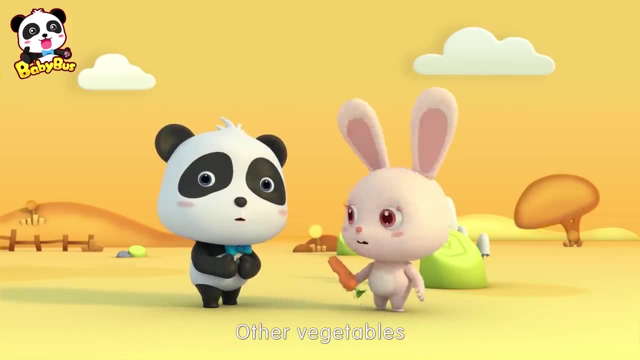 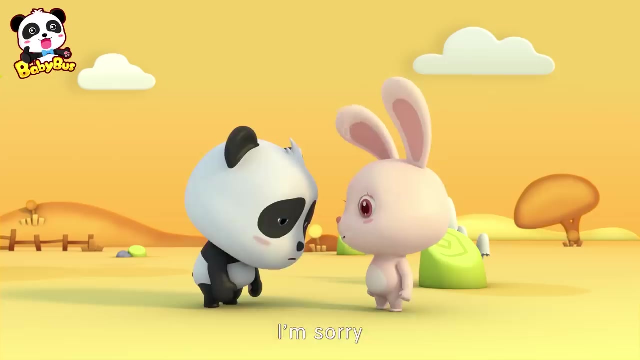 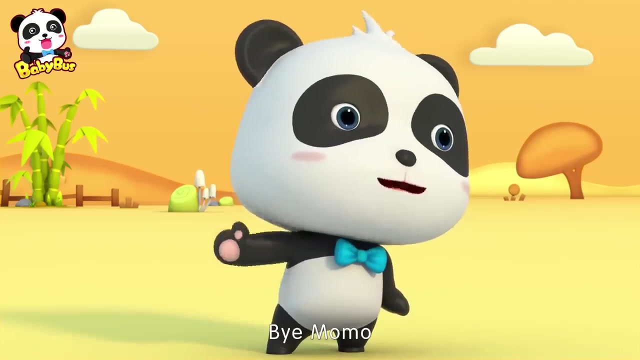 Momo, did you eat my bamboo shoot? But Kiki rabbits love carrots and other vegetables instead of bamboo shoots. Oh, I'm sorry, It's okay, I want to get some carrots. Bye, Bye, Momo. If it's not Momo, then who made the hole in the bamboo shoot? 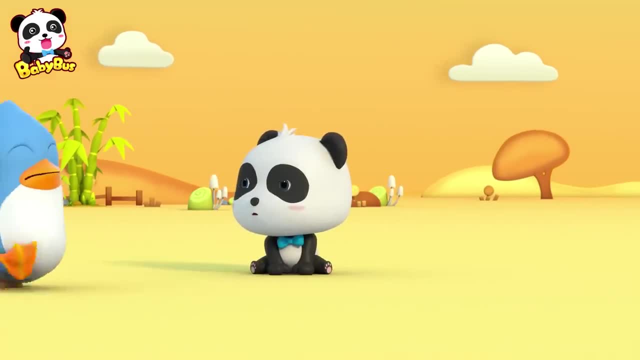 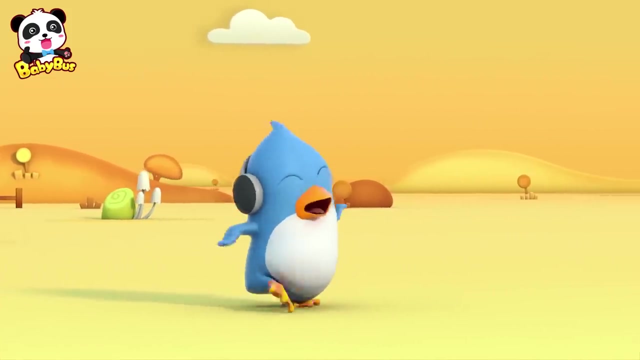 Who is it? Who is it? Is it Are продолжating? Hum, Oh, it's Rudolph. He's a really good dancer. Wow, Donald is very good at dancing. Hi, Rudolph, Rudolph, Rudolph. 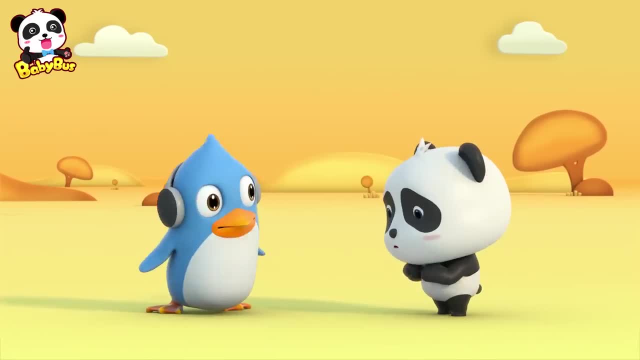 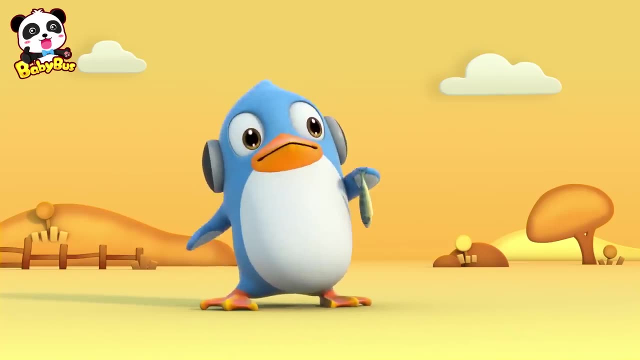 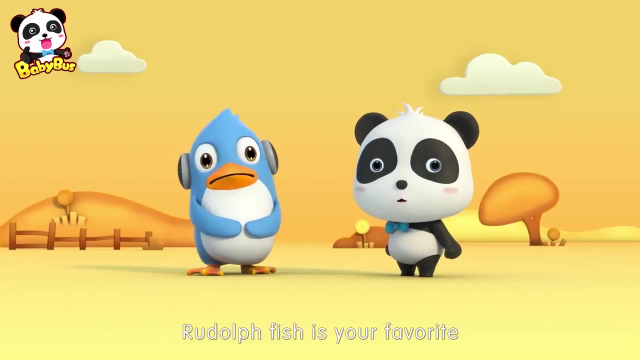 Hey, Rudolph, Rudolph, Rudolph, What's going on? Are you calling me? Did you bite my bamboo shoot? Rudolph, fish is your favorite, isn't it? How about bamboo shoots? I don't eat those. 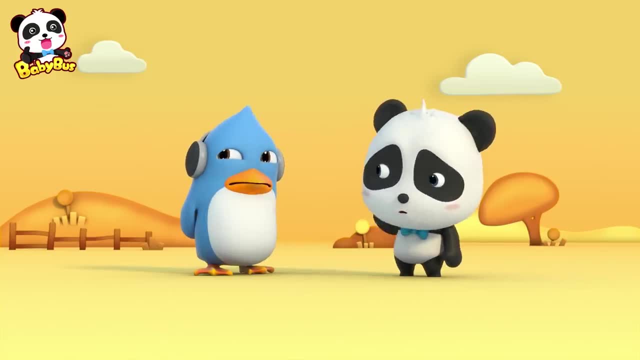 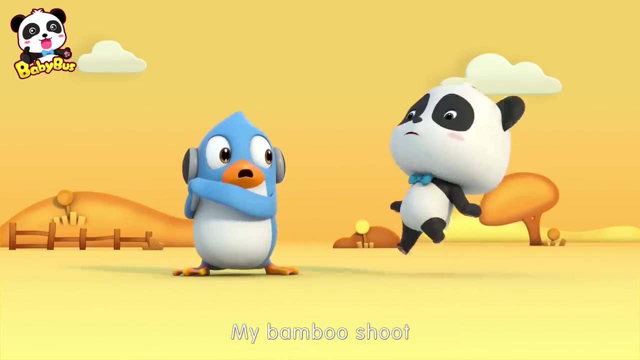 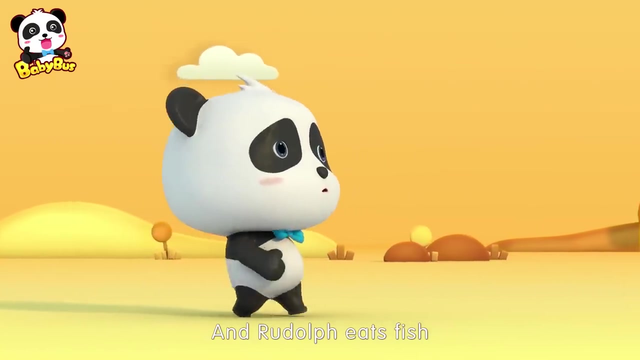 He doesn't seem to eat them either. Let's dance together. Okay, great idea. Wow, you're really good, Kiki. why aren't you dancing If Momo eats carrots and Rudolph eats fish? who ate Kiki's favorite bamboo shoots? 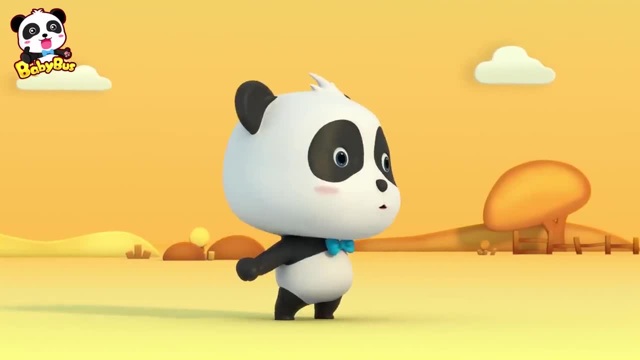 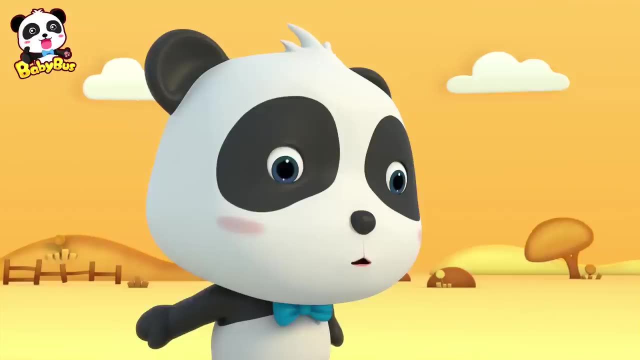 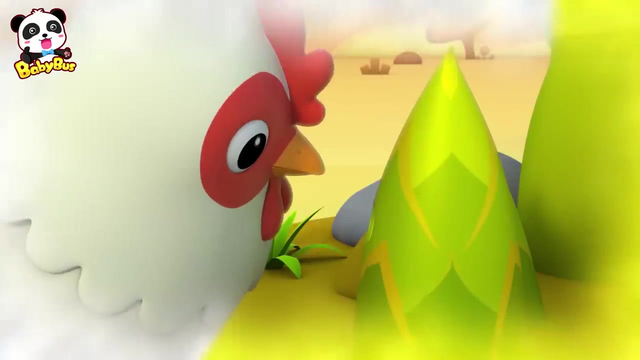 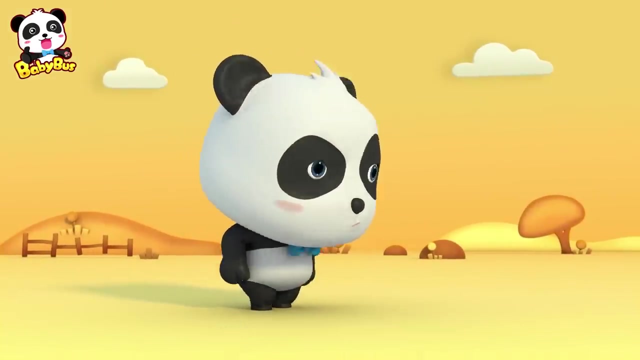 Kiki, what do you see? A hen. You think the hen pecked at your bamboo shoot. Wait, you've been wrong twice already, haven't you? Let's ask her politely. You don't want to be wrong again, do you? 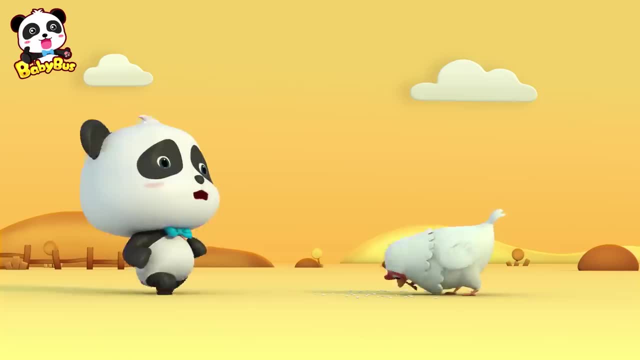 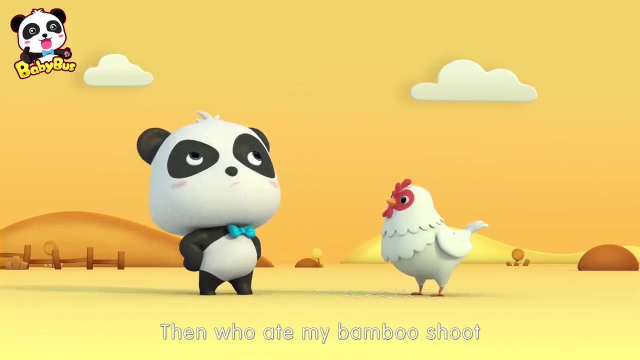 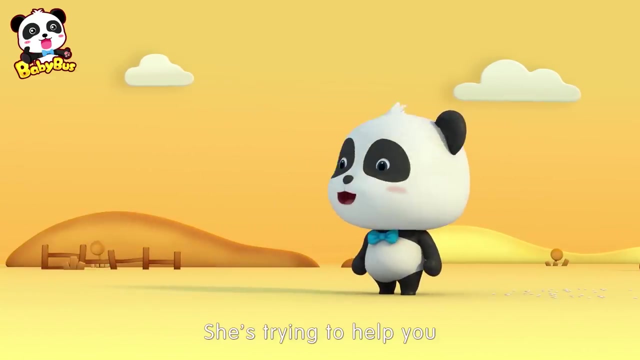 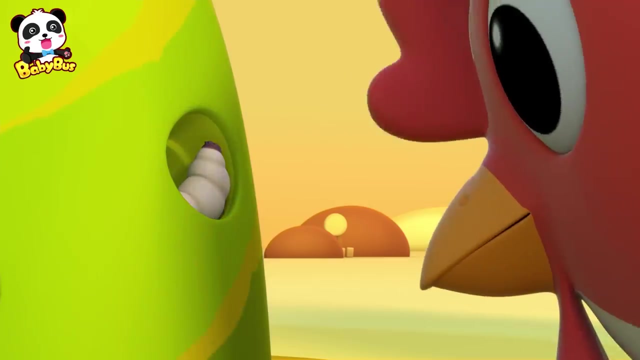 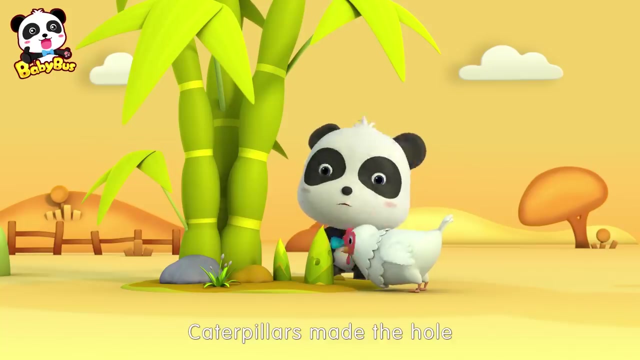 Let's ask Kiki, Miss hen, did you happen to eat my bamboo shoot? Miss hen doesn't seem to eat them either. Then who ate my bamboo shoot? Kiki, follow her. She's trying to help you. Oh, Caterpillars made the hole. 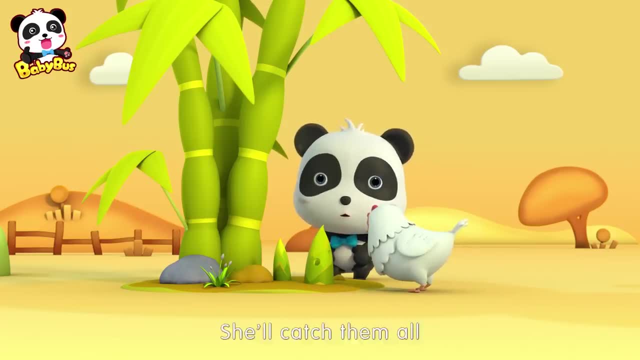 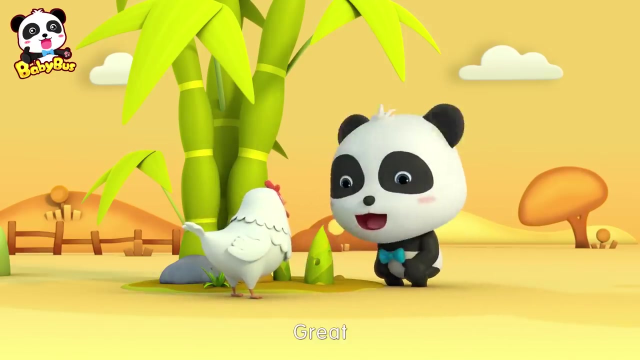 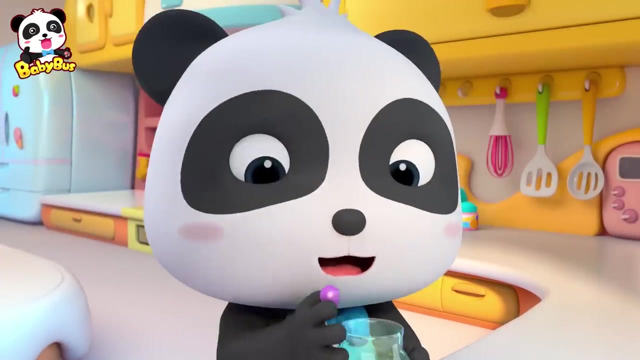 Miss Hen is really good at catching worms. She'll catch them all. Wow, She ate all the caterpillars. Great. Now Kiki's favorite bamboo shoot will grow healthy again- Awesome. Thank you, Miss Hen. Bye, Kiki, can you help me? 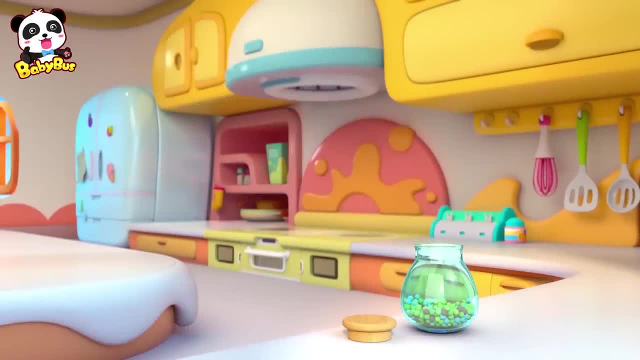 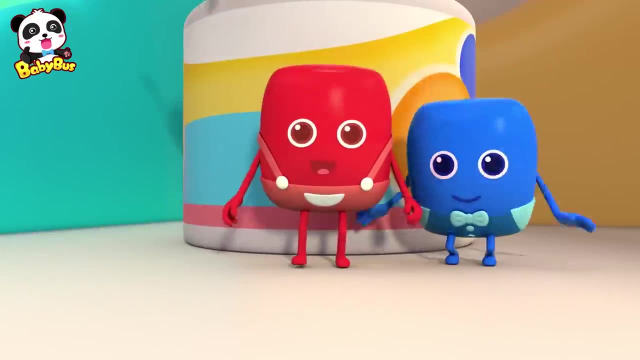 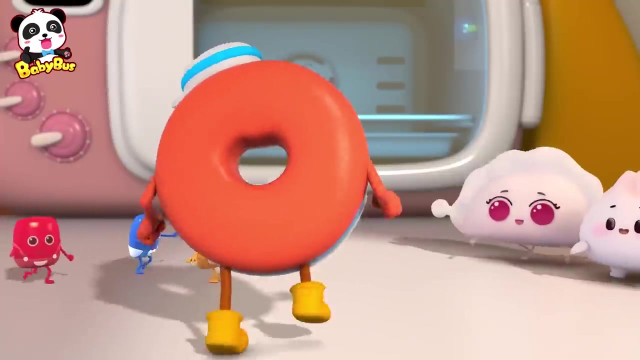 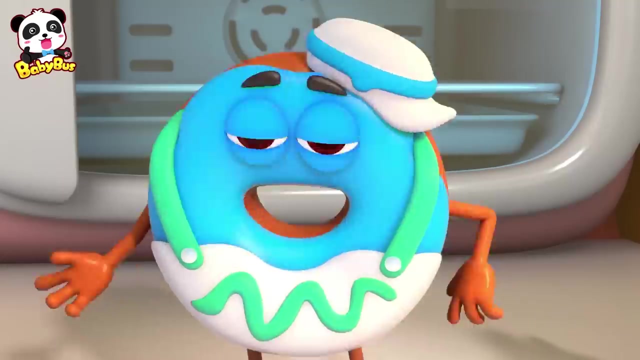 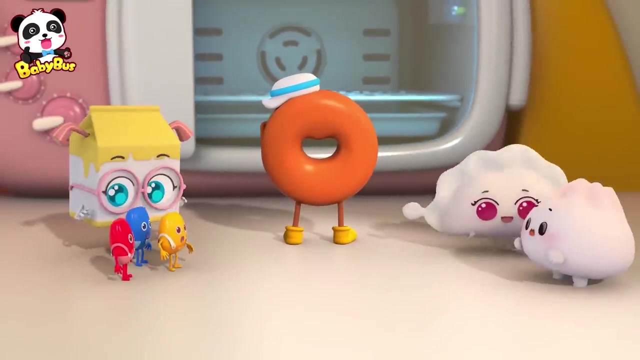 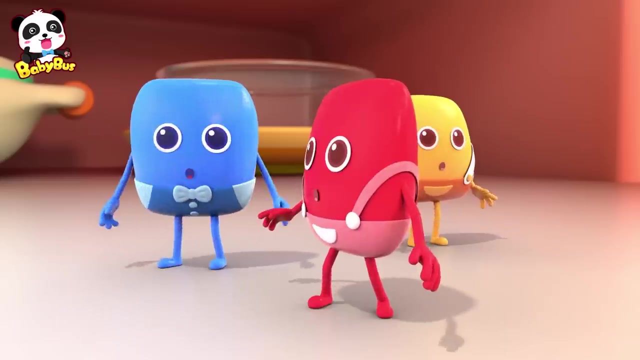 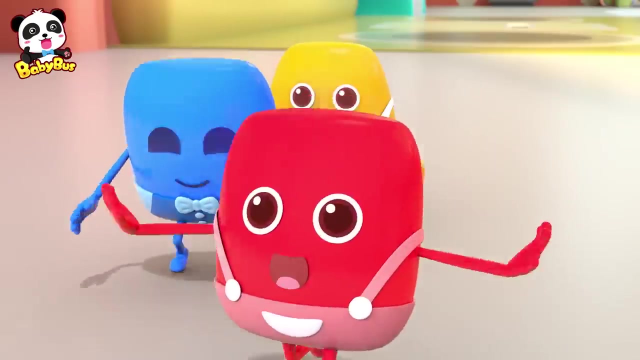 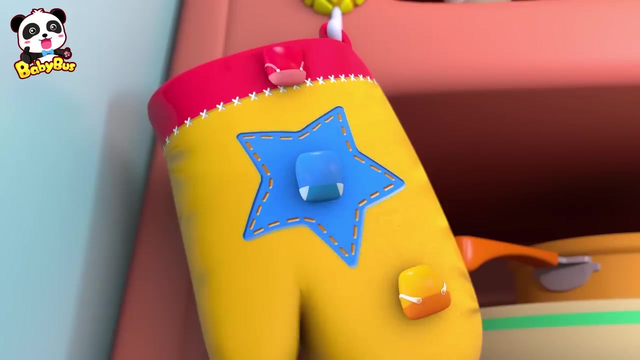 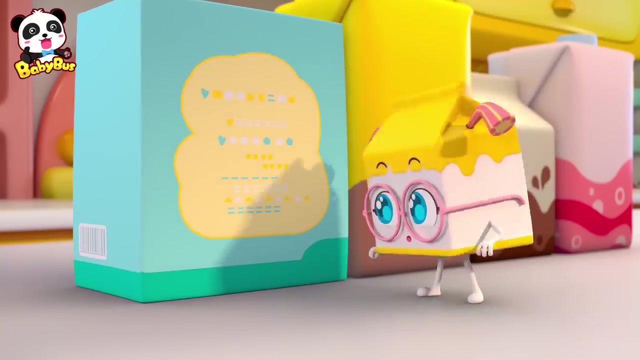 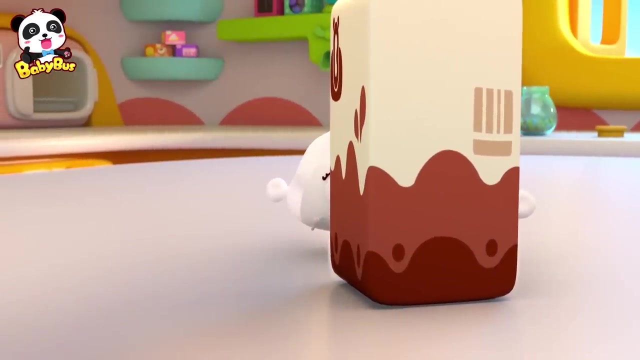 Okay, Let's play hide-and-seek. Yay, I'll be it. first, Go hide everyone. One, Two Over there. Wait, Where should I hide? Ouch, Where should I hide? Aha, That's it. 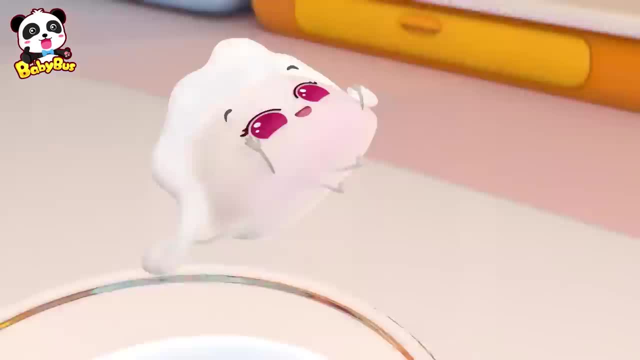 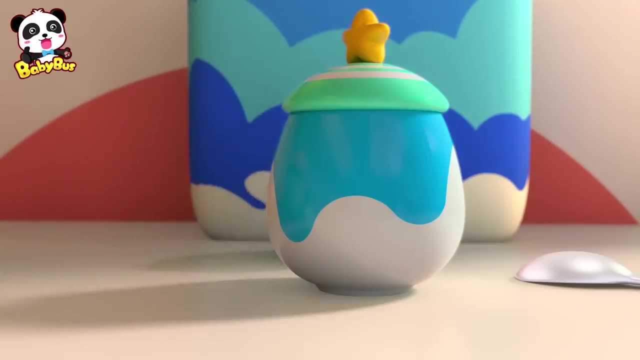 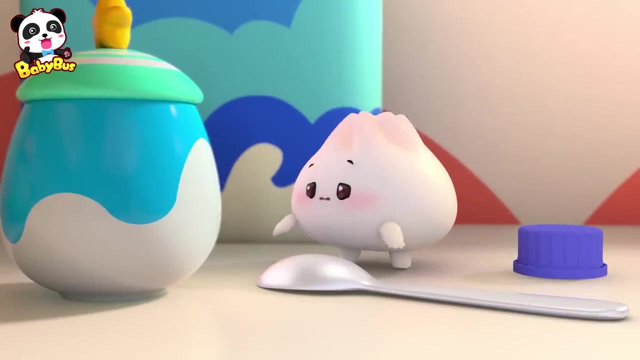 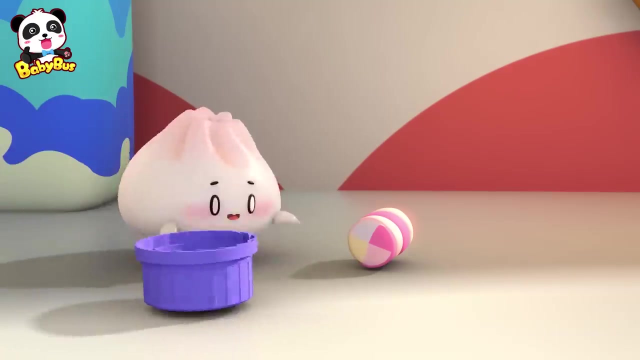 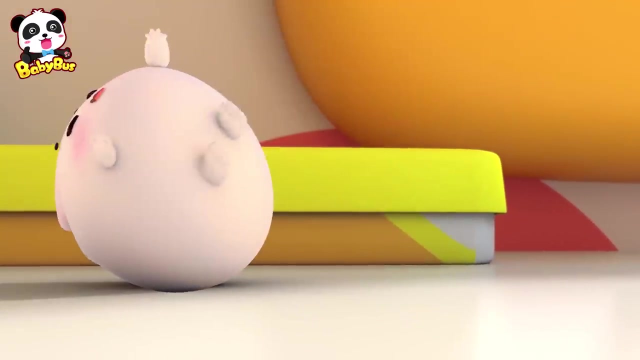 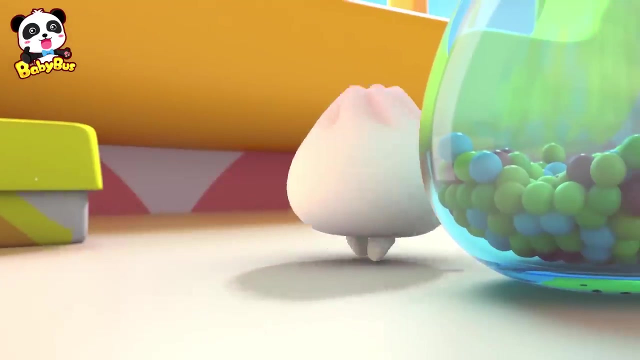 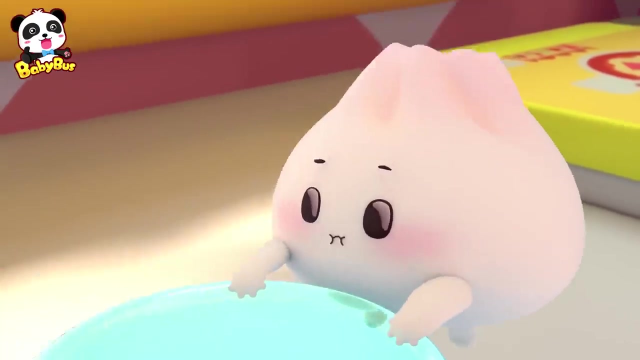 Cha-cha, Ah, Ah, Nine Ten, Ready or not? here I come, I need to hurry. Two, Three, Four, Five, Six, Seven, Eight, Nine, Ten, Eleven, Twelve, Thirteen, Thirteen. 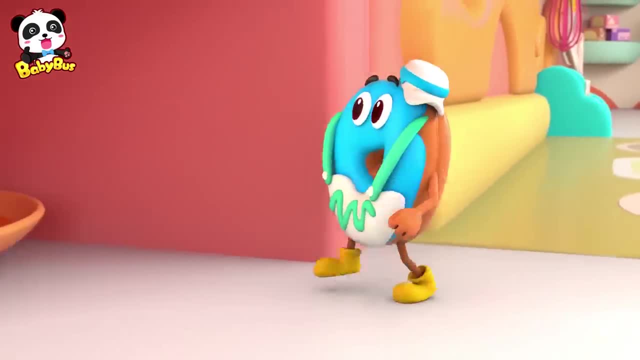 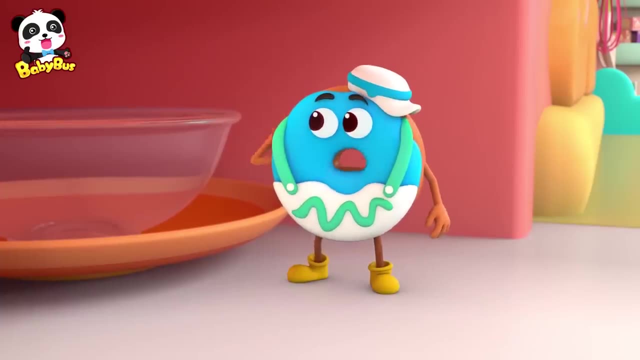 Thirteen, Four, Five, Six, Seven, Eight, Nine, Ten, Ten, Two, Two, Two, Two. I'm gonna get you. Huh, Huh, Huh Huh. Where are they hiding? I found you Three Candies. 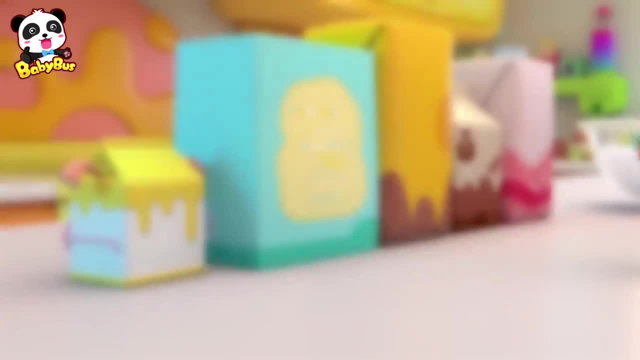 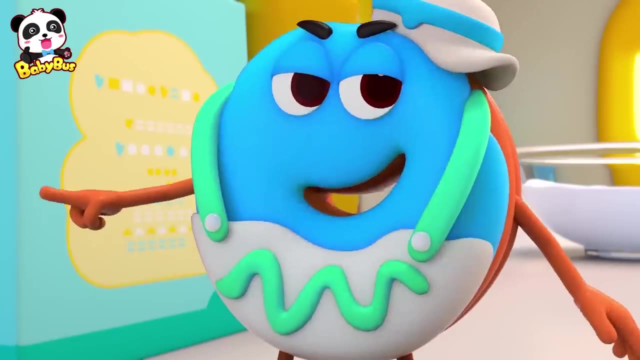 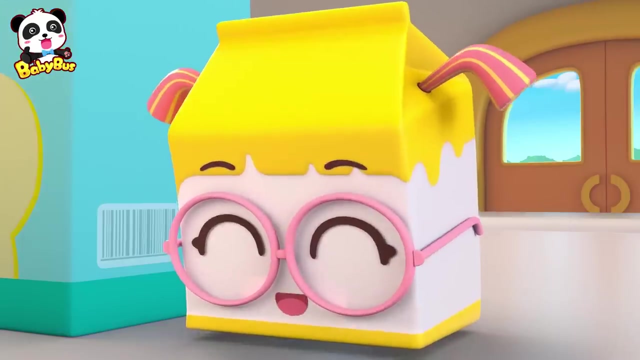 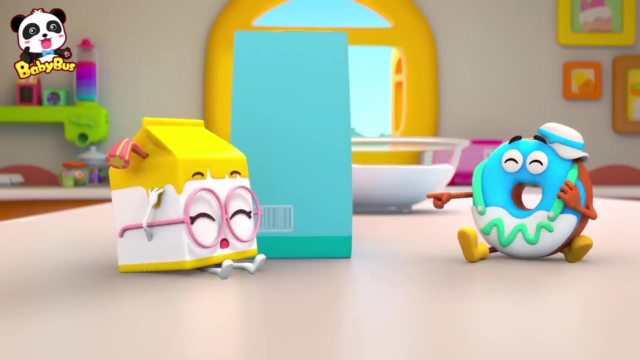 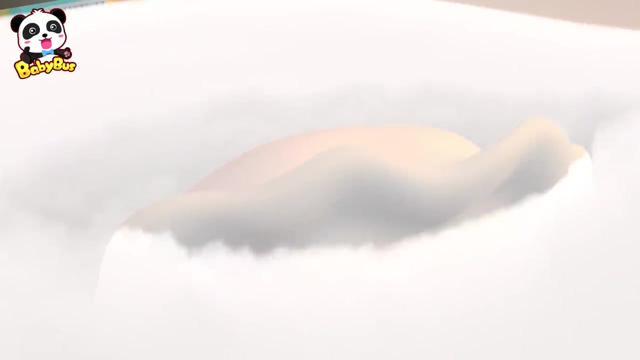 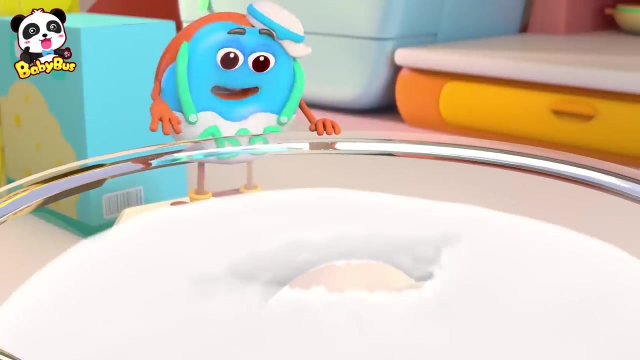 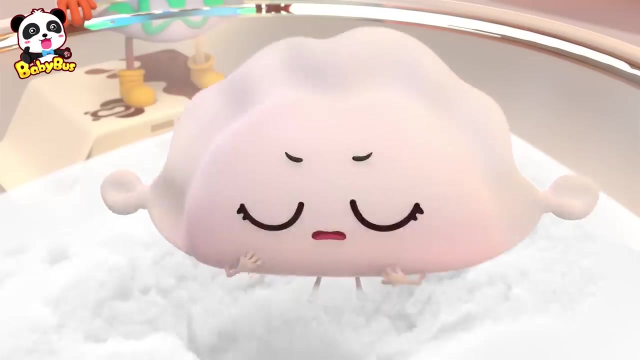 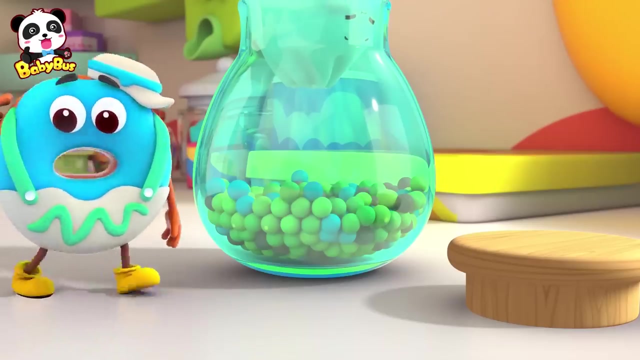 He got us. I found you, Deedee. No way I won't be found so easily. Come out, It's not fun. You found me. You found me too quickly. Now only Bo is left. Where is he? 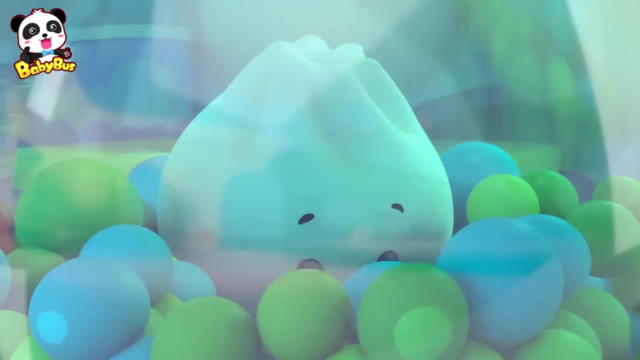 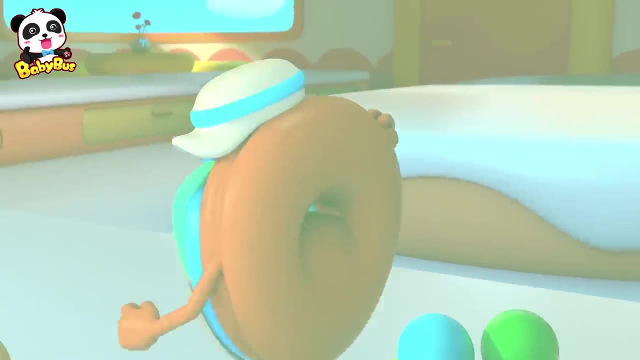 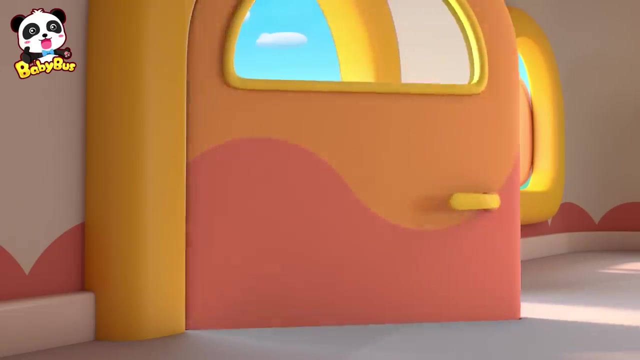 What's that sound? Maybe it's Bo. He must be around here somewhere. What's that sound? He's coming for us. Oh, I can't believe it. I found you Three Candies. I found you Three Candies. 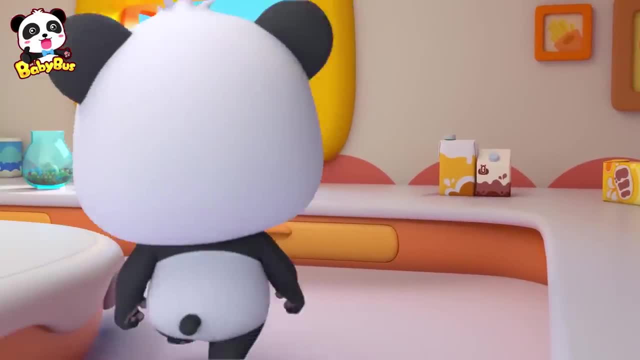 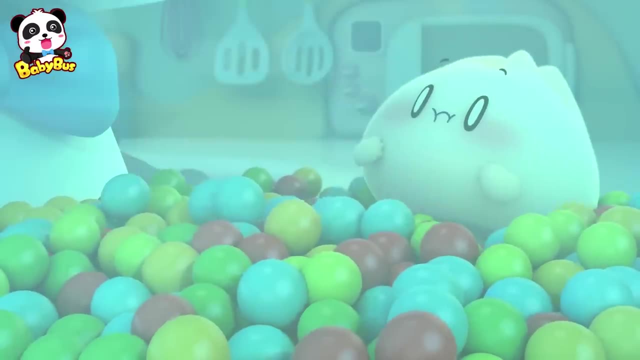 You two are so cute, But I found you Three Candies. I'll never find you again. I'll never find you again. Ha ha ha. What are you doing? Three Candies. You're going to find me again. You're so cute, Three Candies. 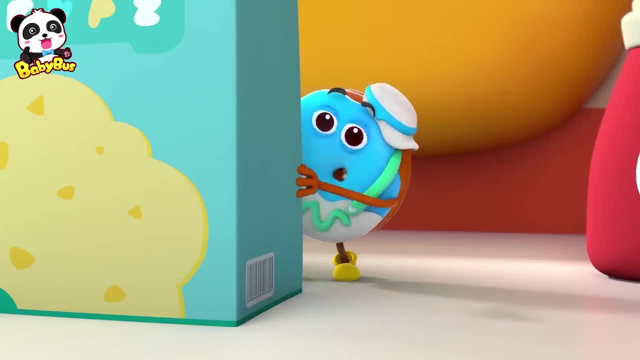 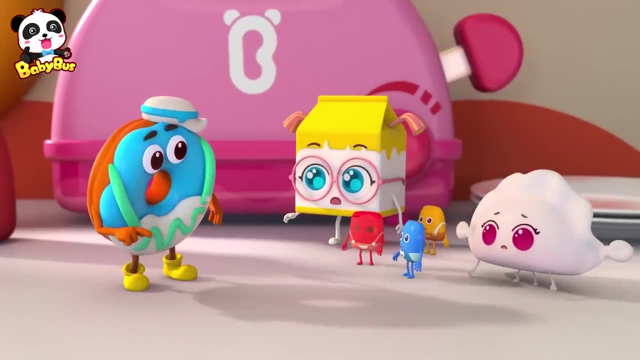 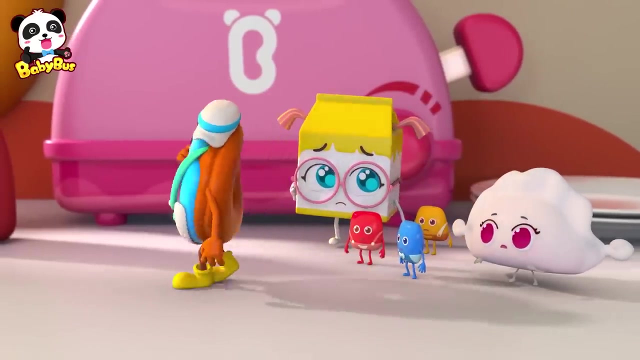 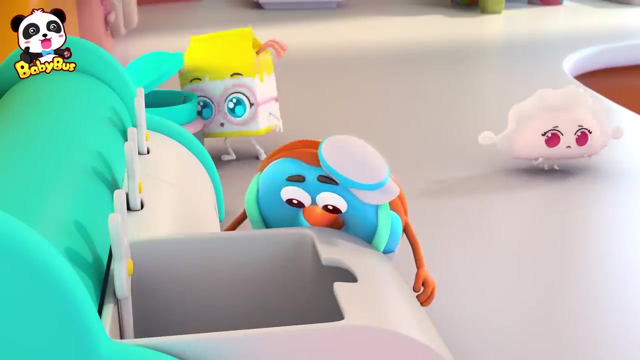 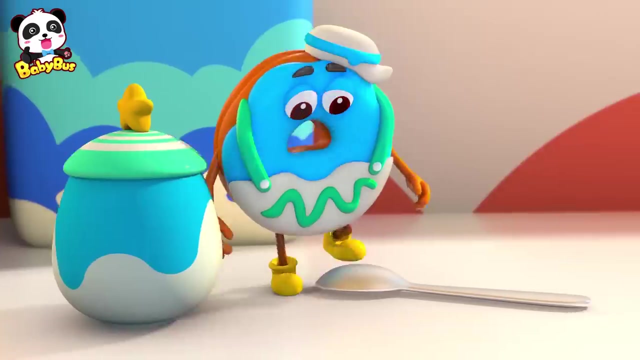 You're so cute- Three Candies. You're so cute- Three Candies. I still can't find Bo. Where is he hiding? Maybe something bad happened to him. We need to find him. I still can't find him. We've looked everywhere. 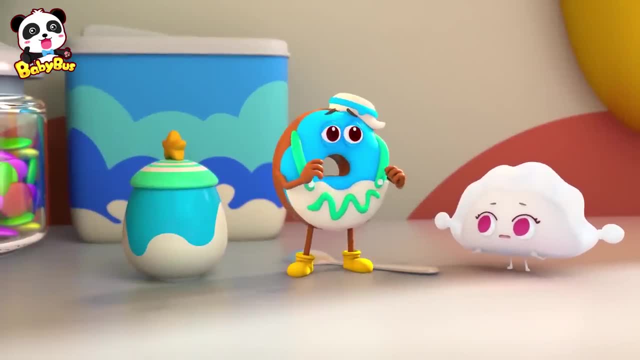 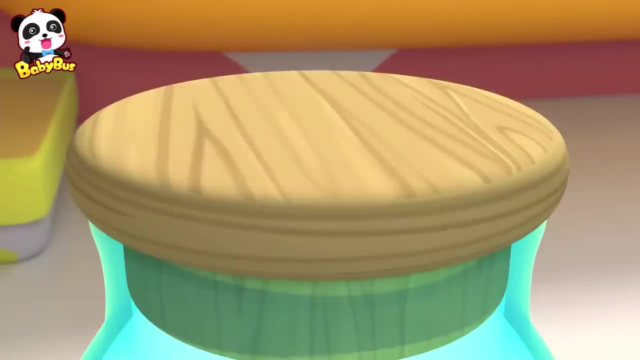 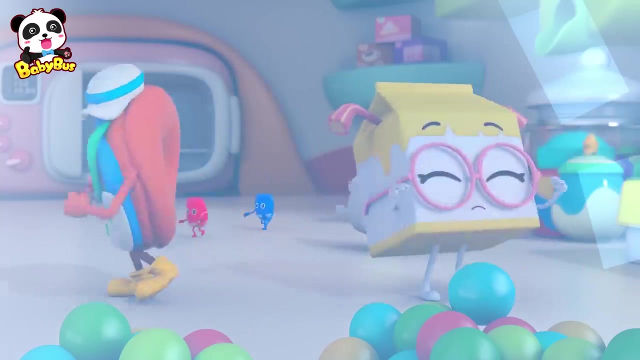 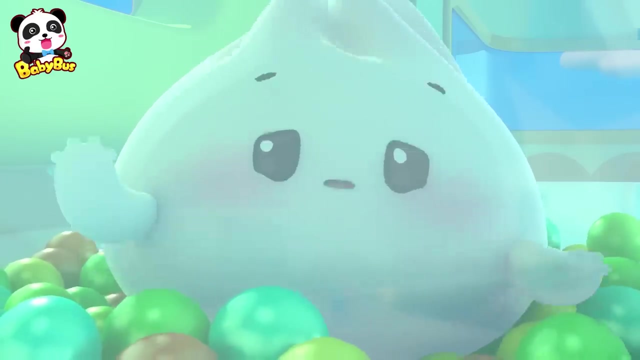 Hey, Bo You win, Come out, now I win. Come out, Bo, You're the winner. Bo, Come out, I can't get out, Let's look somewhere else. Help, Hey, I'm here, Please help me. 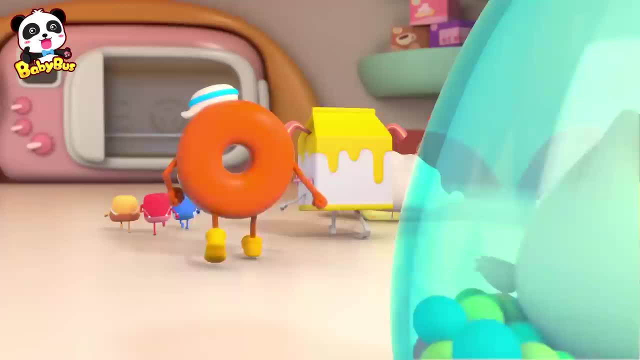 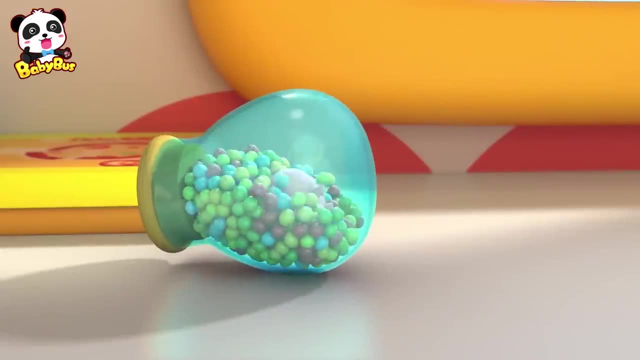 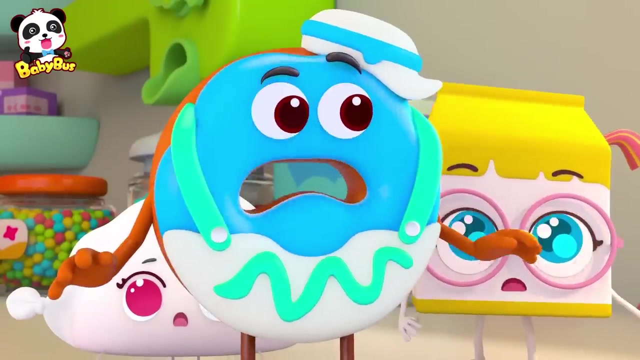 I'm here, Please help me. I'm here, Please help me. What should I do? What should I do? Let's go, Let's go. Huh, It's Bo, Huh, It's Bo, Huh, It's Bo. 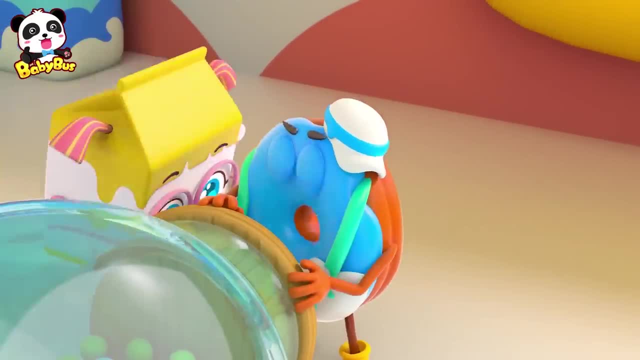 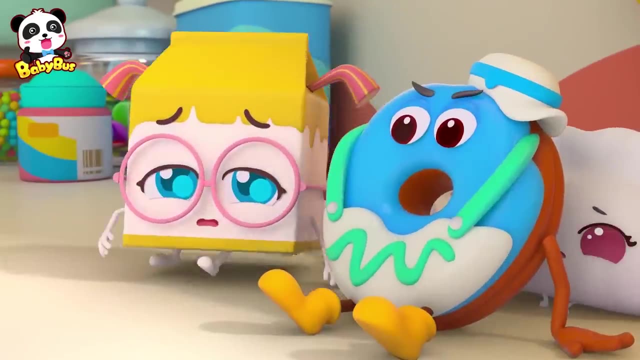 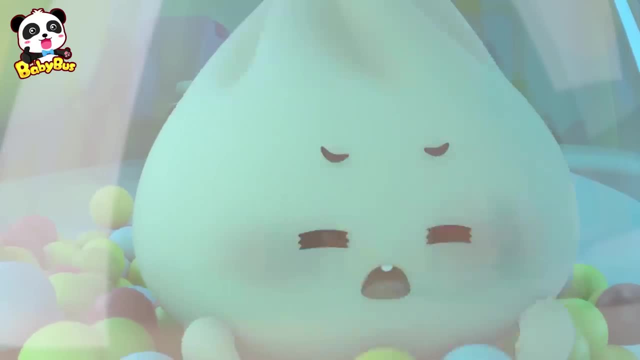 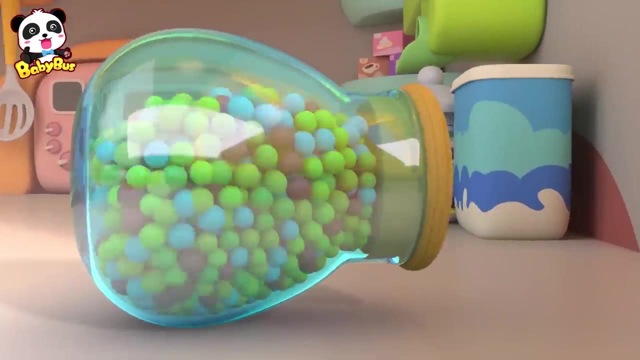 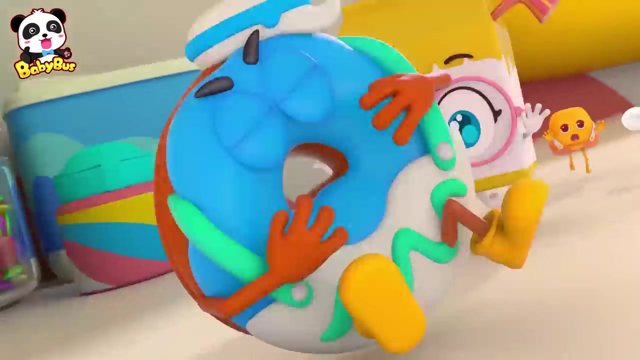 It's so tight we can't open it. Let me out, I can't breathe. Let me out, I can't breathe. Let me out, I can't breathe. Help, Help, Help. What happened? Help me, Help me. 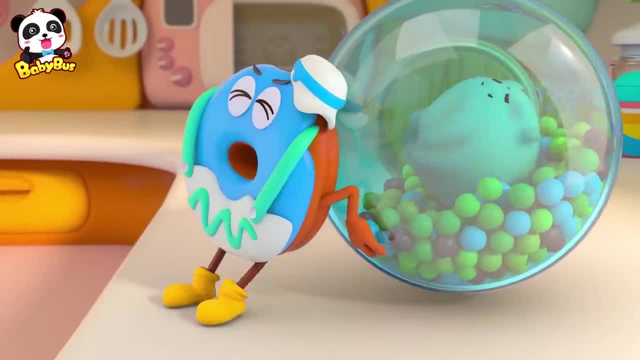 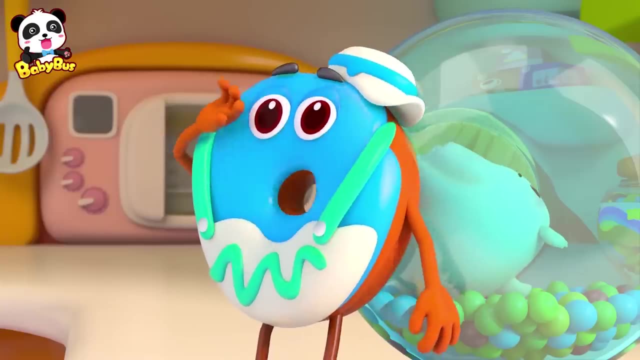 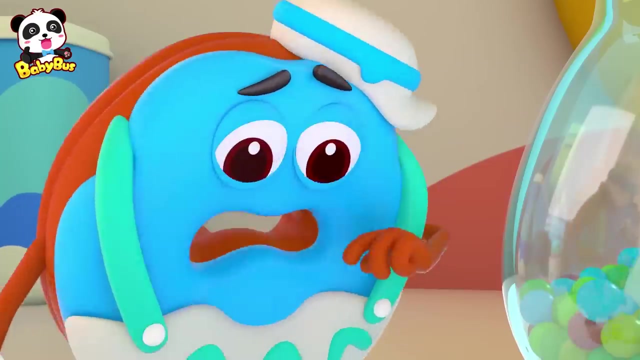 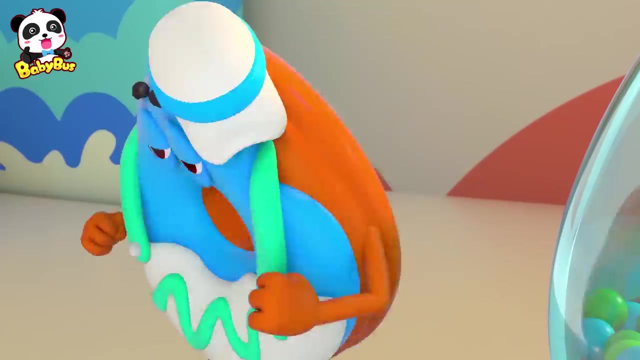 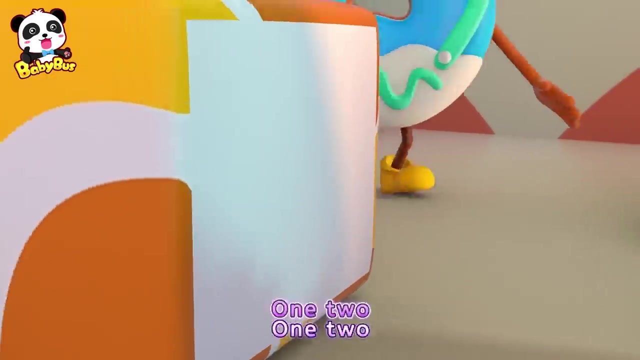 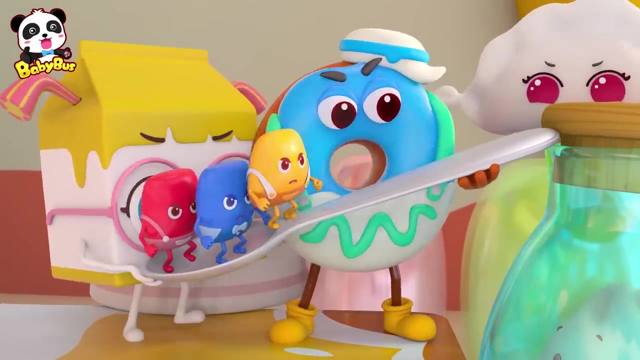 That was close. We need to find another way. Huh, I have an idea. One, two, one, two, one, two, Stop. One two. one, two, one, two Ready. One, two, three, four. come on everyone. 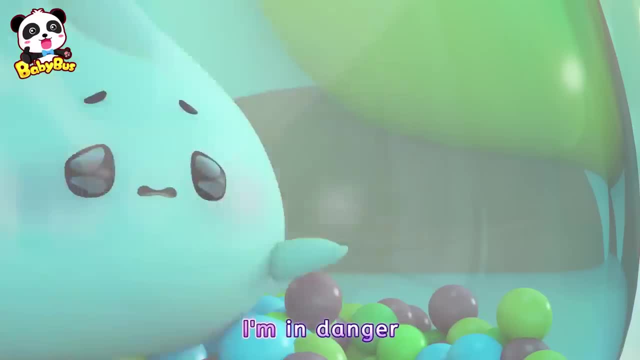 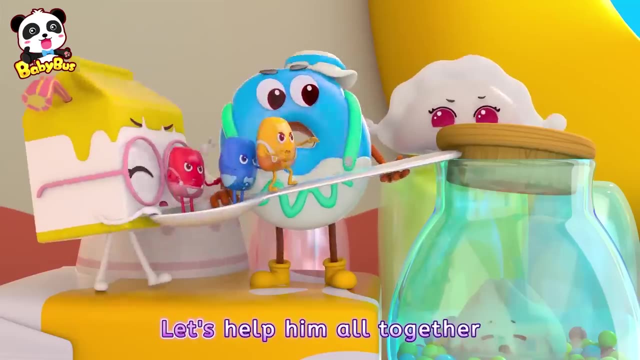 All together, help our friend out. I'm in danger. I'm in danger. Let me out. let me out. I'm so scared. Let's help him all together. Ah, it's open. Let's help him all together. I'm stuck. 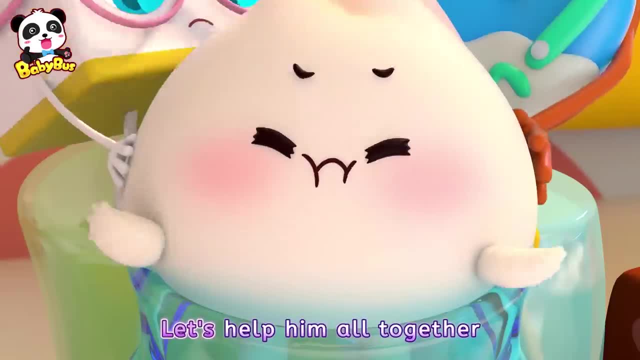 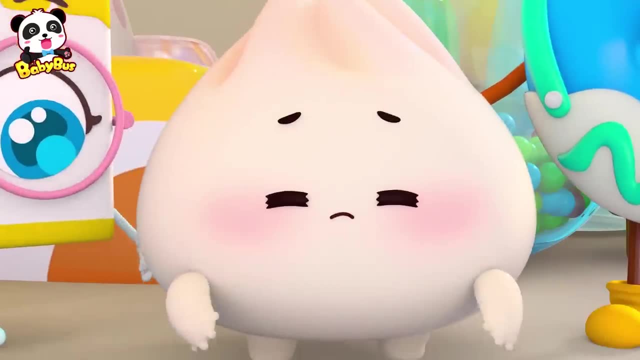 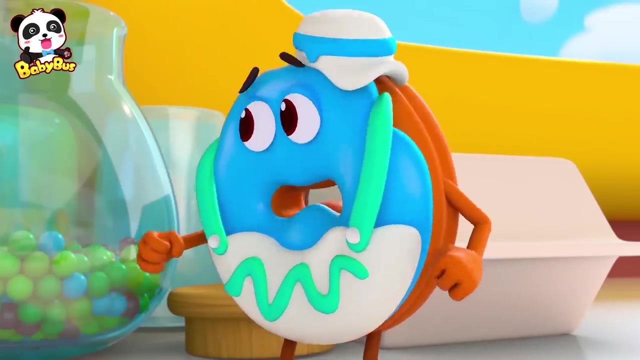 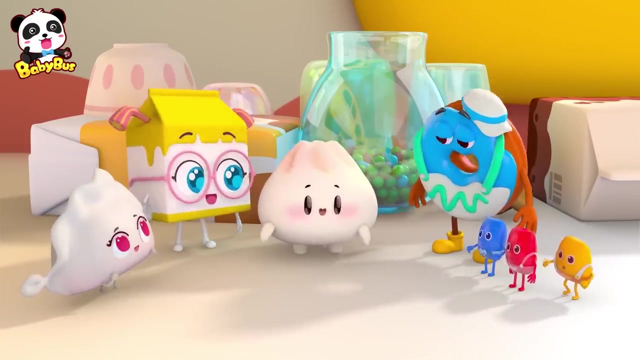 Let's help him all together. Almost done. Let's help him all together. Yay, we did it. Thank you for helping me, guys. It was so dangerous. I will never hide in a bottle again. Kids, you need to be careful when you play hide and seek. 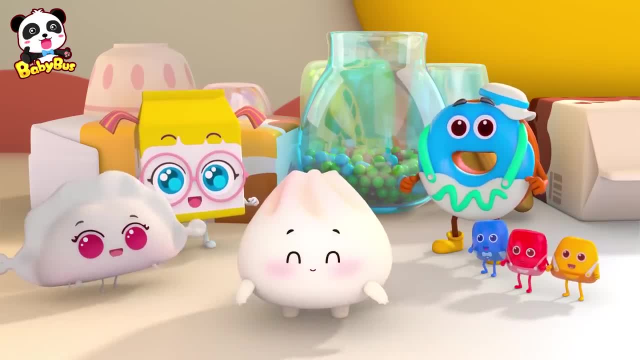 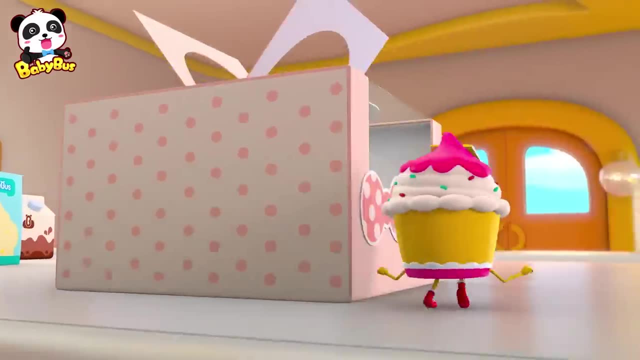 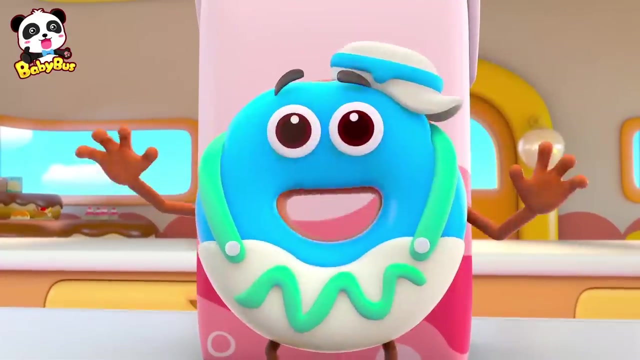 Only hide in safe places. Only hide in safe places. One, two, three, four, five. Are you ready, Ready or not? here I come. Are you ready, Ready or not? here I come. Are you ready, Ready or not? here I come. 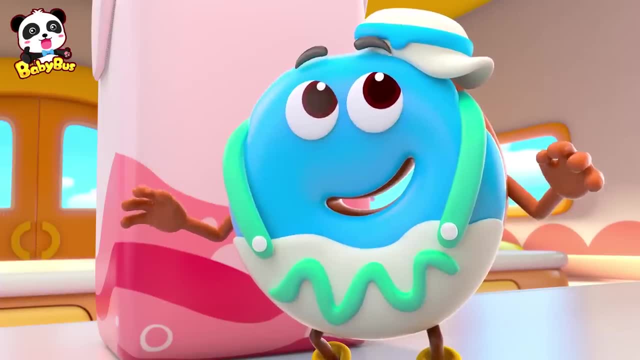 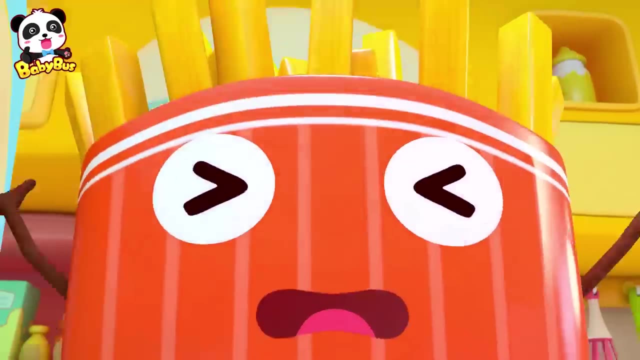 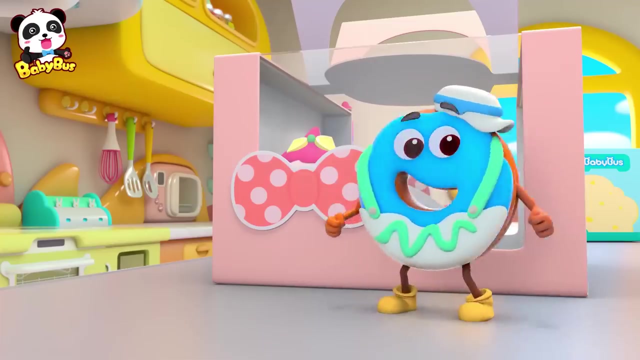 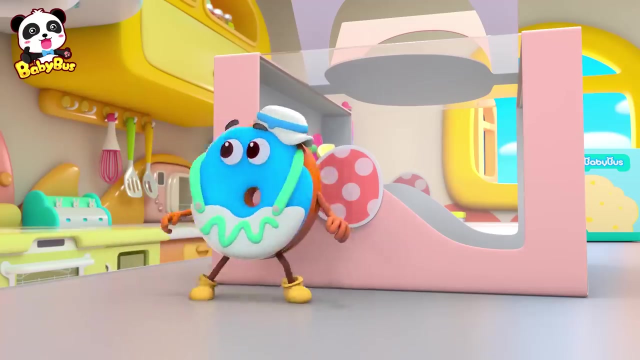 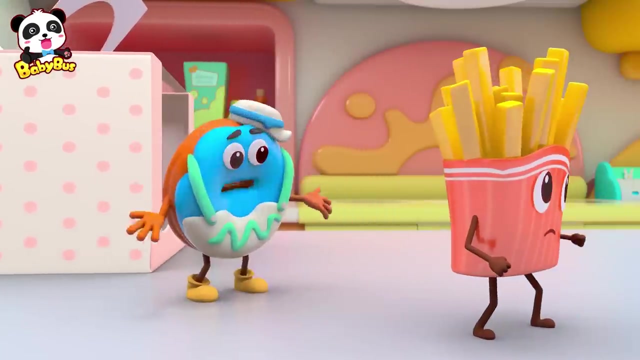 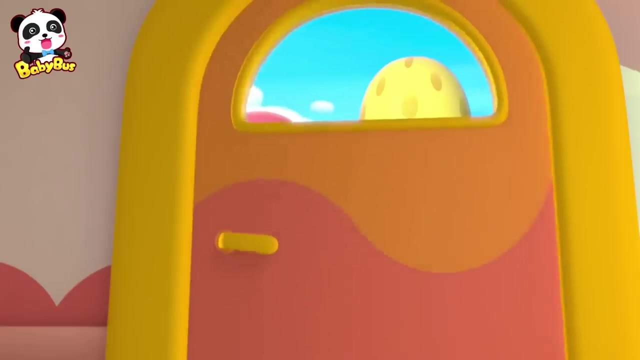 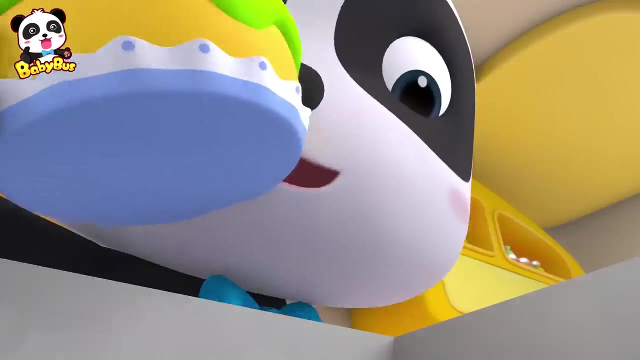 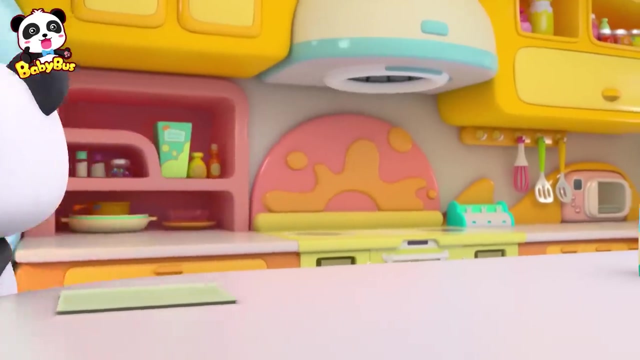 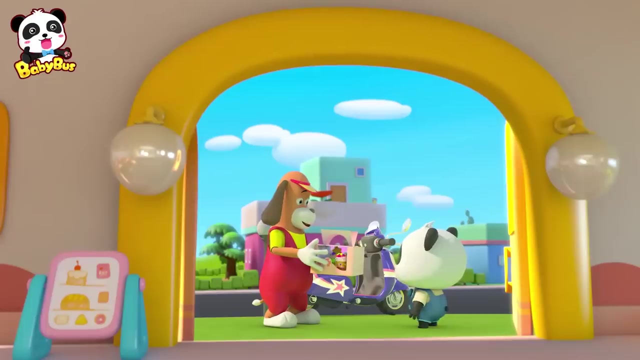 Huh, Oh, Yay, Yay, yay, Yay, yay. I found you. You got me so quickly. Where is Katie? I can't find her. Please deliver this cake to Rudolph. Okay, no problem. 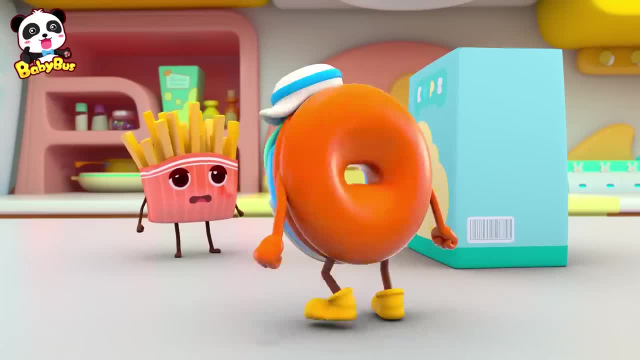 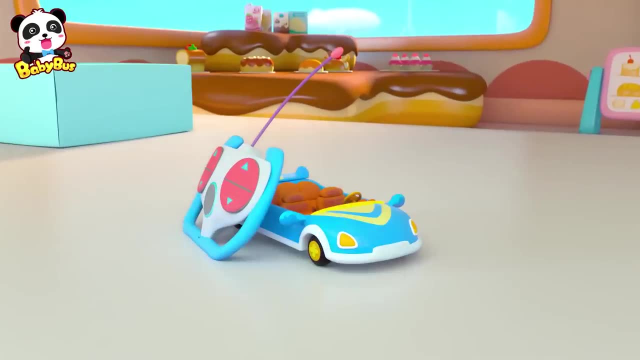 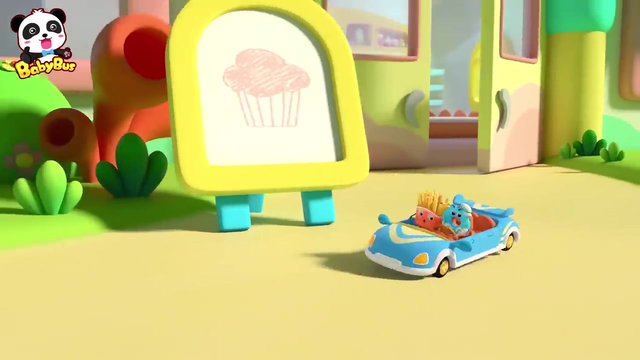 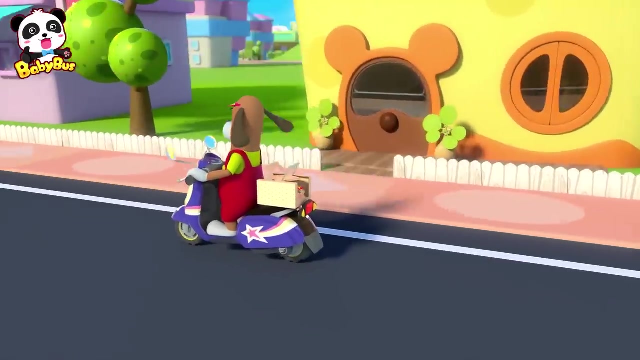 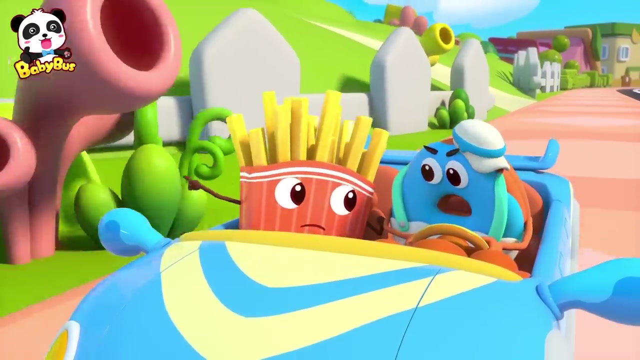 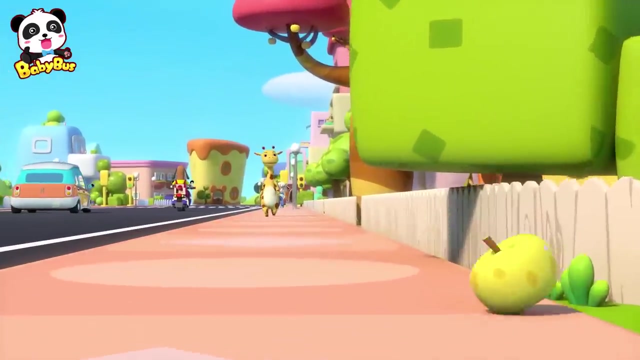 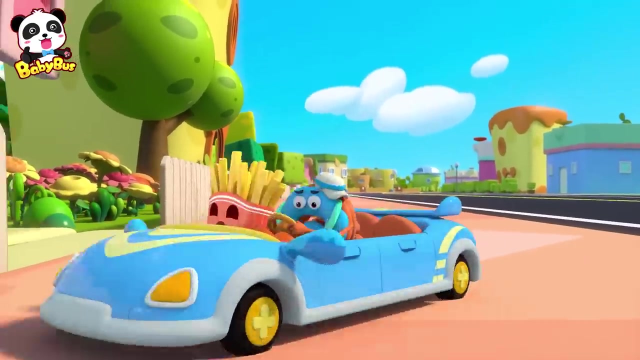 Oh no, Katie is in the box. What should we do? That's it. Let's go save her. Okay, We're there. Hurry up, No problem, Full speed ahead. Ah, Ah, Ah, Ah Ah. 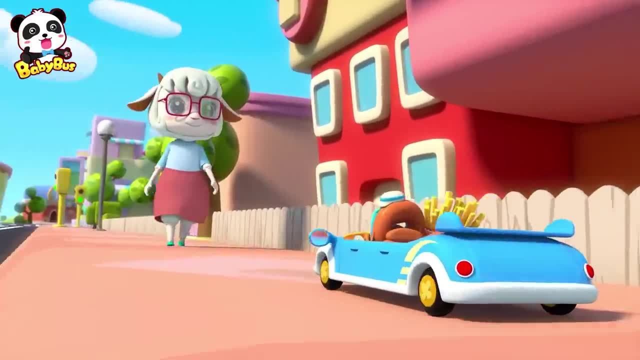 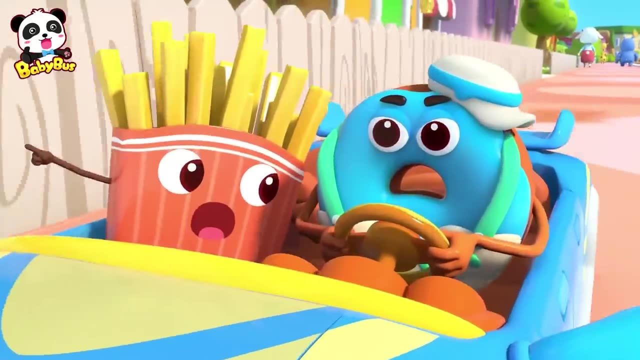 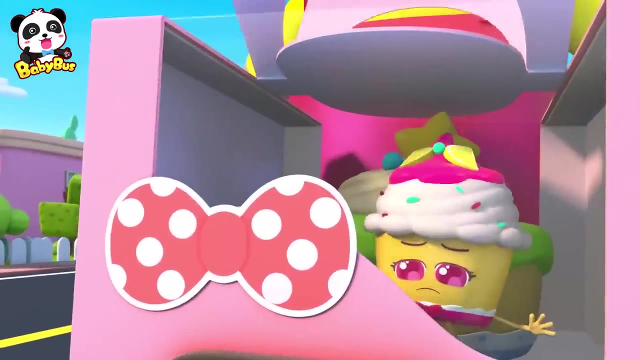 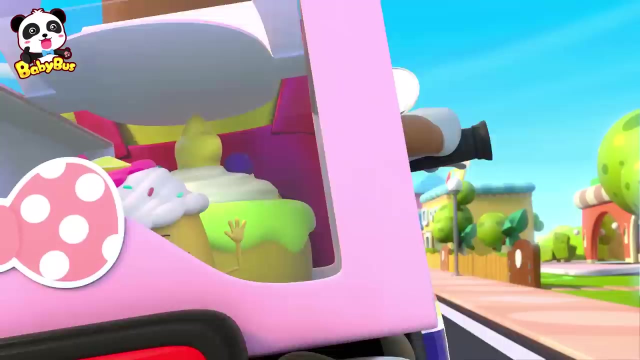 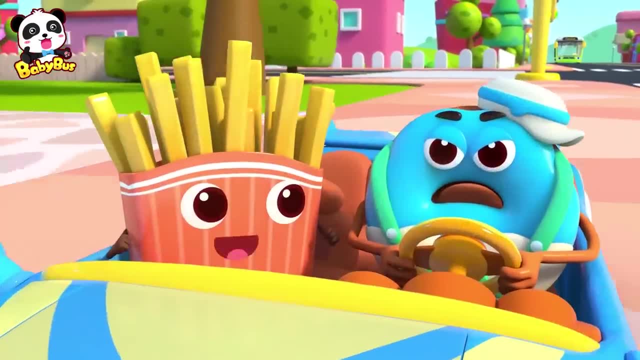 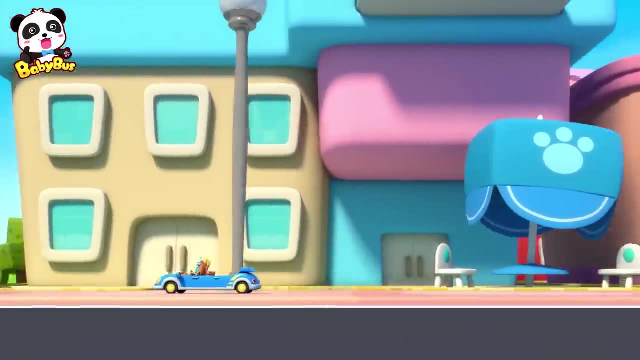 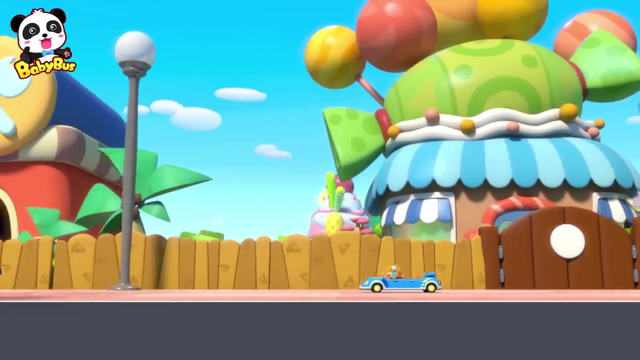 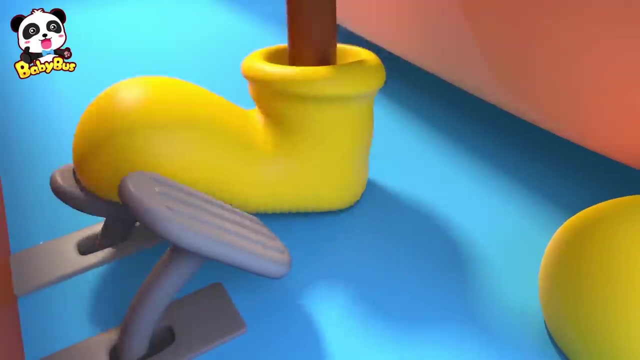 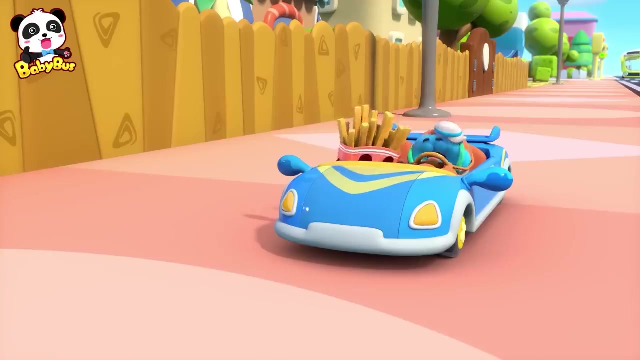 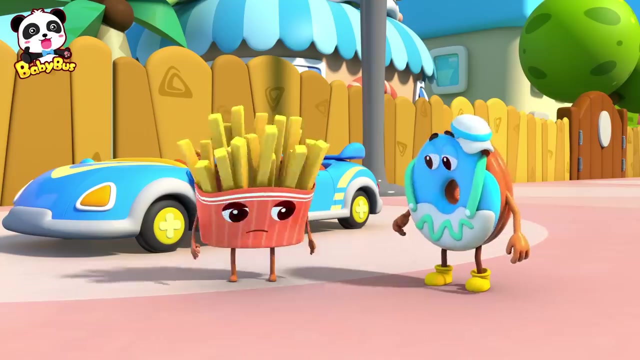 Here, Save me. Yay, We're almost there Faster. Trust me, I'm really good at killing. Oh, driving Hurry, we need to speed up. Oh no, We're out of battery. What should we do? We won't be able to get Katie. She must be so scared now. 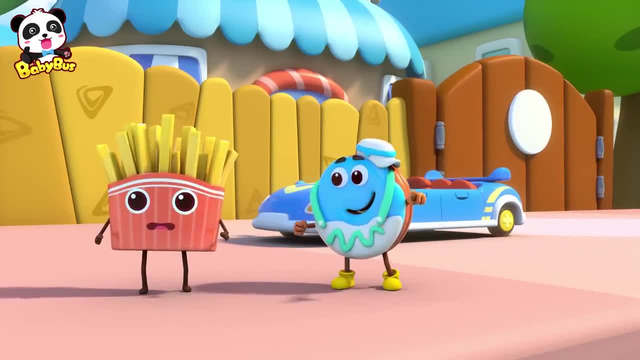 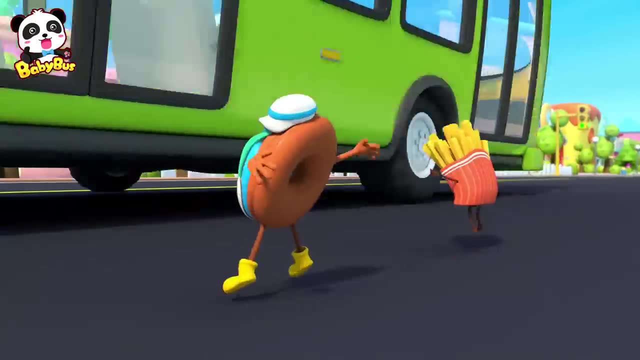 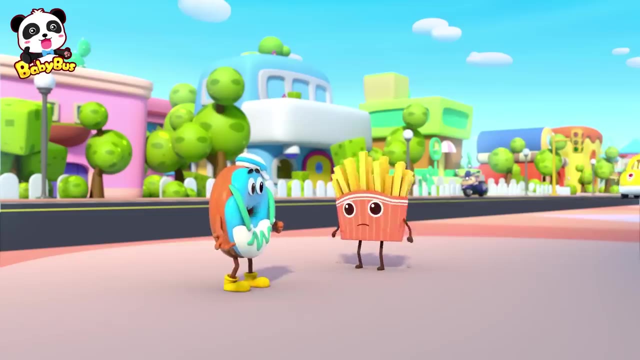 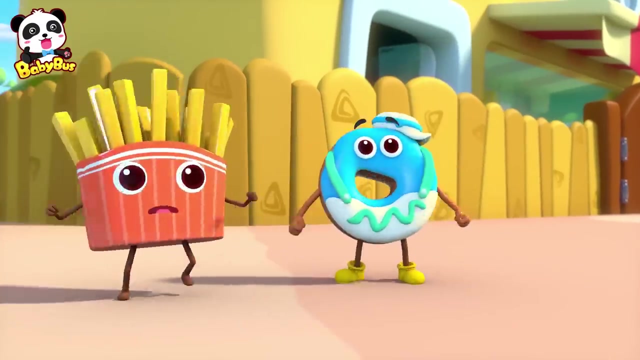 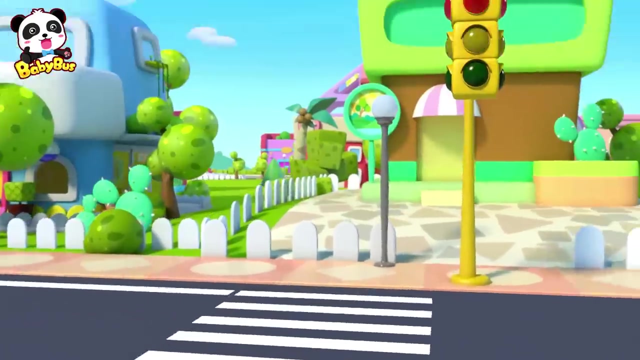 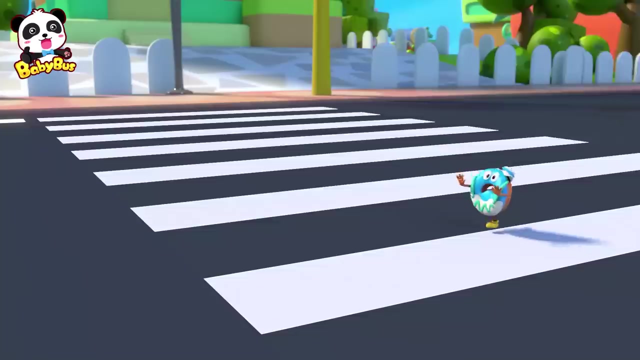 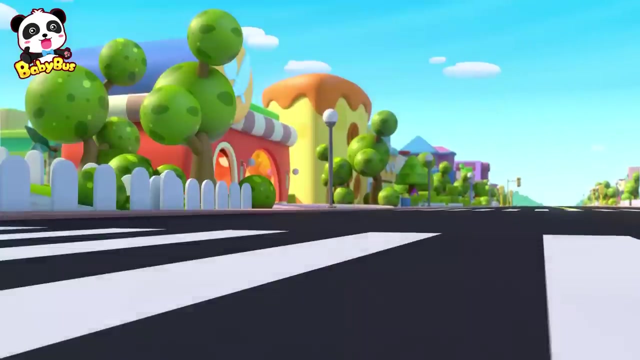 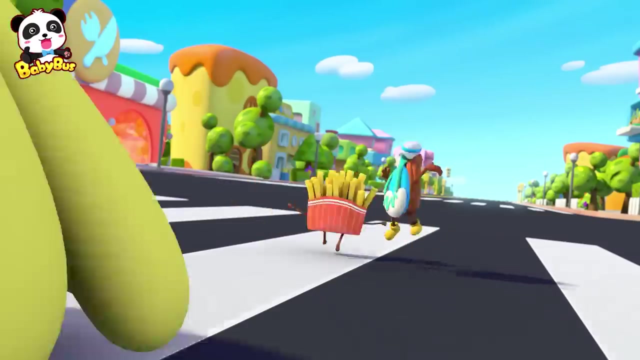 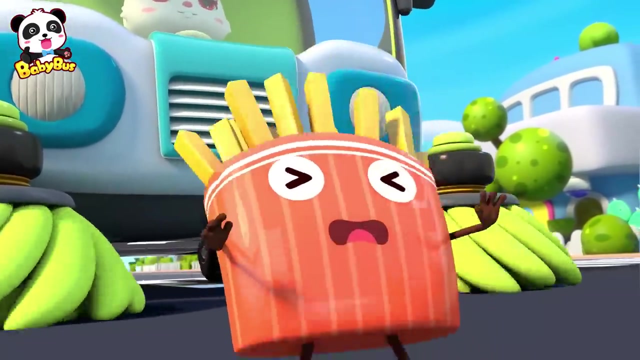 Hey look, She's over there, Let's go. Oh no, We can cross when the light turns green, It's green, Let's go. Aargh, Ahhh, Ah, puh-puh-puh, Ahhh. 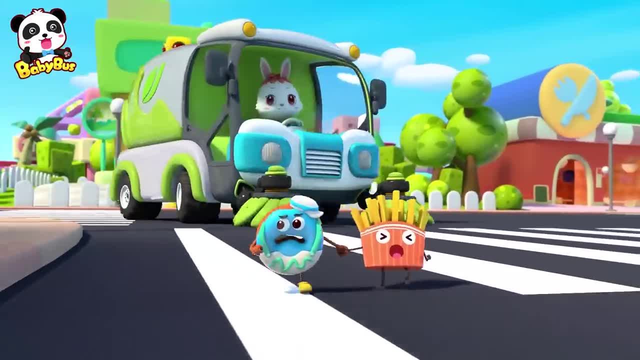 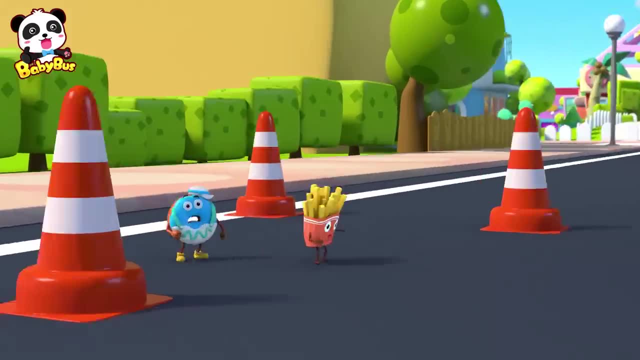 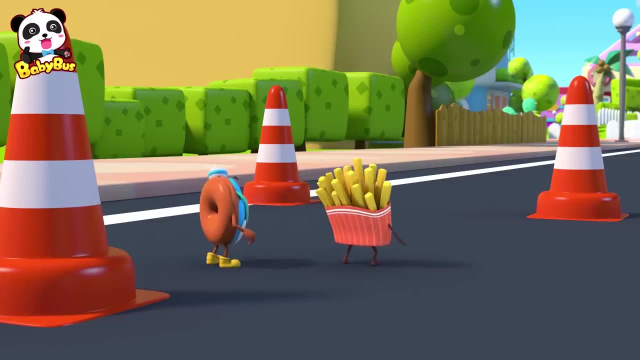 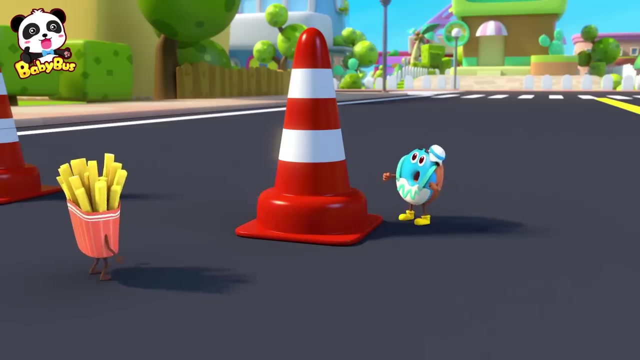 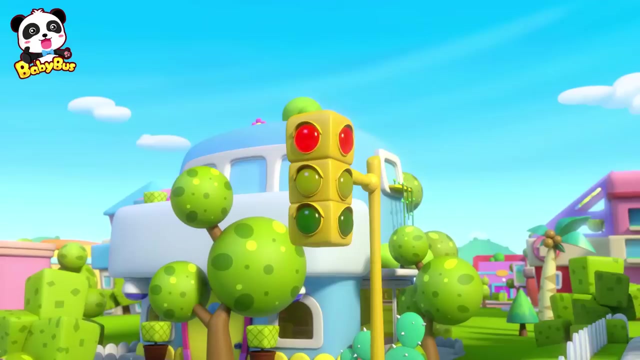 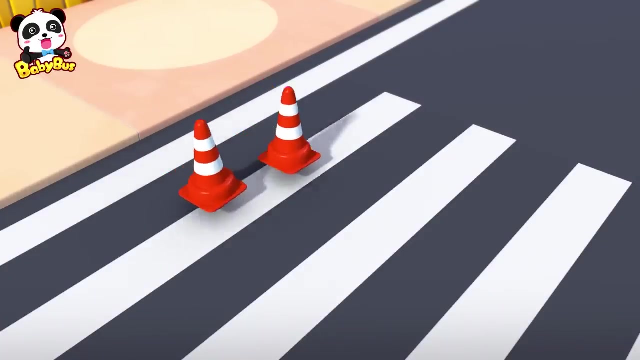 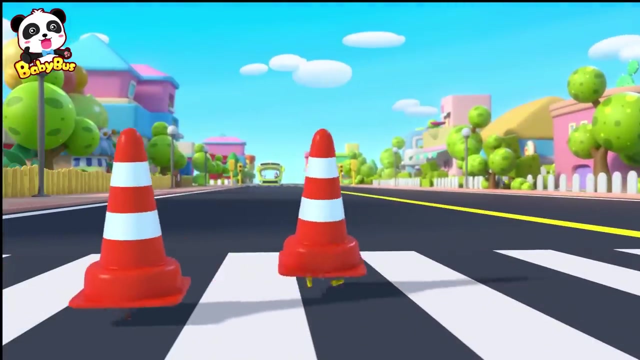 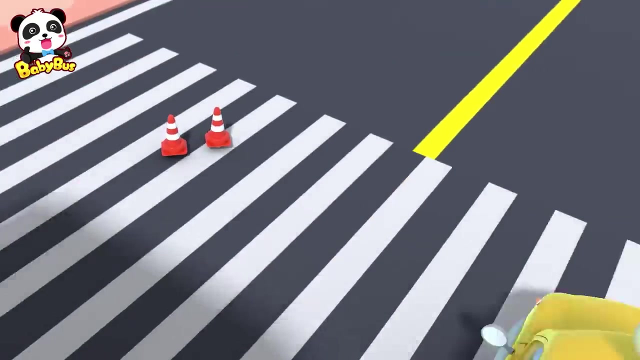 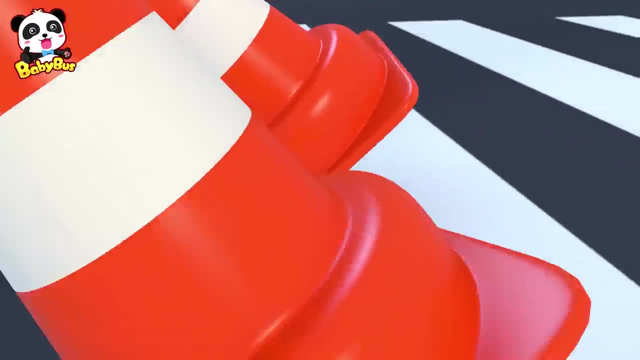 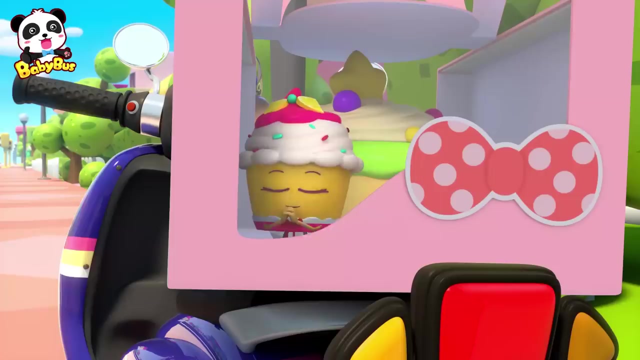 Ahhhh, Ahhhh, What's going on? Ah-ha, I got it. It's green, Let's go. A bus is coming, Get it, Get it, Get it. That was close, Let's go. Donnie Fry, please come save me. 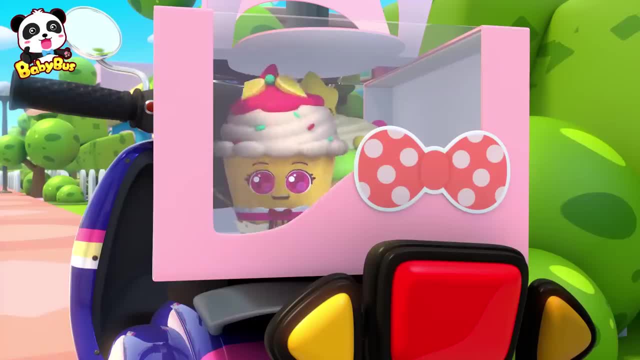 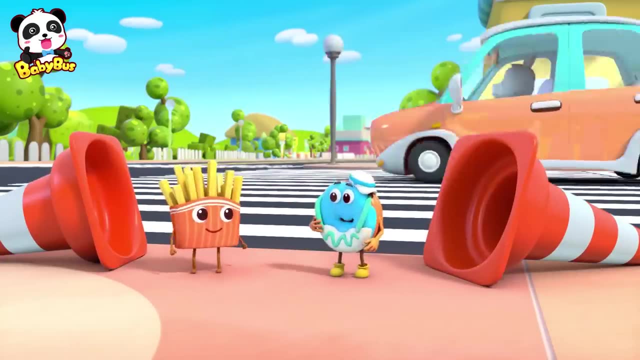 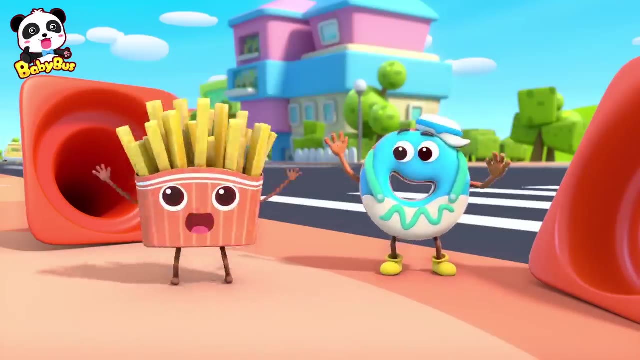 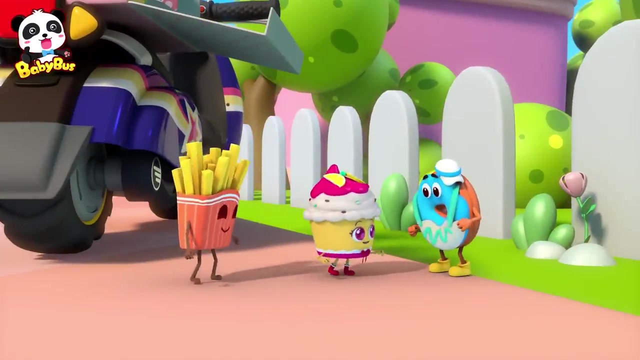 Donnie Fry, I'm here. I'm here. That was so scary. It's Katie, We're here to save you. Thank you, guys. I knew you would come and save me. Of course, We're good friends. 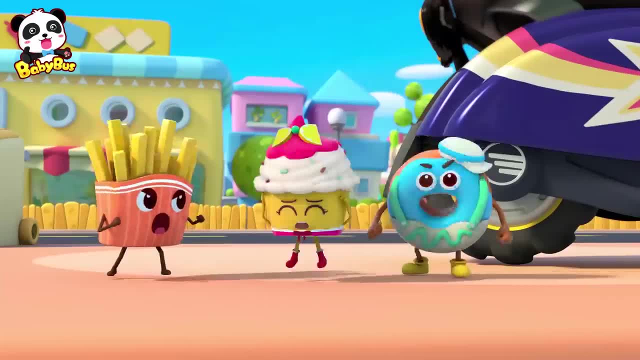 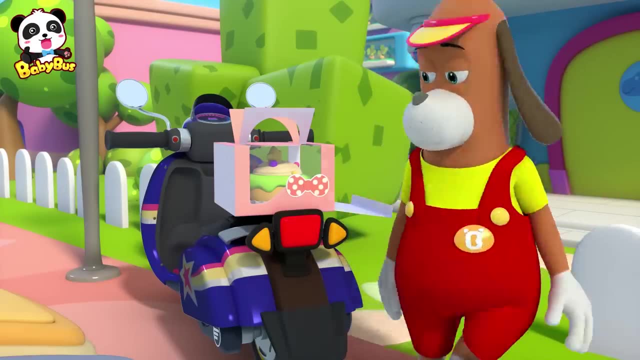 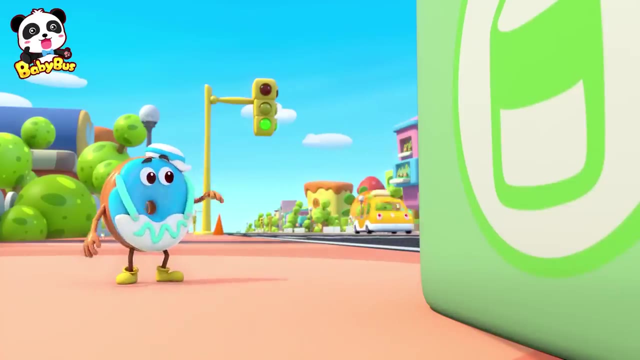 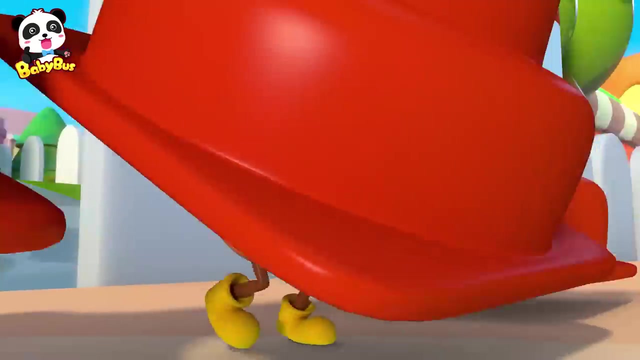 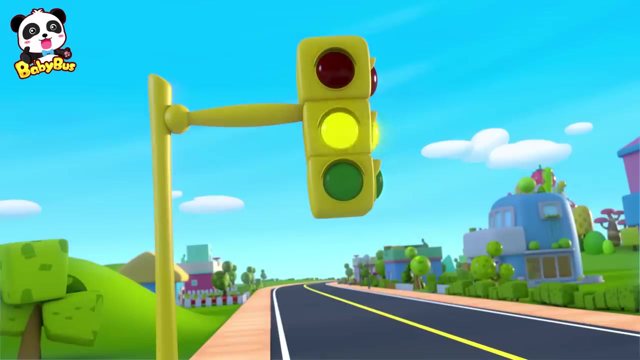 Ah, Quick hide, Quick hide. Ah, Hmm, Huh, Uh, Come out, guys, Let's go home. Okay, Okay, Yeah, Hihihaha, Hihihaha, Hihihaha, Hihihaha, Hihihaha. 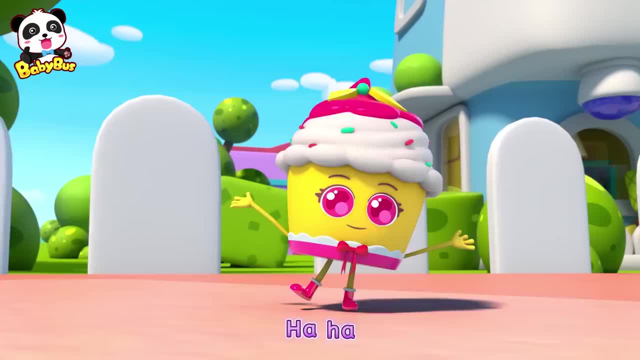 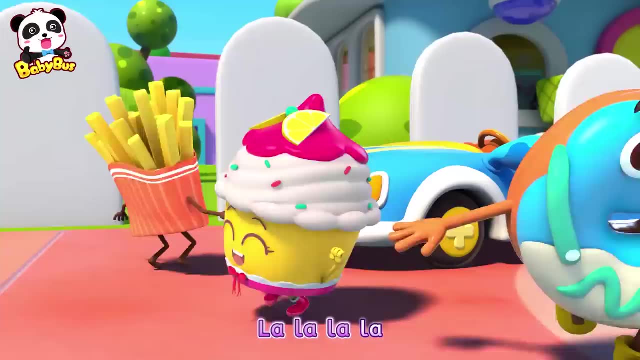 You're smart and brave, my good friend Hee-hee-ha-ha, hee-hee-ha-ha, You're smart and brave, my good friends La-la-la, la-la-la, la-la-la-la-la-la. 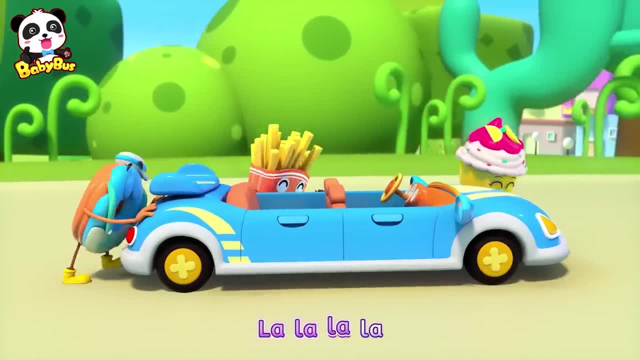 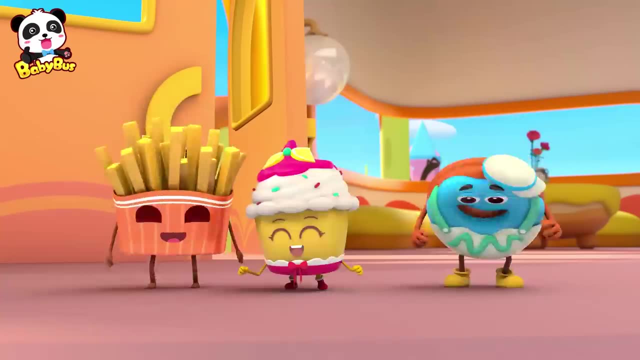 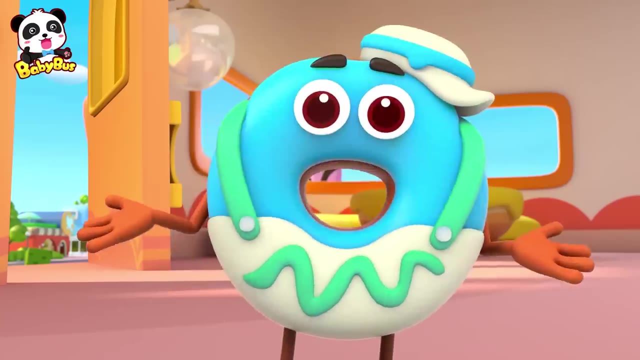 You're so great, La-la-la, la-la-la, la-la-la-la-la-la, Wow, we're home. Yay, Yay. If your friends are in danger, be brave and think of a way to help them, But always remember to be careful. 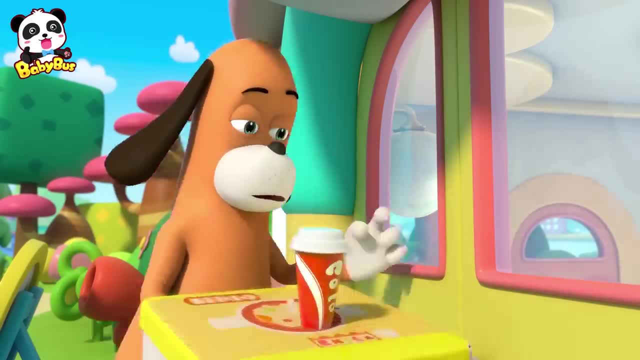 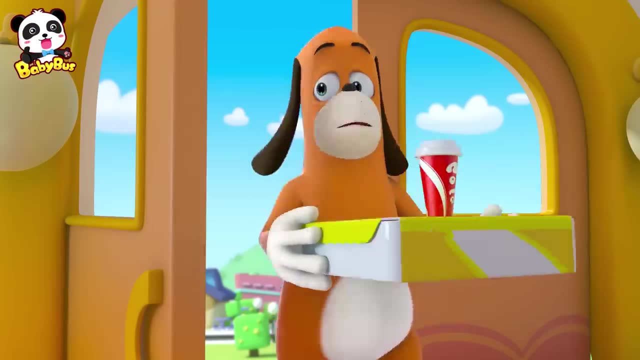 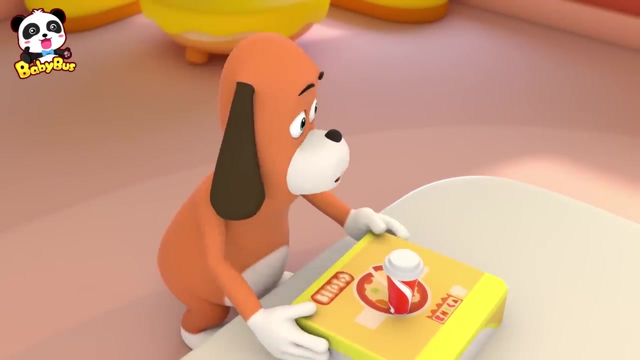 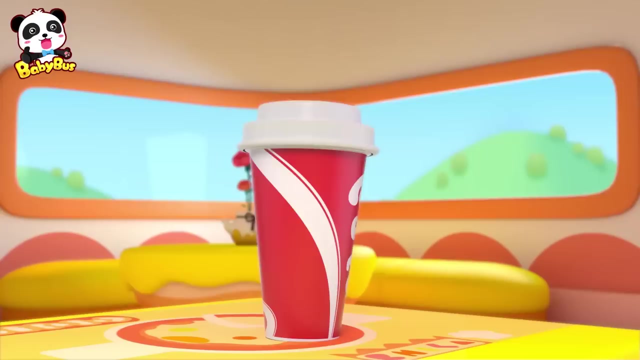 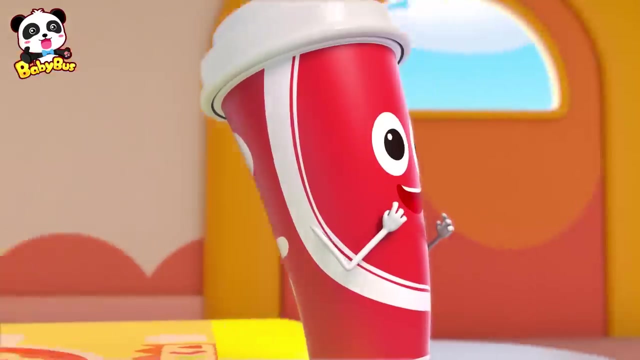 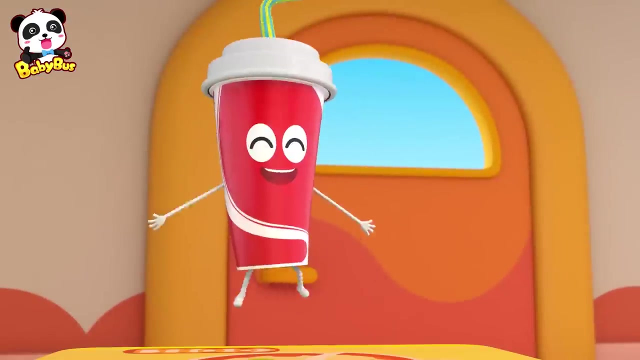 Your food is here, Kiki Mew-mew. Hmm, where did they go? Hmm, I'll just put it on the table. Hmm, Hmm, Ha, Oh, yeah, Whoa, Huh, New friend, Ah. 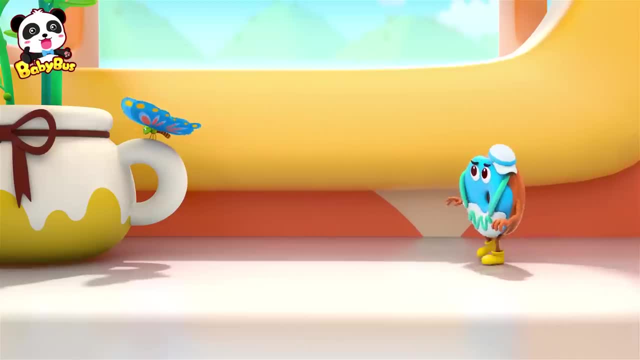 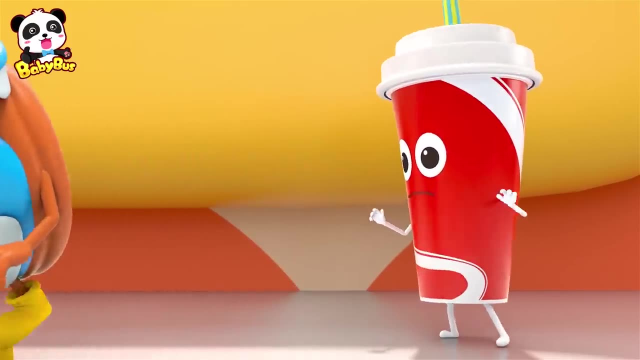 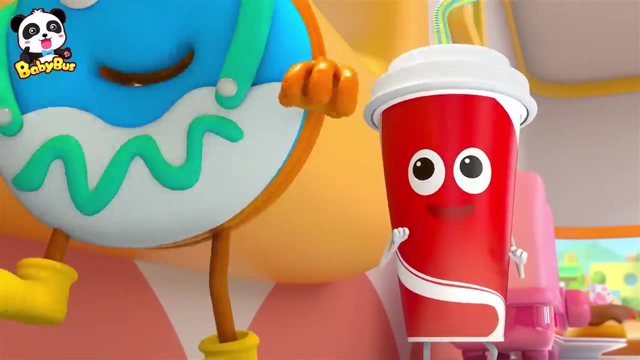 Hee-hee-hee-hee-hee-hee-hee-hee-hee. Hi Ah, Shh, Shh, Ah, Hee-hee-hee-hee-hee-hee-hee-hee Huh. 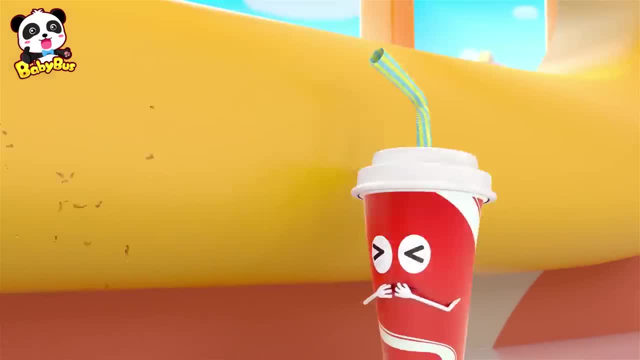 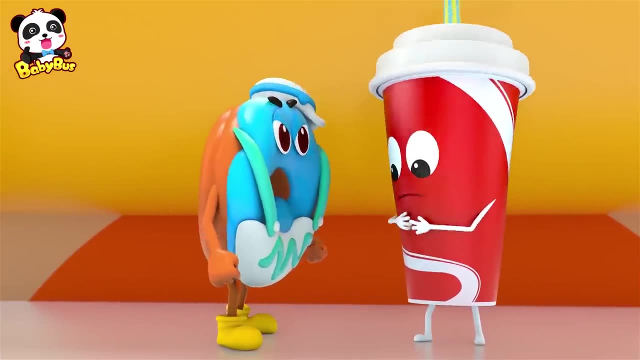 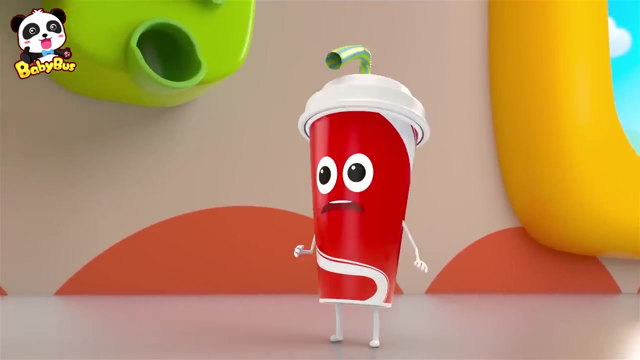 Mew-mew-mew-mew-mew. Ah Huh, You scared away my butterfly. Hmm, Mew, Sorry, Sorry, Huh, Huh, What's that sound? Huh, A beautiful castle, La-la-la-la. 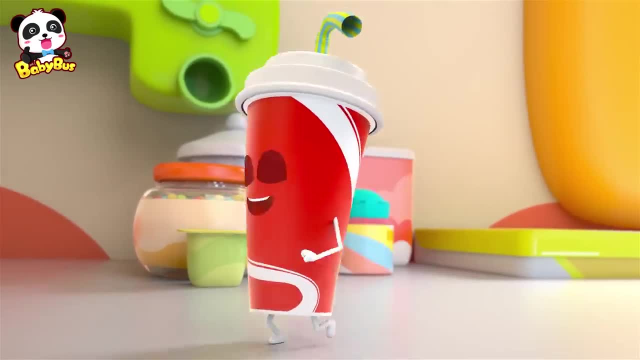 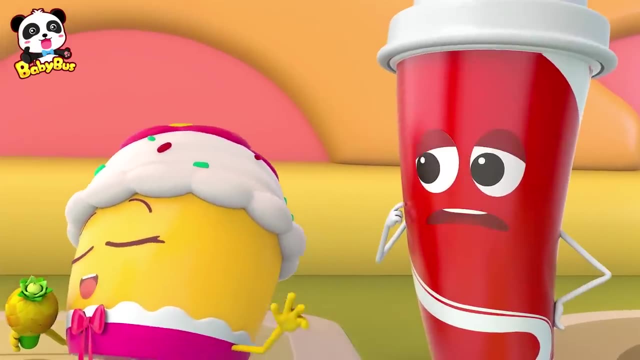 You and me together. Such a nice voice, Hee-hee-hee-hee-hee, Hi, La-la-la-la-la-la, Let's build a castle, Let's be friends, A beautiful castle, La-la-la-la-la. 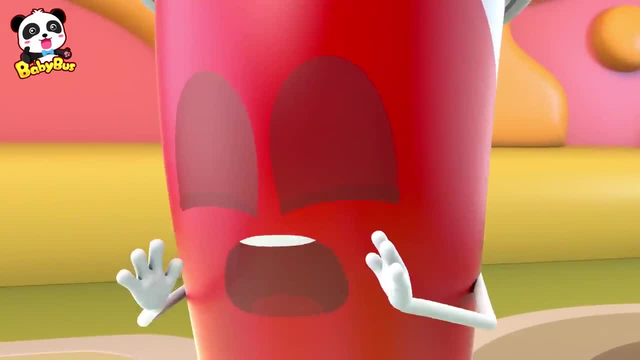 Hi, I'm Kola, You and me together. La-la-la-la-la-la, Ha, La-la-la-la-la-la, Oh hi, You're a really good singer. Can you teach me how to sing? Of course, Listen carefully. 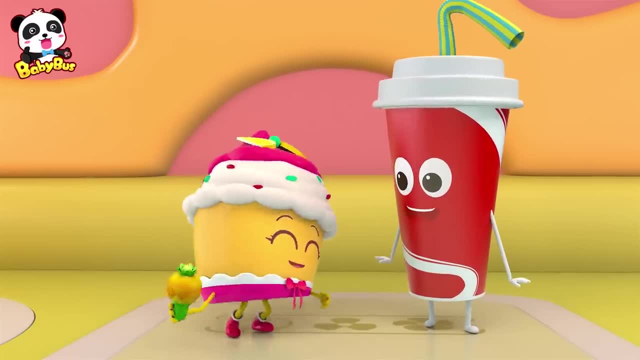 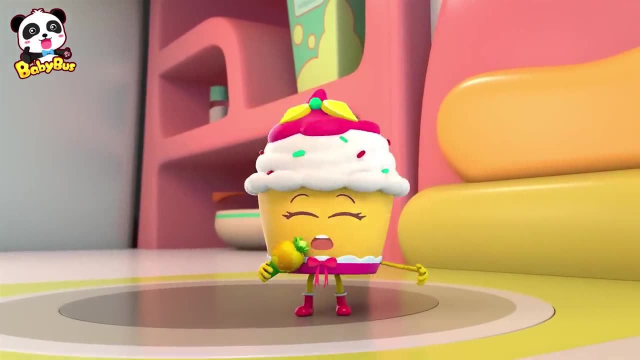 La-la-la-la-la-la, Let's build a castle La-la-la-la-la-la. Great, Now it's your turn. Okay, Watch me. Hee-hee-hee, Oh, Oh, Oh, Oh, Oh, Oh. 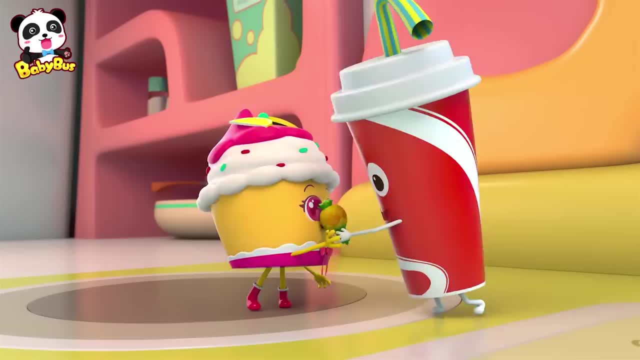 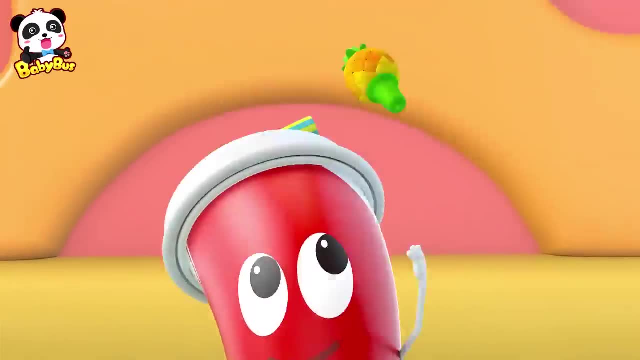 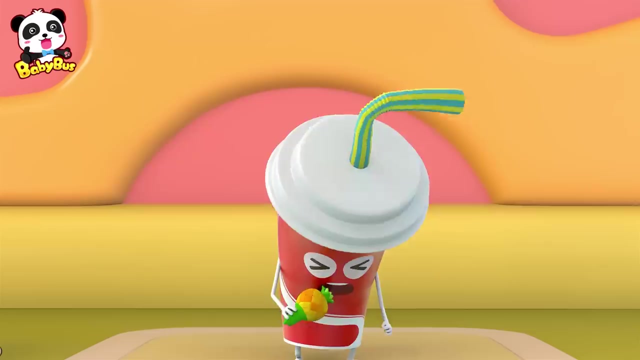 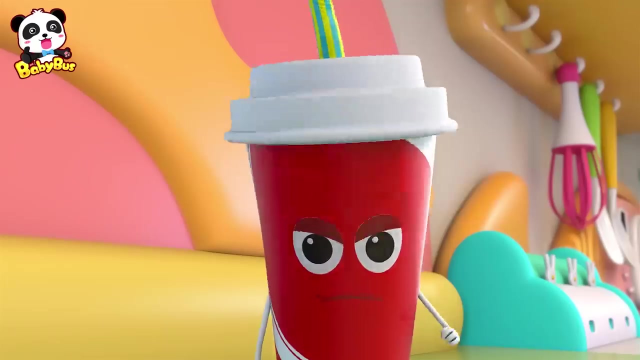 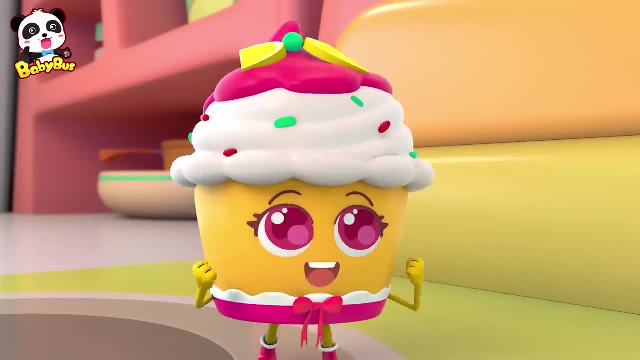 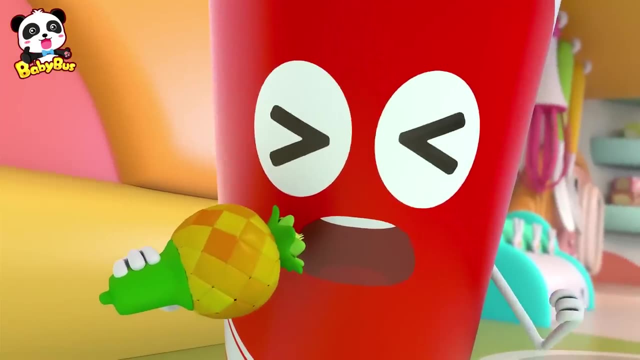 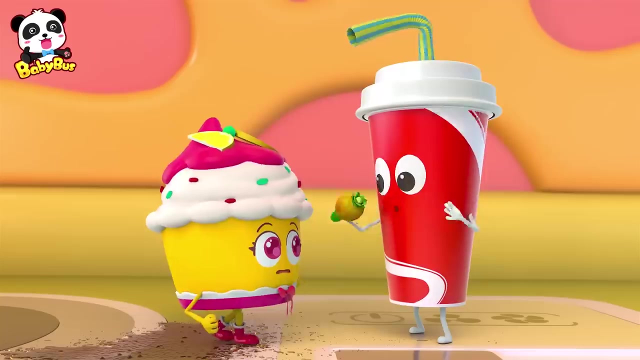 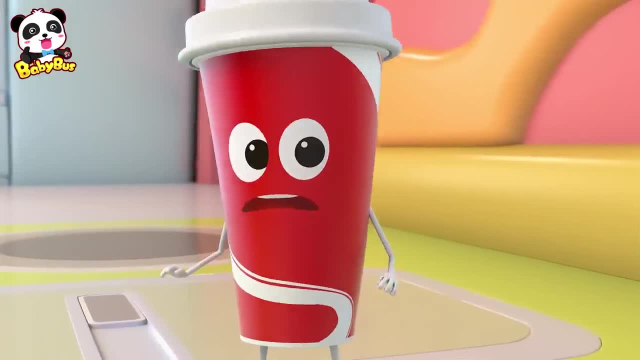 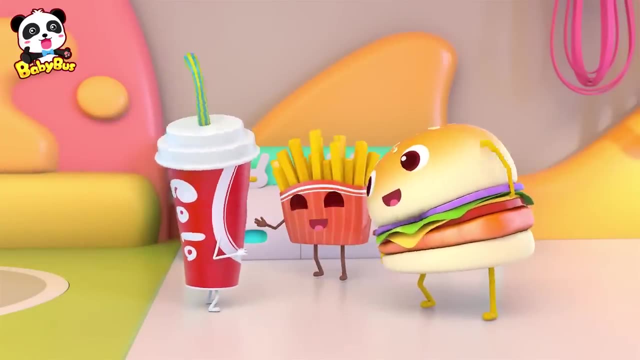 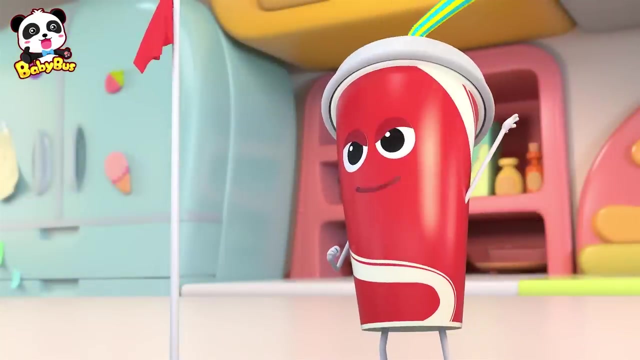 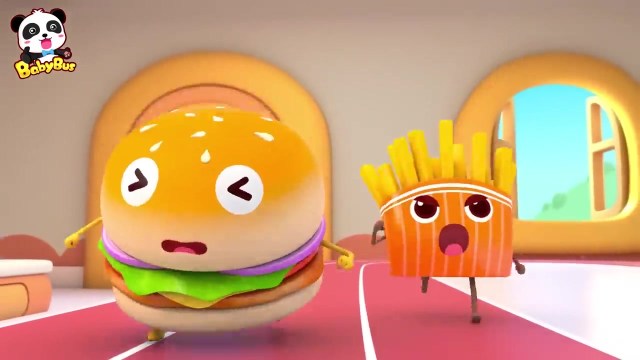 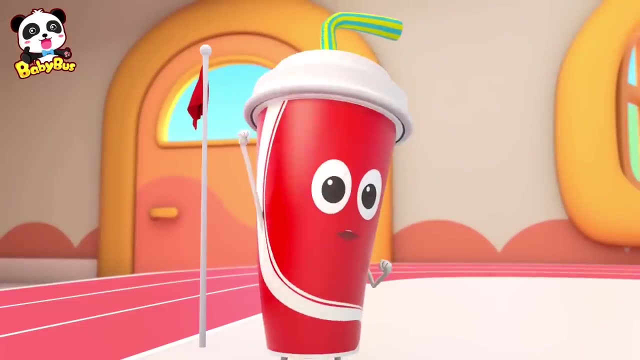 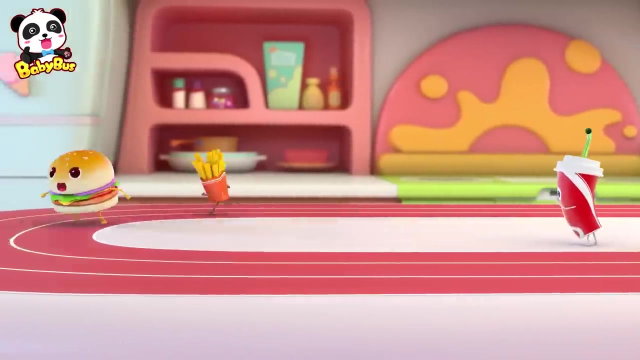 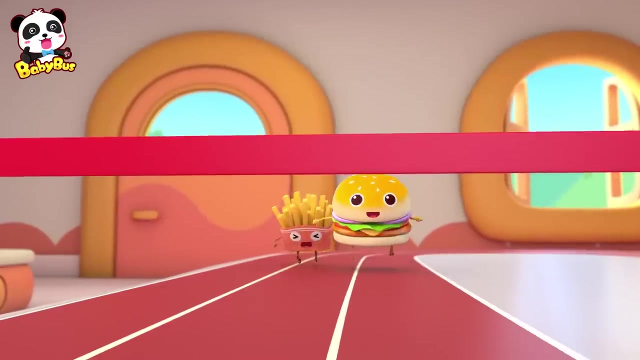 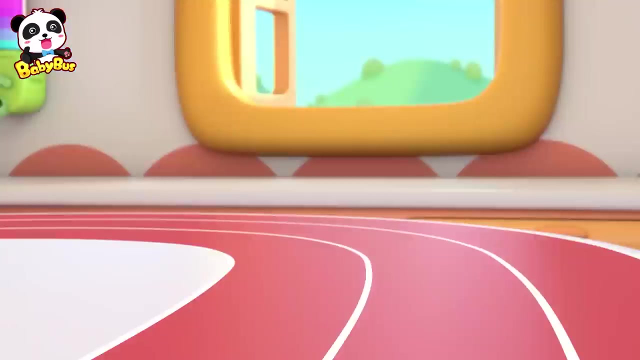 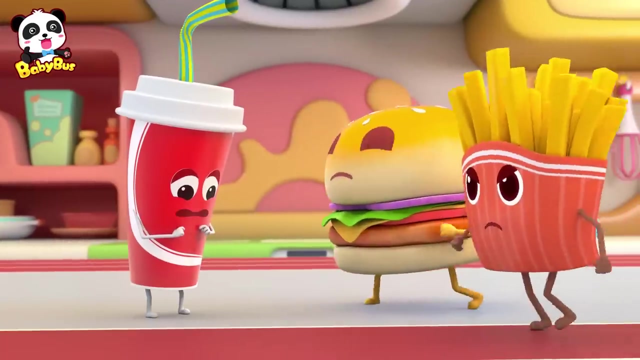 Will you help us? Okay, We will have a running race. Can you be the referee? Okay, That's it. Go, Come on run, Come on run, Come on run. Hey, Sorry, I didn't mean it. 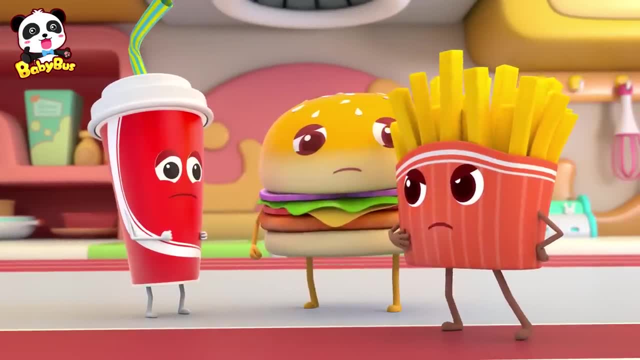 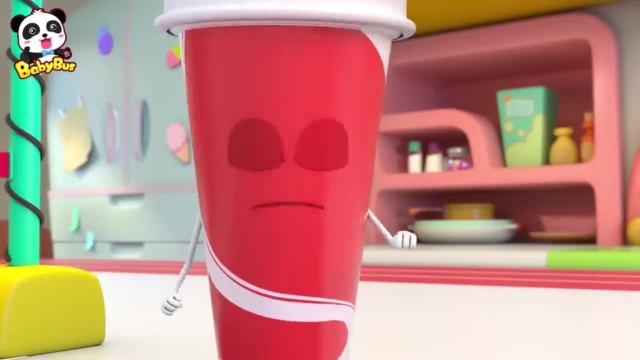 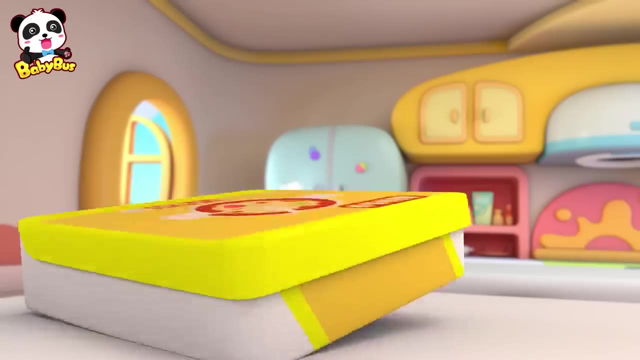 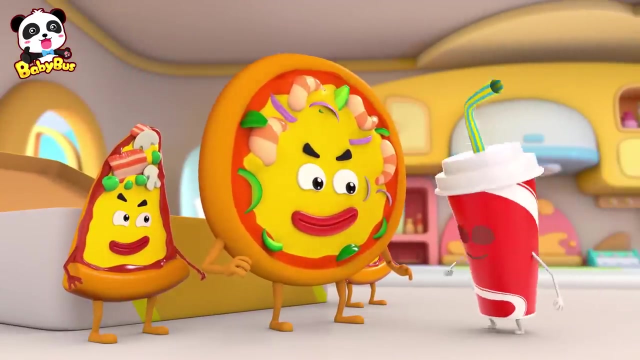 You ruined our race. It's all your fault. Sorry, I burp when I get nervous. Let's go, Wait What You'd better run. You don't know me. I love you. Hey you, Hey, You got me. 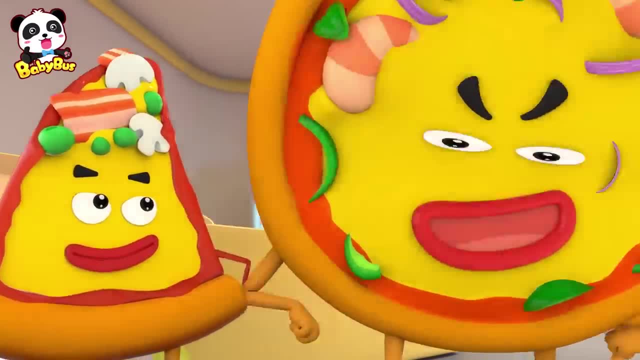 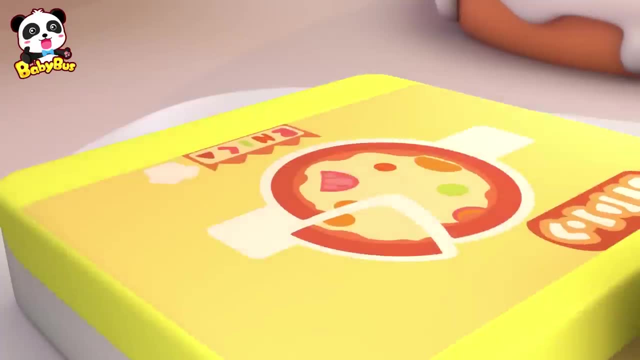 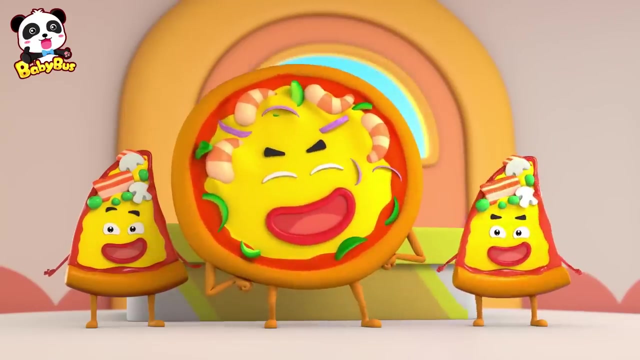 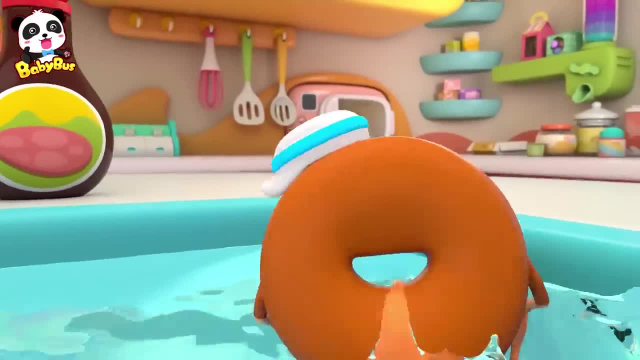 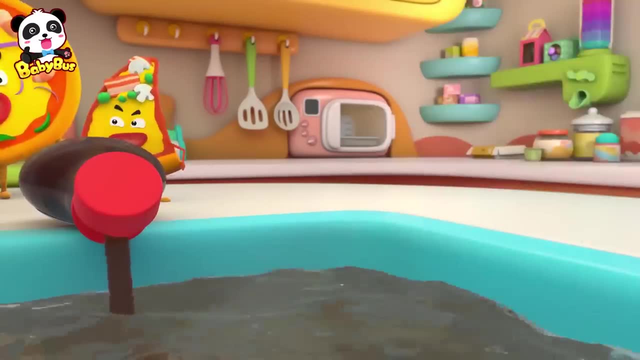 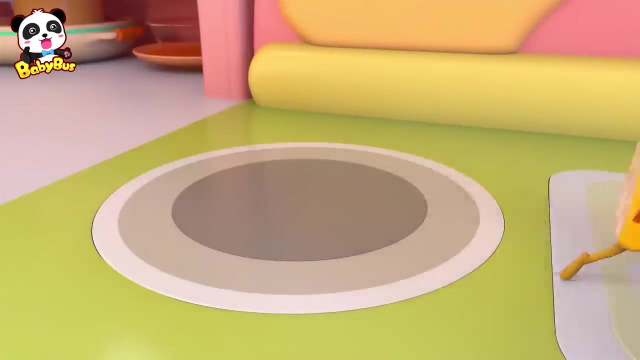 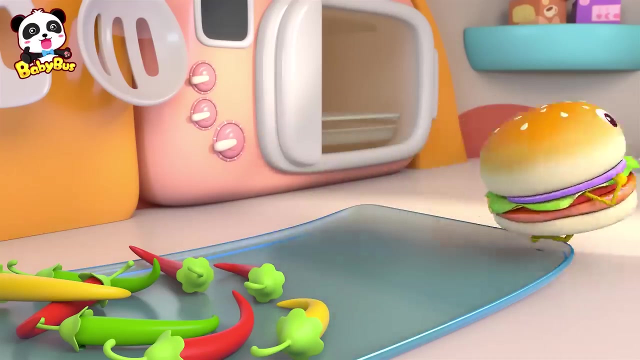 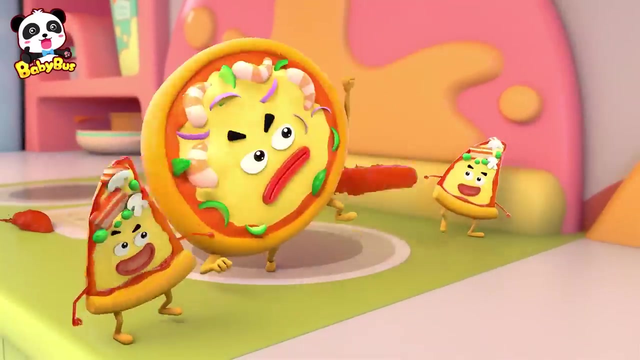 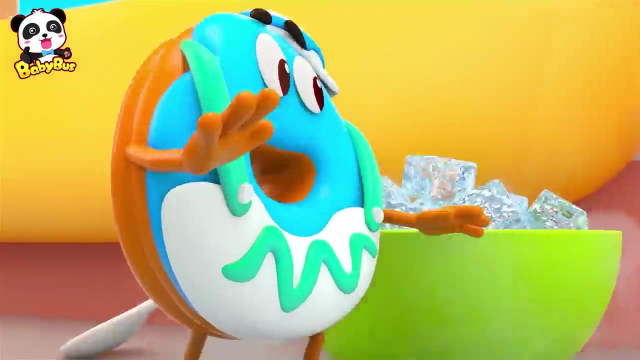 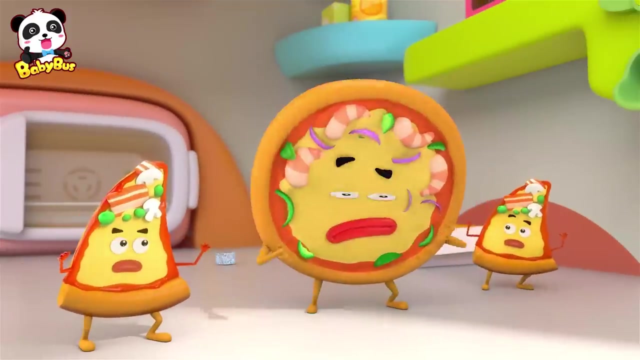 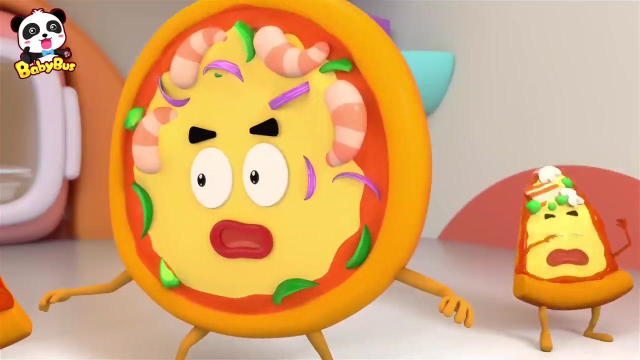 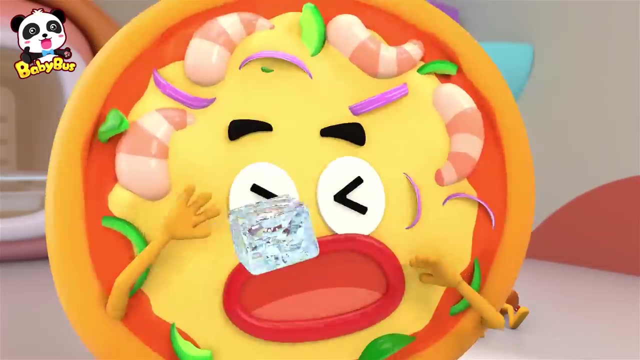 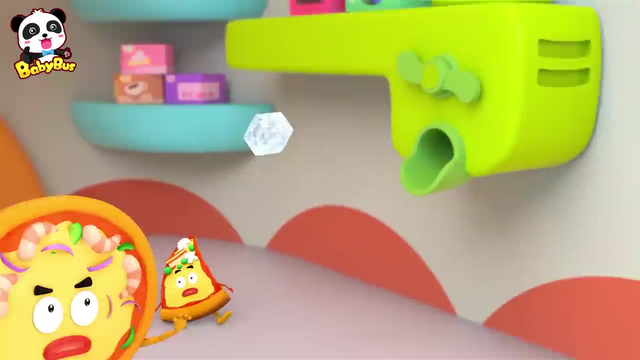 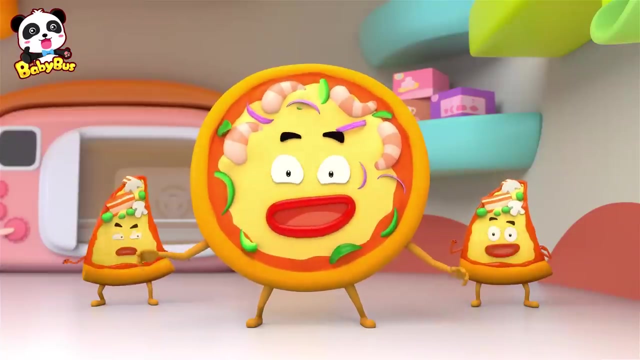 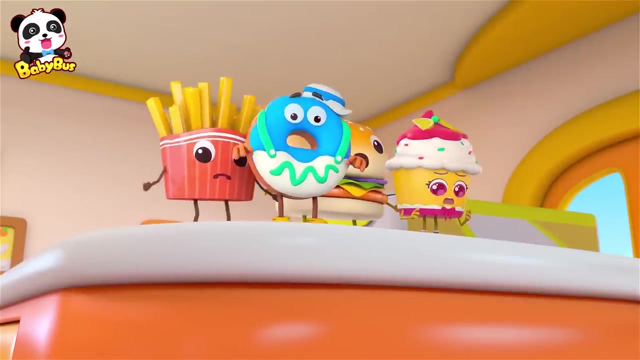 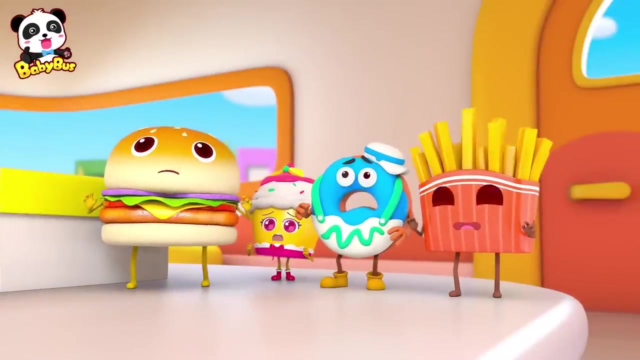 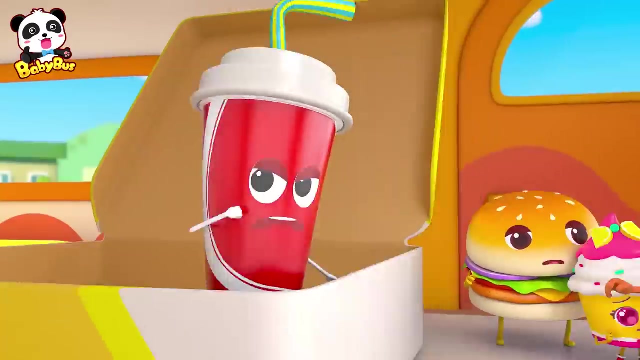 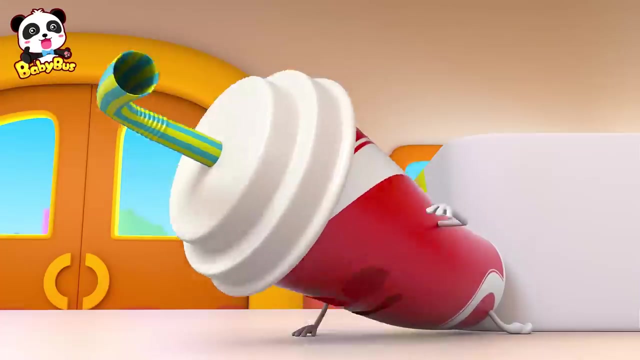 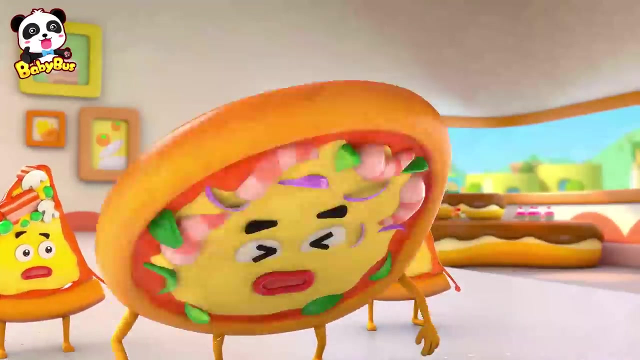 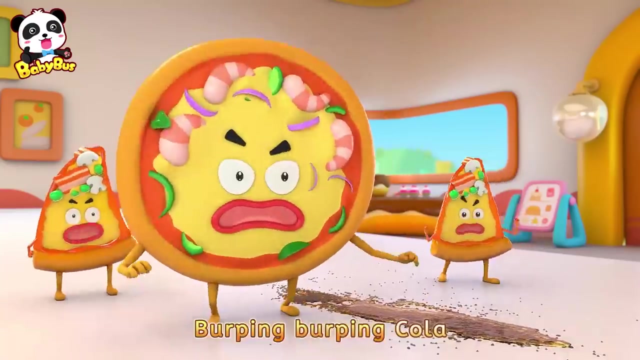 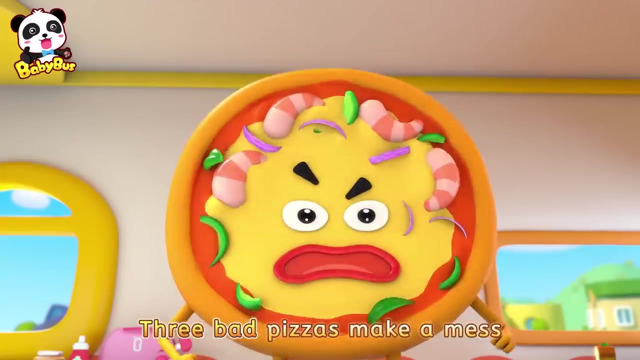 La, la, la, La la la. I have an idea. Ice Cube Bob, You can't get away. Stop You again. Stop, Don't come any closer. Three bad pizzas make a mess. Brave Cola says: what should I do? 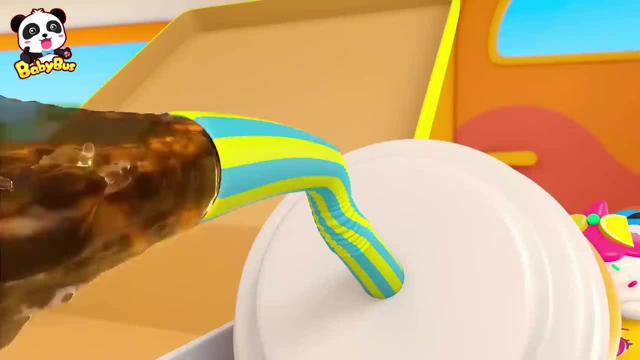 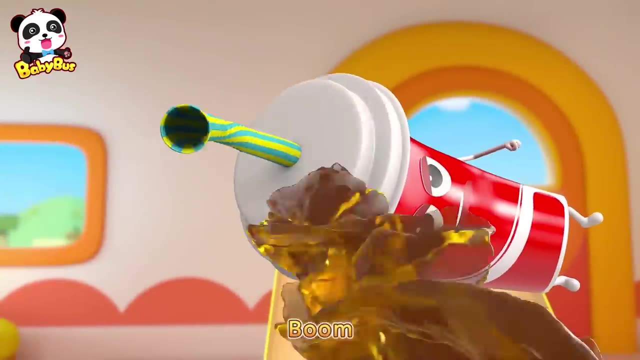 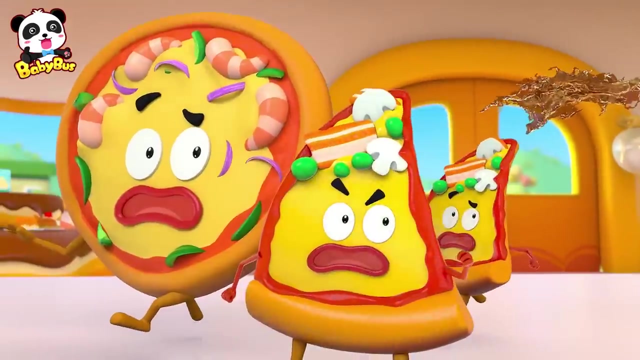 Let's see what we found out. Cola Bomb, Come on, come on, Brave Cola, Cola Bomb, Cola Bomb. Here we go, here we go, Brave Cola Burping, burping Cola, Burping, burping Cola. 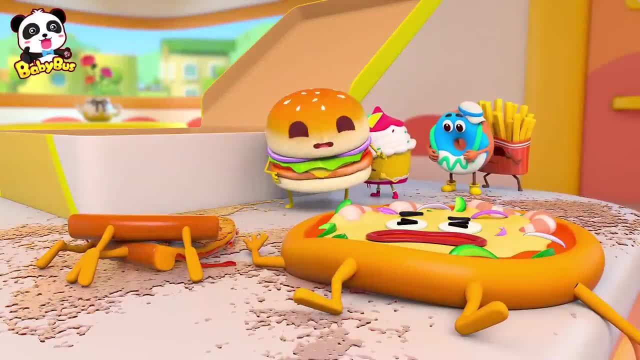 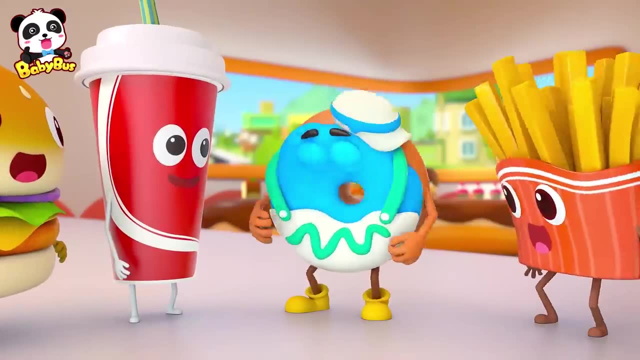 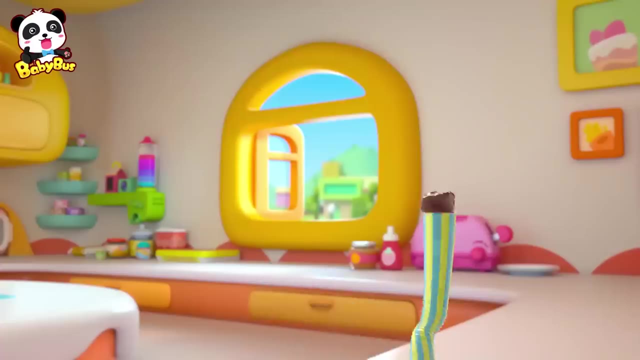 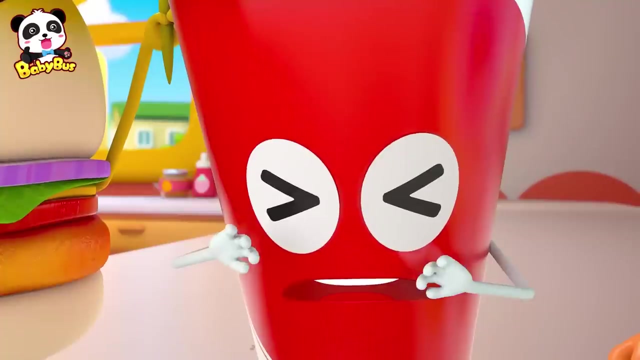 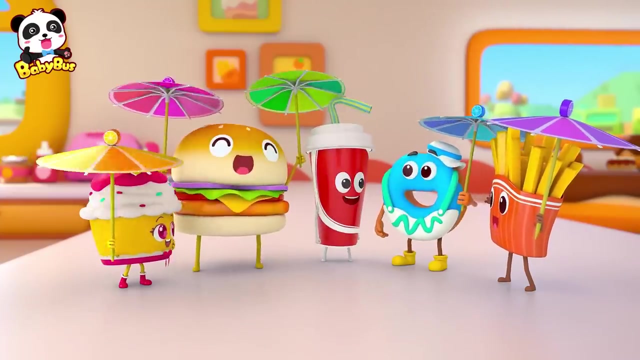 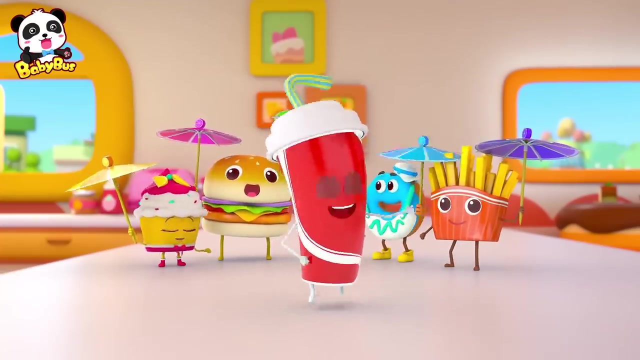